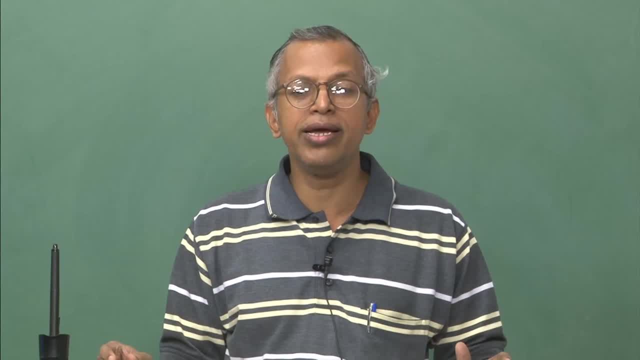 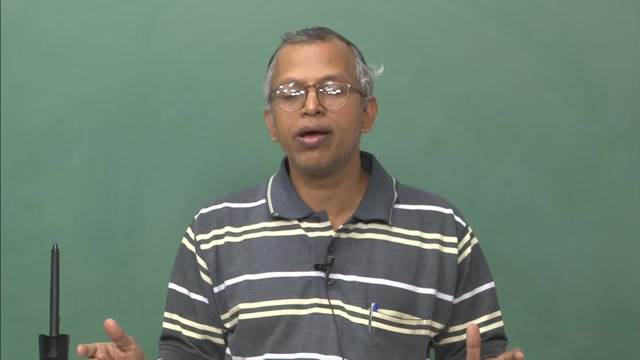 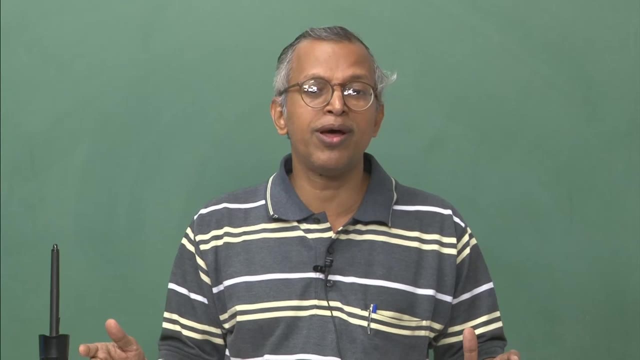 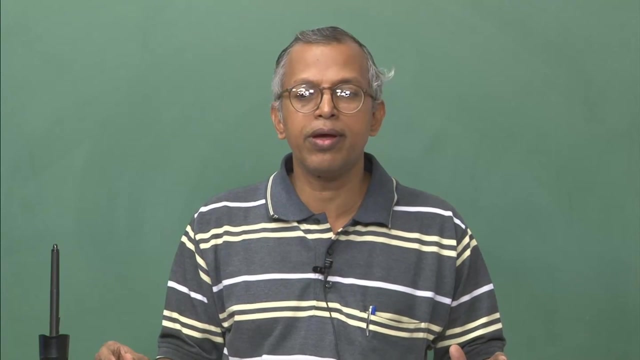 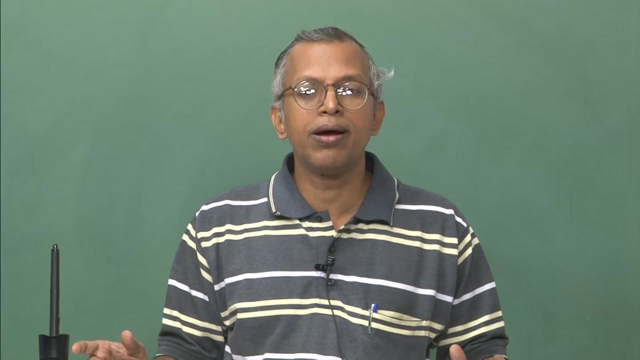 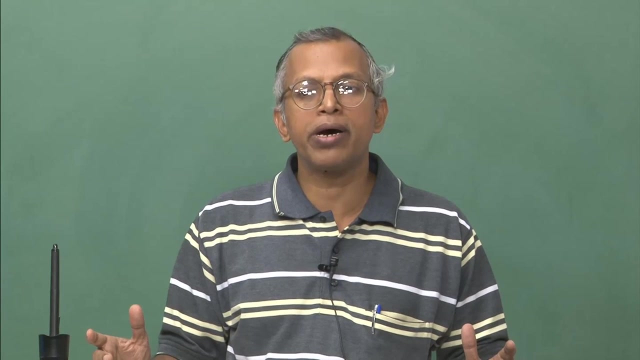 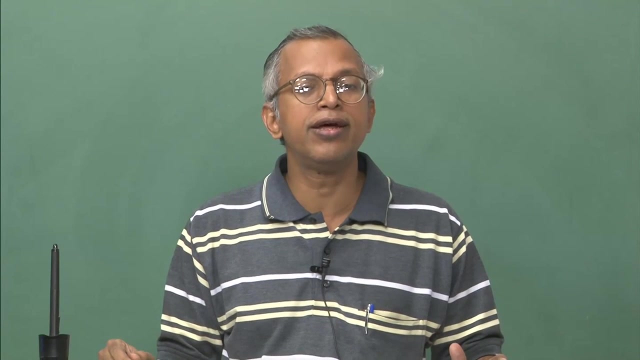 flow And I had already initiated discussion in the last lecture on the compressible flow and, if you recall, I ask a question: whether a fluid will be compressible or a flow will be compressible. So we talked about the compressibility factor and we also talked about there are other definition. 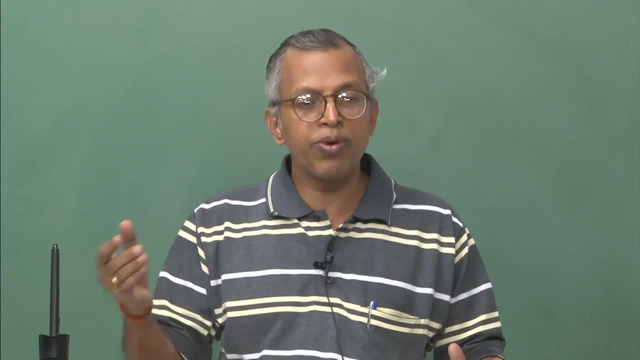 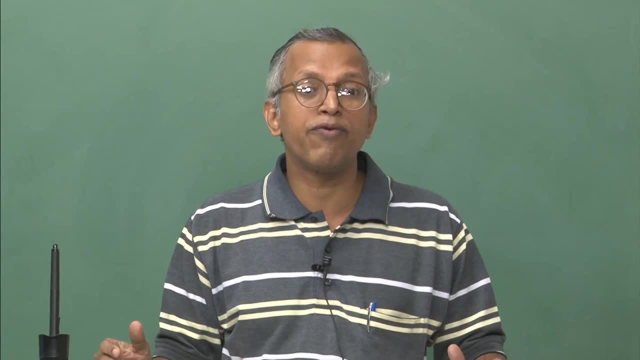 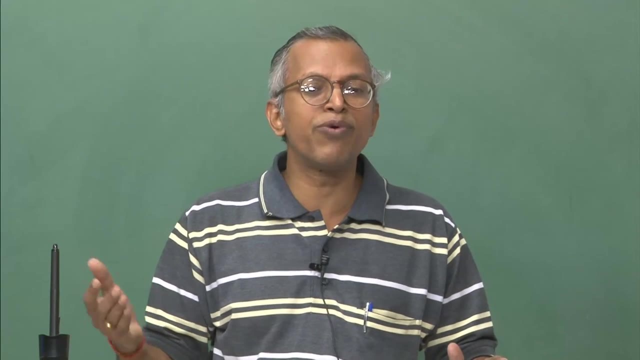 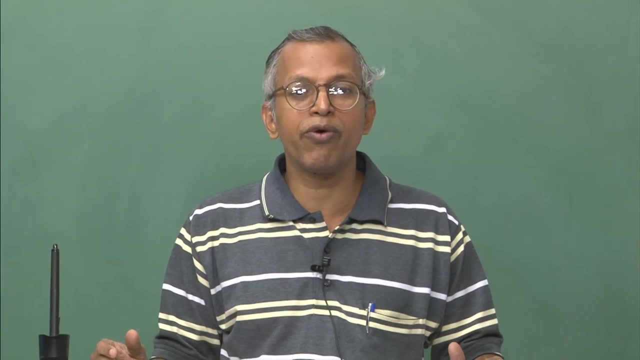 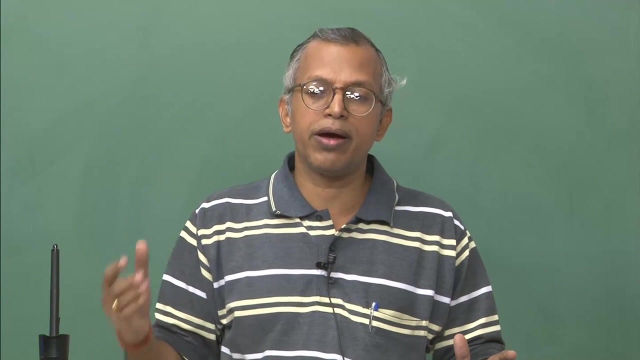 as well, because this is a more general. but to be more specific, one has to talk about the compressibility factor for isothermal flow condition or for an isentropic flow, And considering the flow to be isentropic. So we use those definition to derive equation. for what? for speed of sound. and I also try. 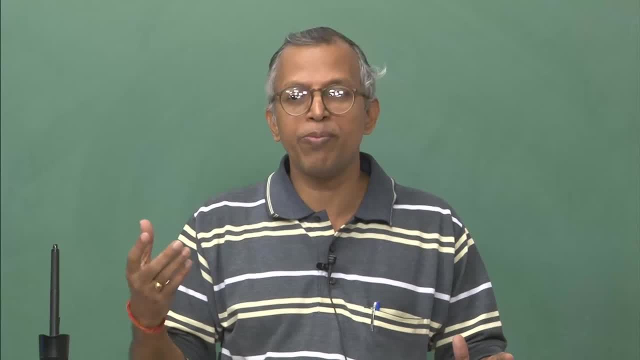 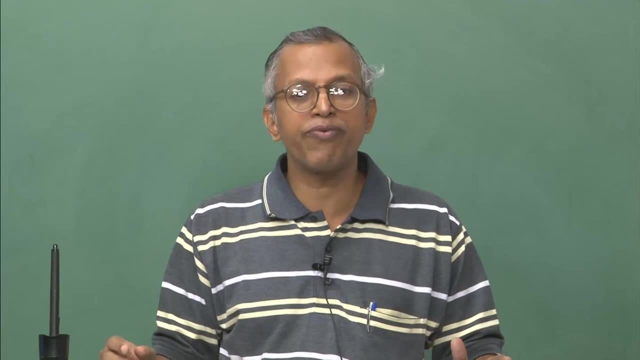 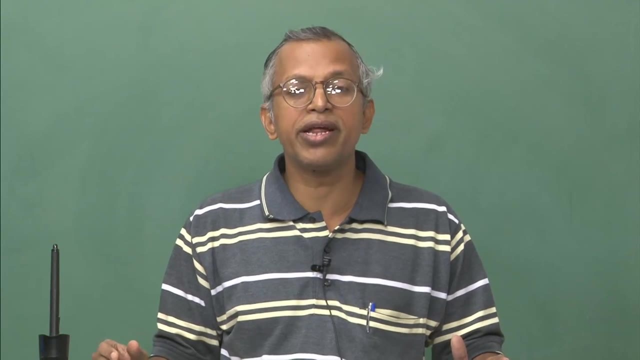 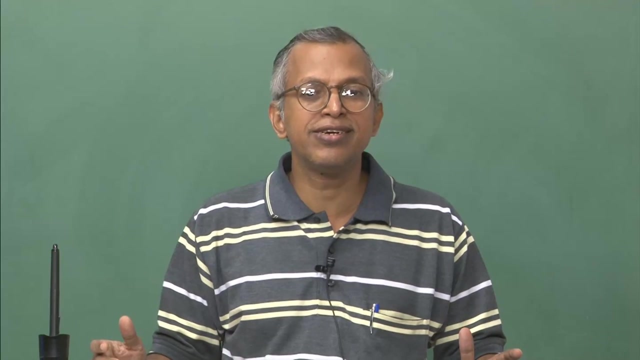 to give an idea about what is the sound, how it behaves? what are the mechanism of the sound propagation going to, the microscopic effects or the molecular level, As I told you yesterday that by using the kinetic theory of gases, theory of gases, one can derive an expression for average molecular velocity which is equal 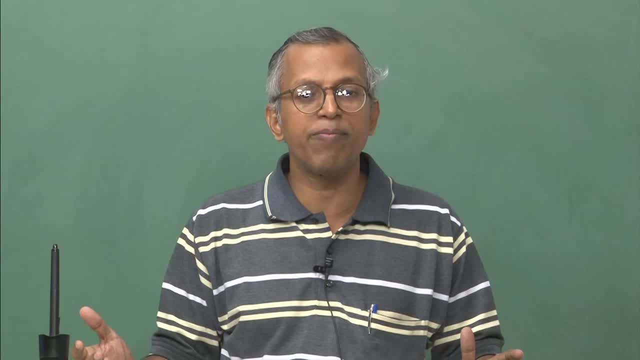 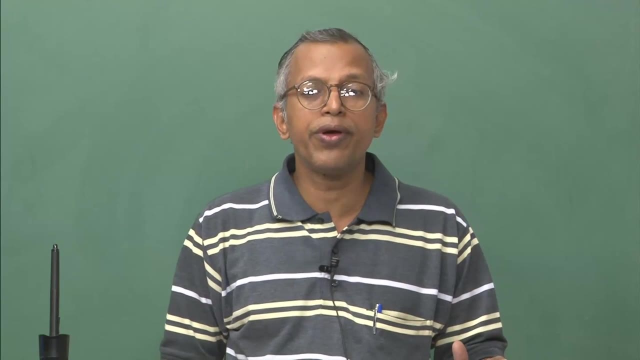 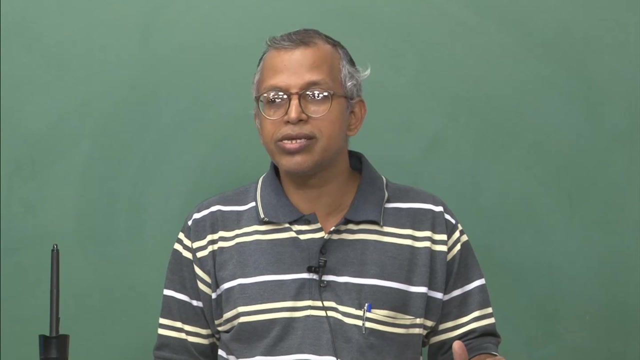 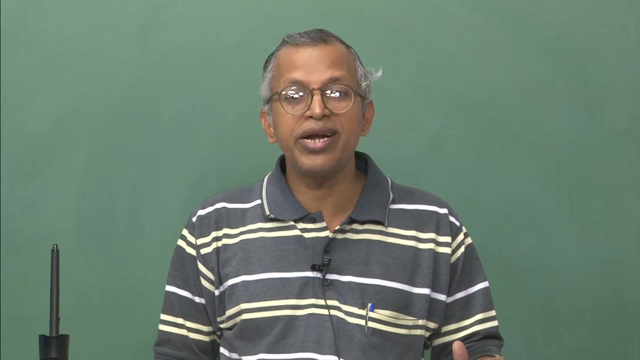 to root over 8 pi t divided by- sorry, root over 8 pi r t divided by k or some constant and which can be related to the speed of sound. And if you look at the speed of sound we have derived for an ideal gas, right, that is a is equal to root over gamma r t. If you look. 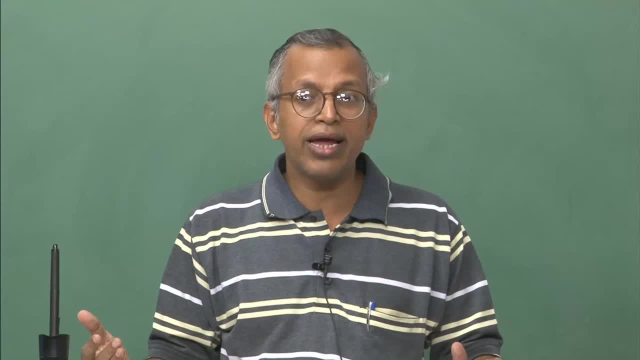 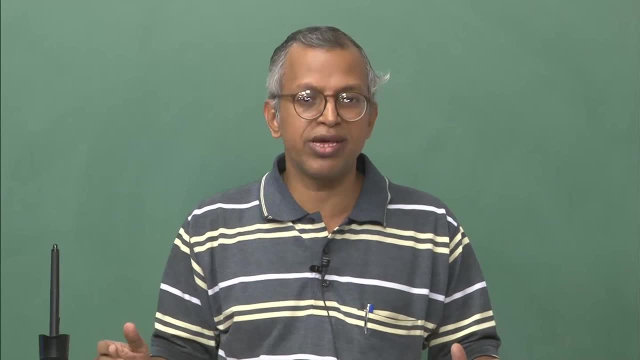 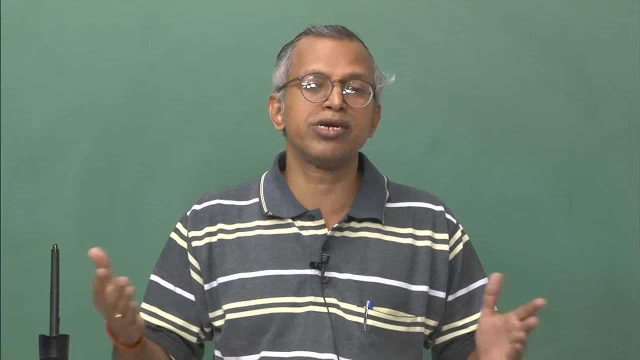 at this root over gamma r t. that means it is a function of the temperature and also the fluid properties. You remember I had taken, you know, example of air and helium. I said so that at same temperature it is having different speed of sound, and keep in mind that r what 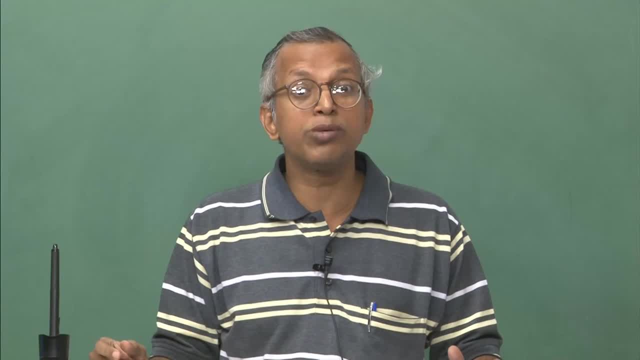 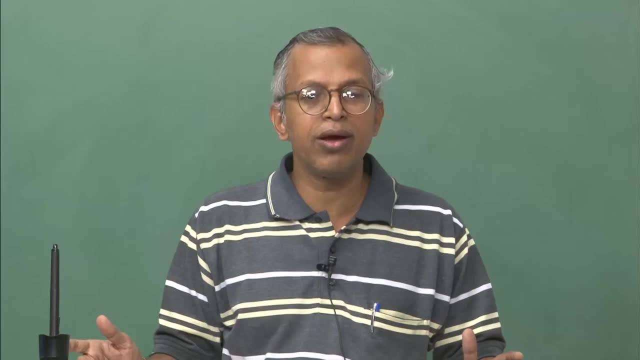 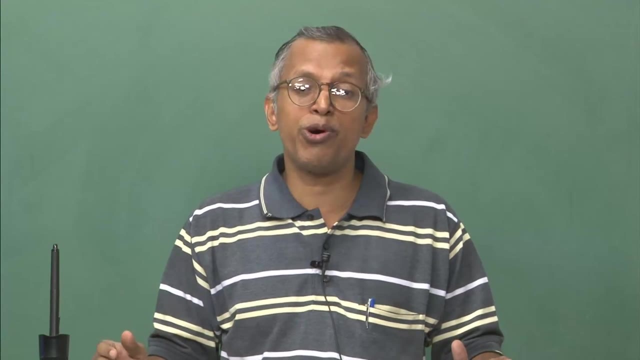 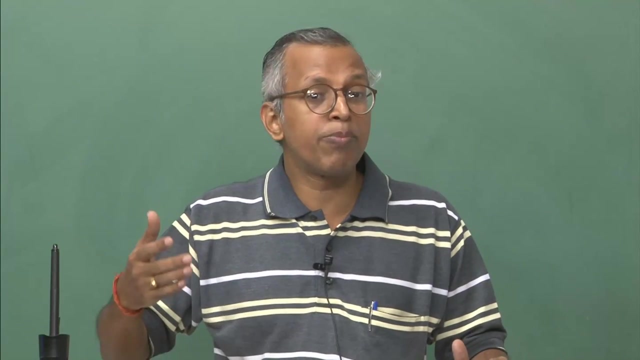 I am using that equation or expression is basically specific gas constant, which is ratio of universal gas constant, and molecular weight. When I talk about molecular weight, then molecular weight of particular gas and this speed of sound will be different in different material, for example. For example, water right, will it be different or it will be same. it will be actually different. 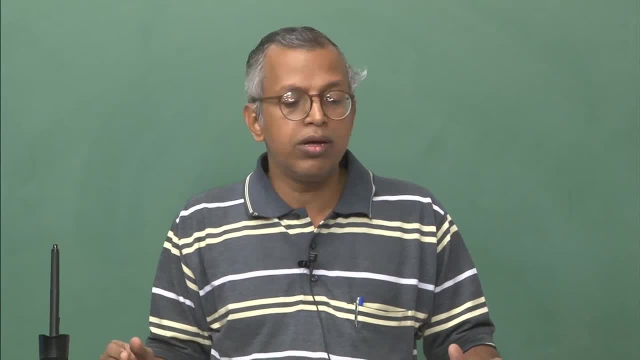 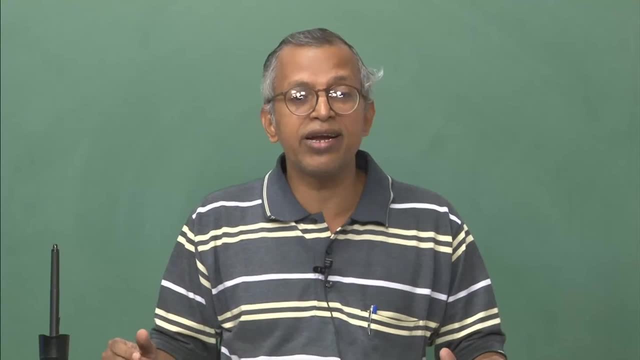 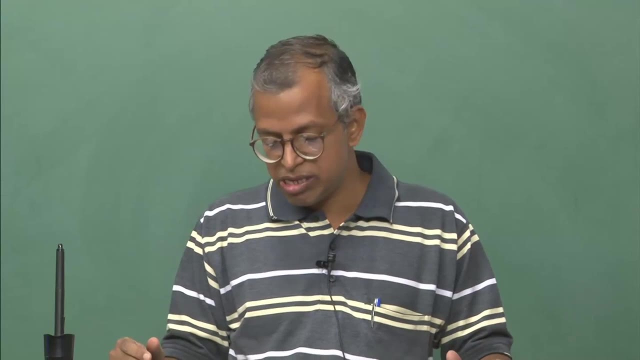 because it depends on the properties of the fluid. And based on this speed of sound, which is very essential to delineate whether the flow is compressible or incompressible, we define a term known as Mach number, which is a ratio of velocity and speed of sound. 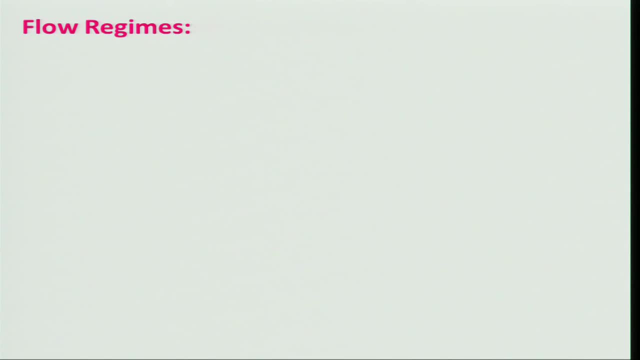 And based on this Mach number, we can divide the flow into various regimes. and what are those regimes? one is, of course, you can call it as a subsonic flow when Mach number is less than equal to 1. because Mach number equal to 1, we call it as a, basically what you call. 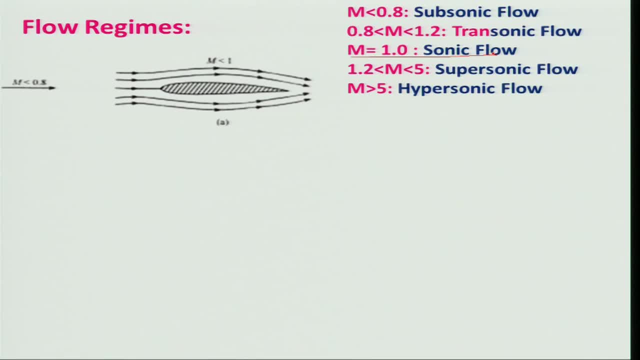 we call it as a sonic flow, Right, Right. So when it is less than 1, we are supposed to say it is a subsonic flow. when it is greater than 1, we should say it is supersonic flow. as usual, right, one is subsonic, other is sonic. 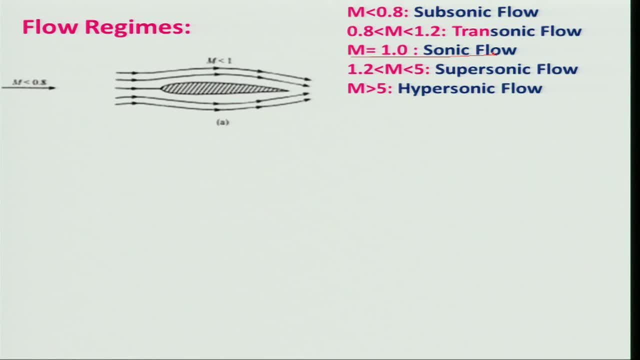 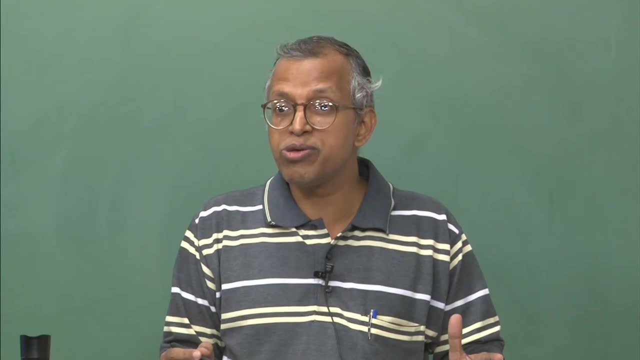 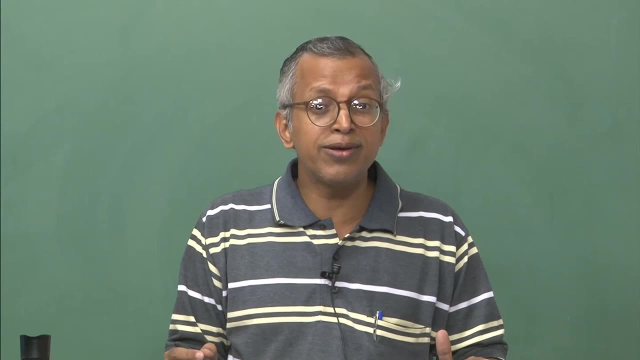 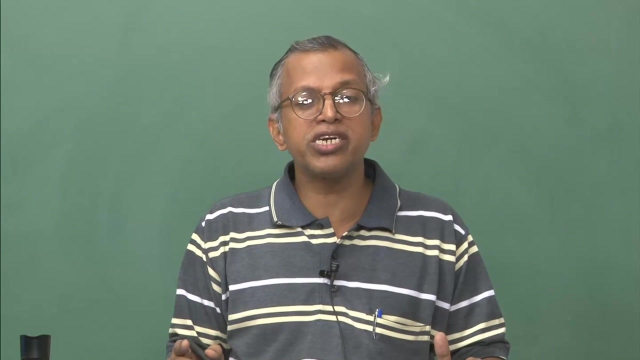 other is supersonic. However, people like a person. you are the bunker man. right, you know him. he is a great fluid dynamist. right, you are aware about bunker man street. Yes, Where this vortex streets will be shaded downstream of the flow over a cylinder or a any body. 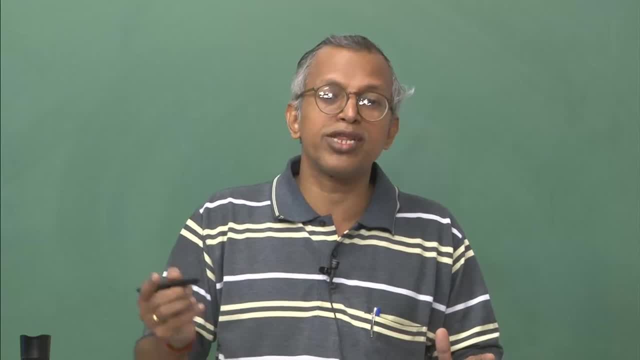 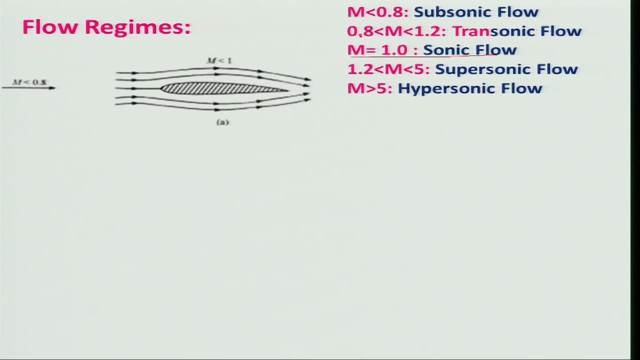 right So you might aware. if you are not aware, just look at he is a. he gave the you know idea of transonic flow, that is, the flow when it is between 0.8 to 1.2. you know, in this regime it is we it call as a transonic flow. Question is, what really happens it you? 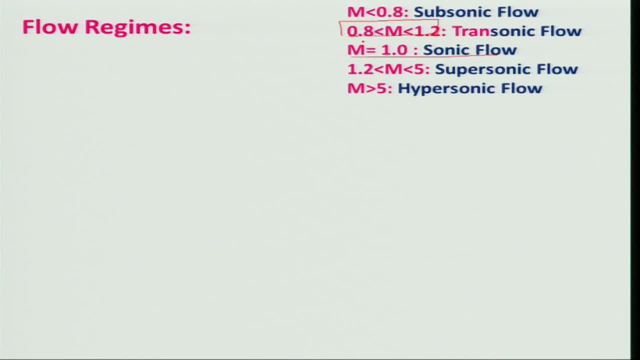 know in this subsonic flow and what happens in transonic flow, which we are going to see, and beside this, like when the flow is between the Mach number of 1.2 and 5 or less than 5, we call it as a supersonic flow. 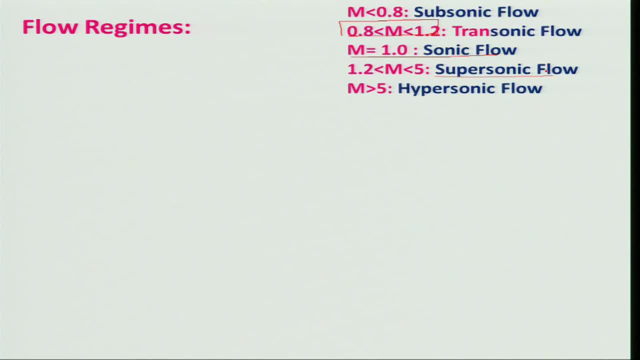 Right Right. When Mach number greater than 5, we call it as a hypersonic flow. Now, what is the difference between the supersonic and hypersonic? similarly, transonic and supersonic and subsonic and transonic? this we need to look at because it will be helpful for us to appreciate the 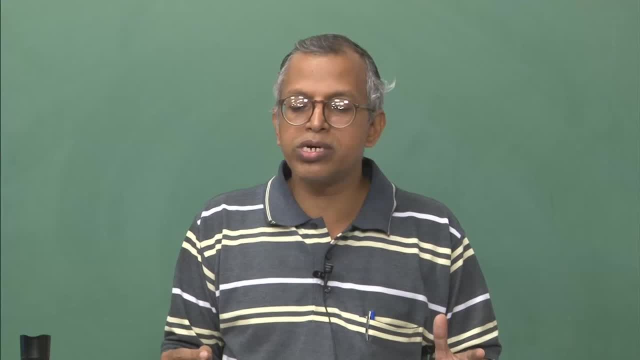 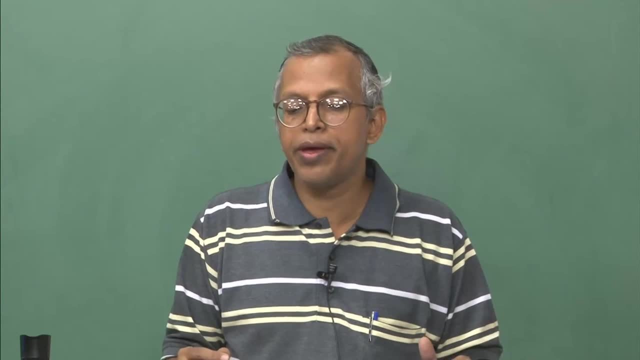 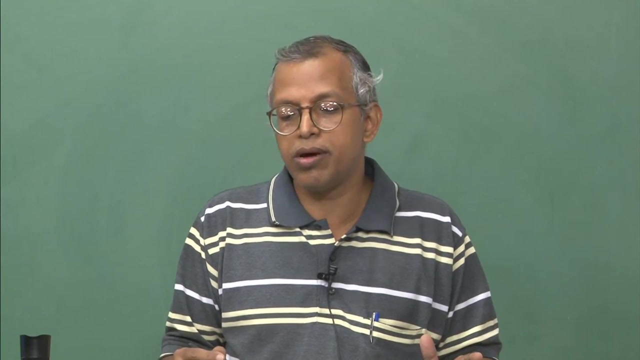 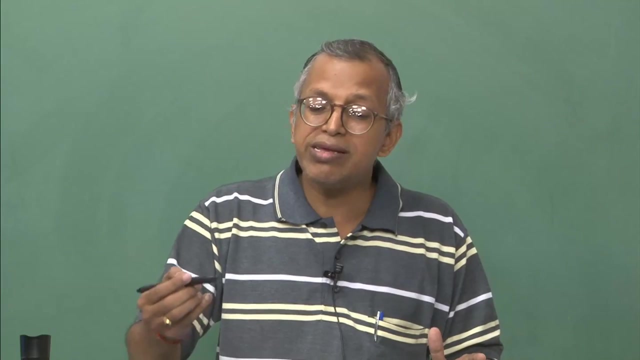 flow in general. of course, we will be mostly dealing with the subsonic flow and supersonic flow. So in our analysis and hypersonic we need would not be really looking at it during our what you call this course or discussion on this course and question is: what is the difference? 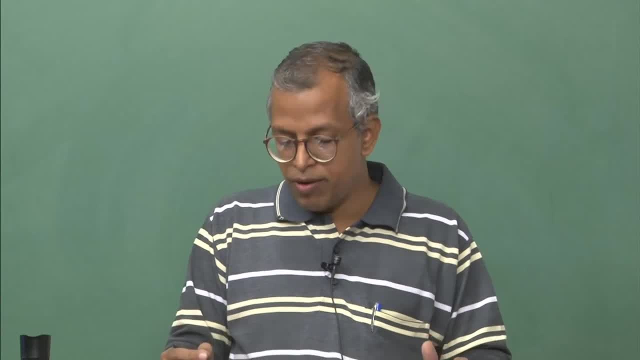 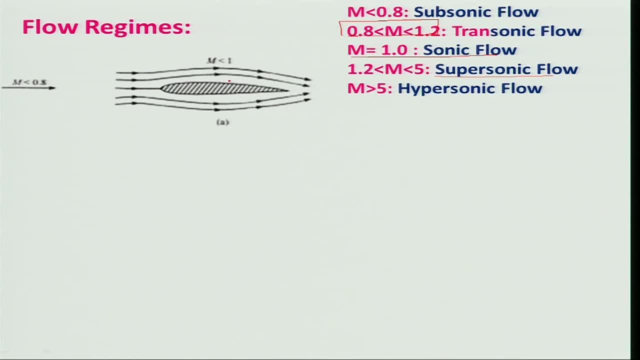 when we can call it as a flow, to be subsonic. for that, let us consider a flow over a, an aerofoil. What it indicates here, it will be subsonic. if it is subsonic throughout this region, then we call it as a subsonic flow. 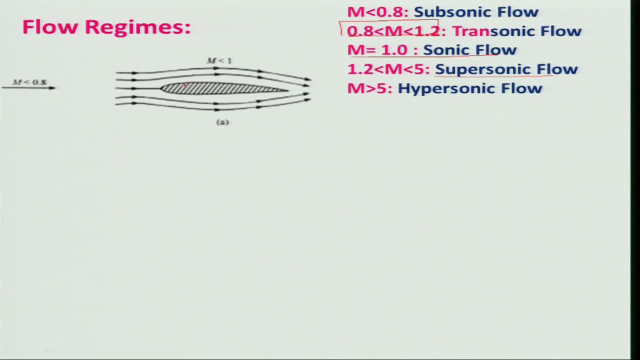 But I am having a doubt why this stream lines are move. you know is like this: if flow is coming Right. So for example, if flow is coming over here, you know something like this: uniform flow, let us in a wind tunnel, kind of things, because uniform flow in nature is difficult to get. 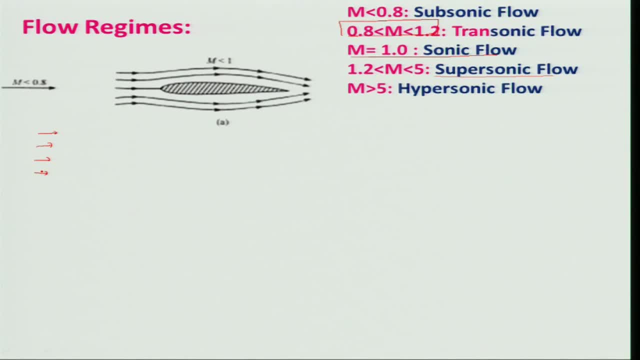 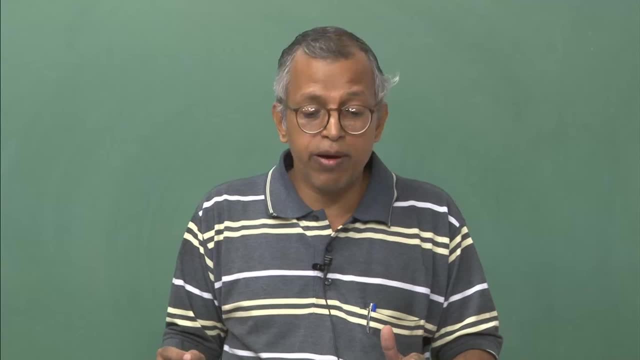 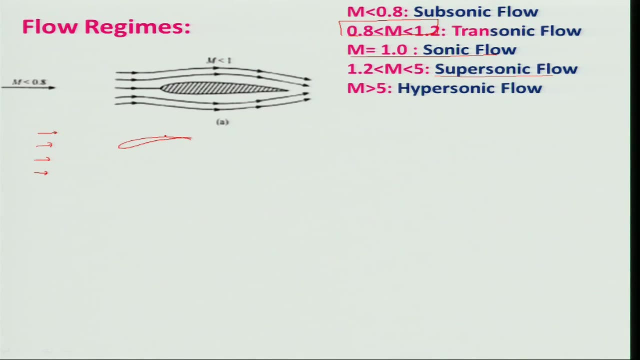 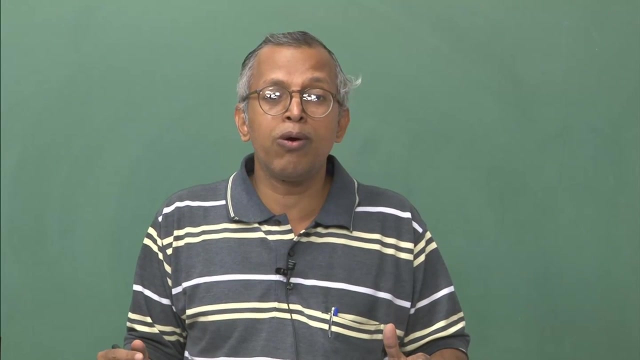 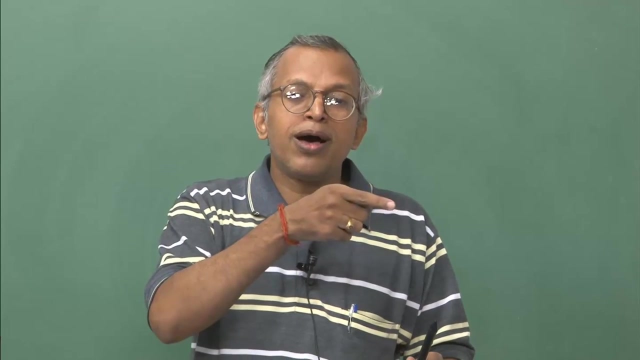 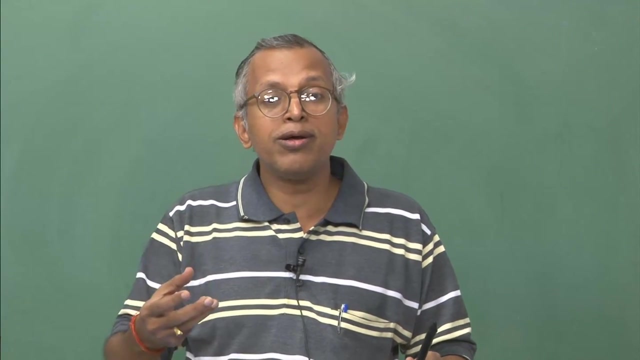 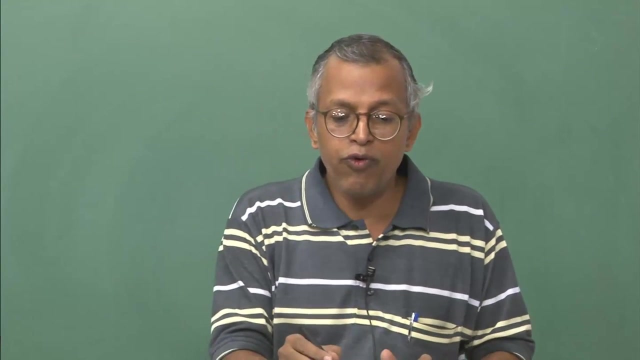 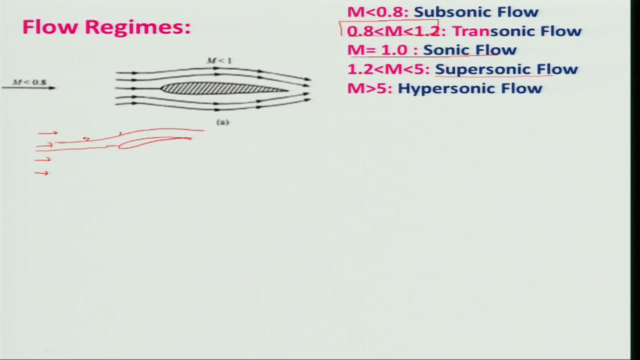 right. So and then what I will do? I will put a body like a slender body or aerodynamic or aerofoil right. So if it is coming, it changes its path or the stream. these are basically stream lines or path and move. that means it is smart enough to say that yes, there is a body I need to. 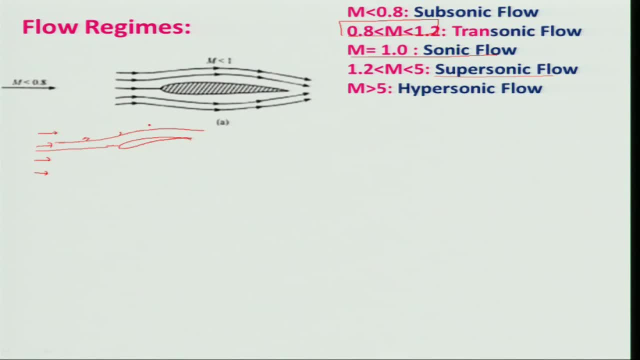 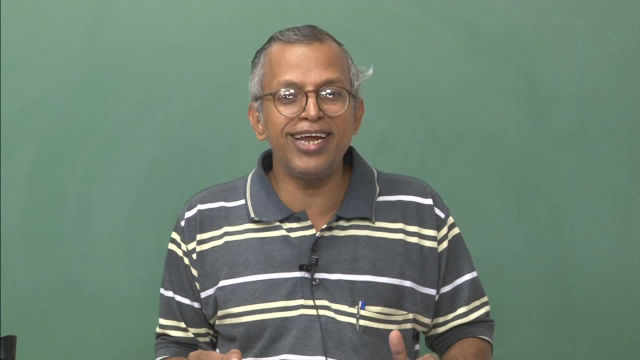 go in such a way that I would not bump into it. for example, if it goes this way, for example, if I say: this is fluid, is going here directly heating the body, you will get hot. am I right? Is it so that means the fluid element is intelligent, like human being, whereas when 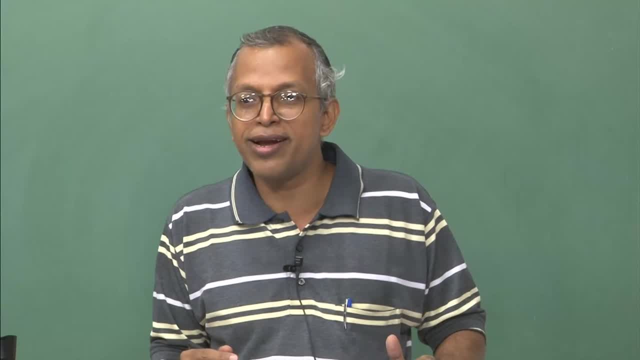 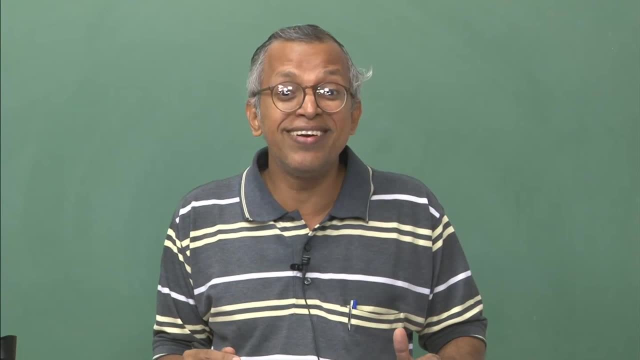 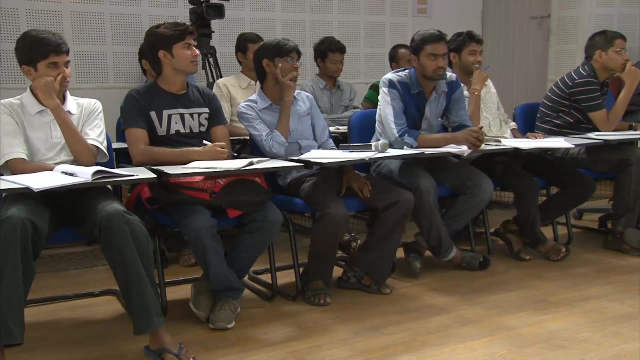 I see our traffic and other things. we are not intelligent enough. we just get bumped into it, right? we do quarrel. we bumped into the people, right? that means fluid. fluid element is smarter than us or intelligent than us. am I right then? how does it do? there is no. 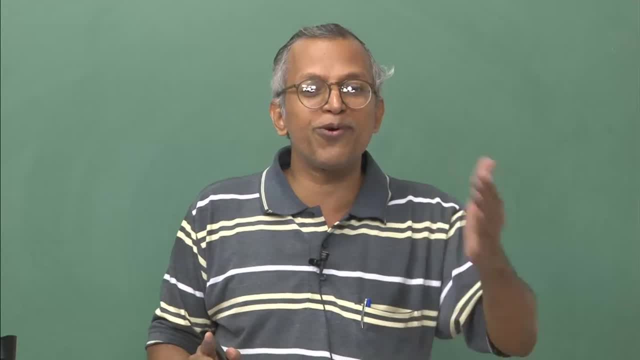 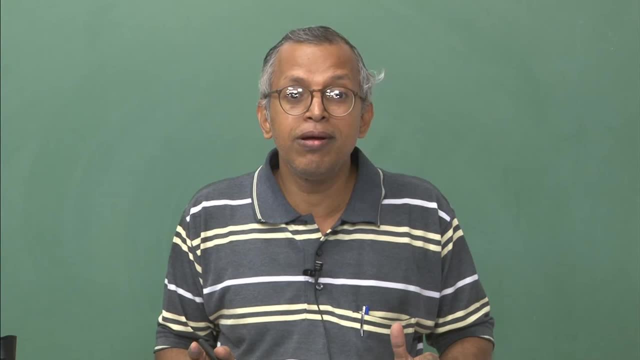 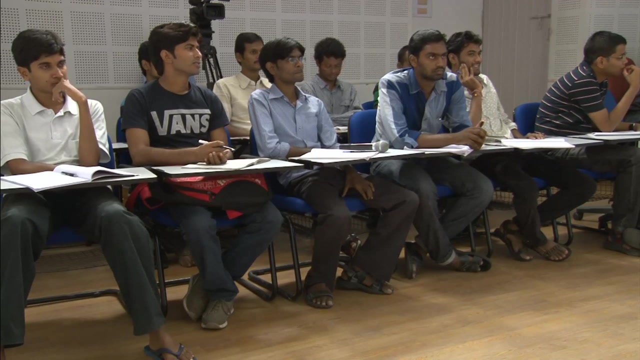 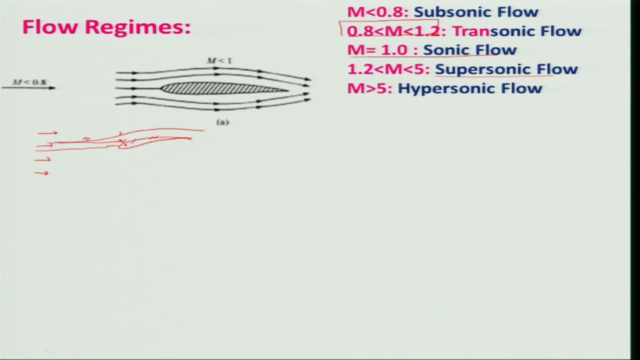 policeman to say that: Look, go, follow this traffic rule, go this way. there will be problem. you know, is there anything nature has given? no, are you sure it is nature has given. that means if there is a body here, right, and if the fluid is there, then it will be coming. of course, some fluid will be coming. 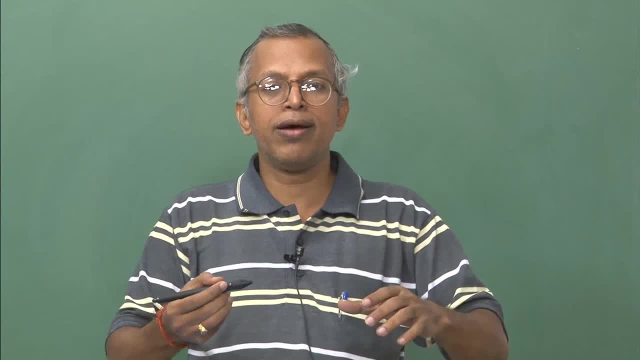 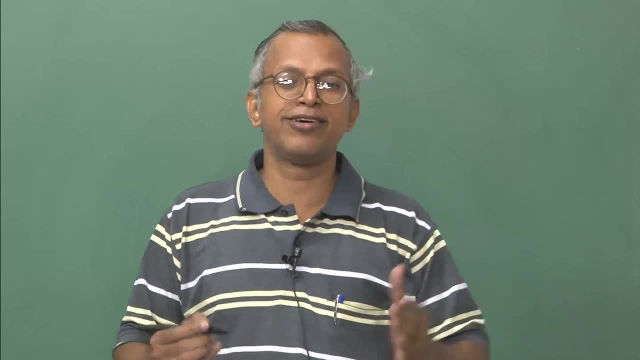 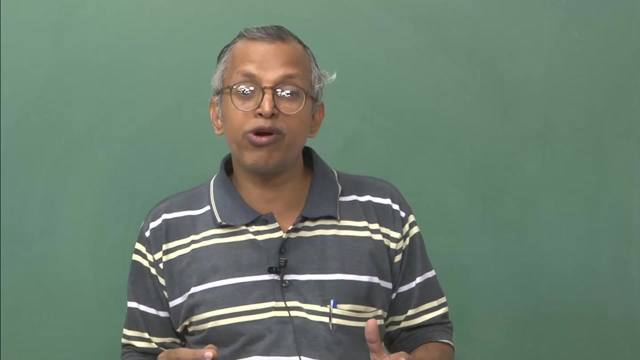 in the beginning. Suppose there is a fluid and I put a body here, then it will give a sound wave and it will be moving with the speed of sound right, and it will make the aware, the fluid element, to say: look, there is a body you should take. 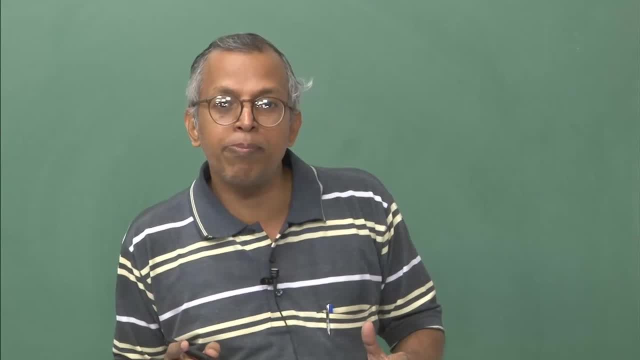 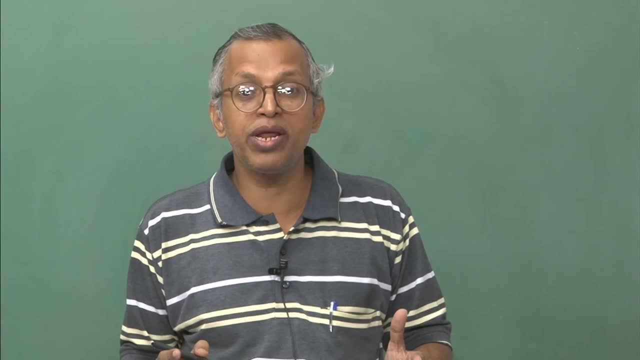 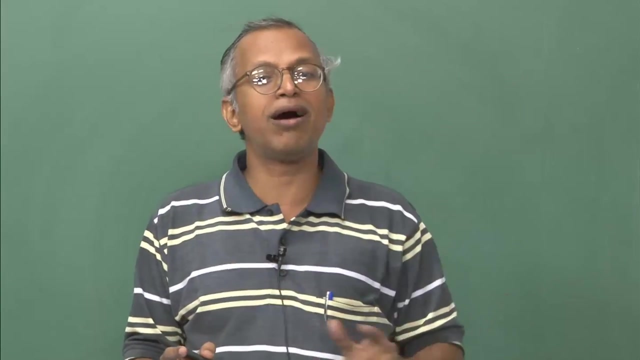 a movement or change your path properly, otherwise you will hit on it. are you getting my point? this is very important point I am talking about. Therefore, the speed of sound is very, very important. when you talk about Mach, number right, I could have put any other ratio, So 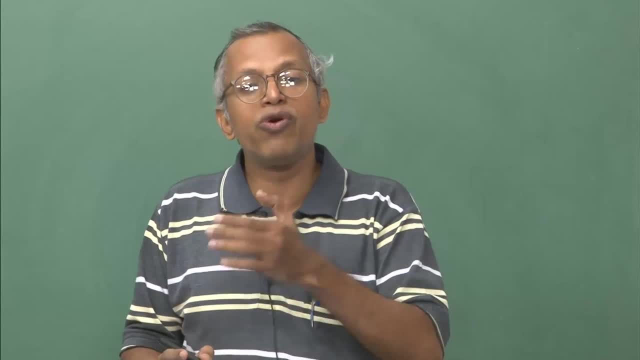 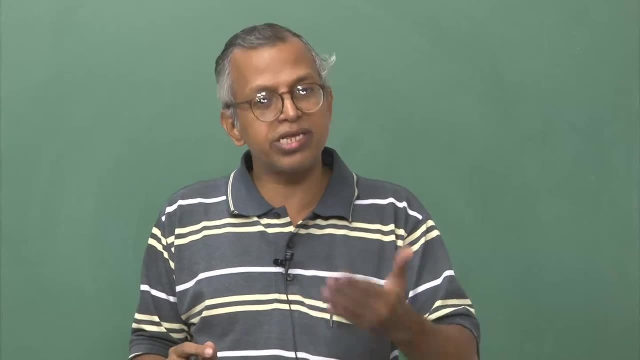 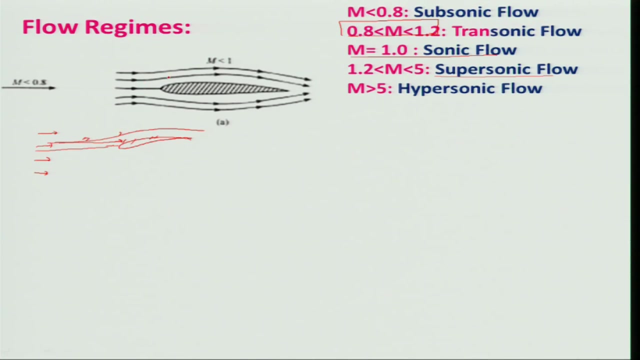 therefore, the Mach number plays a very important role to define or to divide the flow regime. whether it is compressible or incompressible, that we will learn as you go along. there is one thing, and other thing is that if the fluid element is moving here, 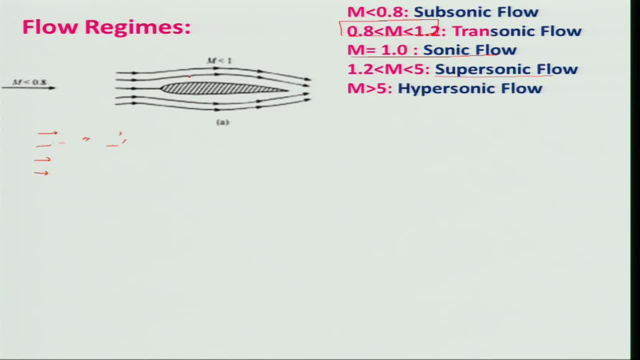 Then what is happening to this stream lines? these stream lines are coming, but if you look at, there is a here, there is a curvature of this body. if it is there, the whatever in figure this stream lines are drawn. is it right? For example, if I put a line here, this is: 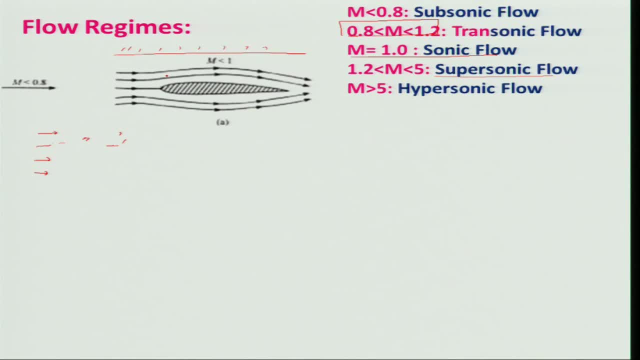 my boundary. you know, then, what will happen if I take this cross sectional area. but simple argument. I will say What will happen? this: there is a decrease in area, right decrease in area. what will happen? you know from your previous learning, right, there will be acceleration if there is acceleration. 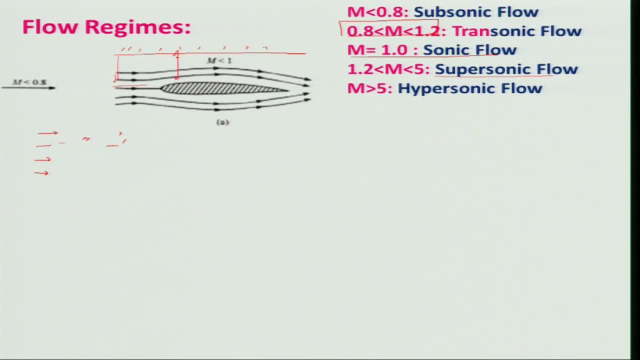 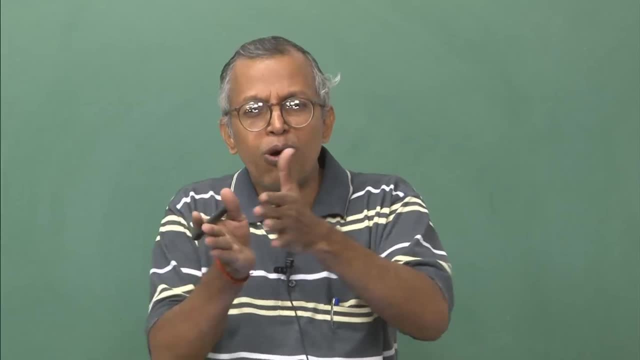 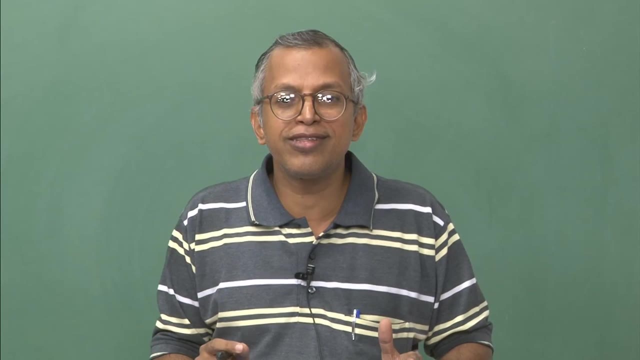 of the flow. what will happen to stream line? It will not only deviate, but it will be crowded. it will be coming through. you know, closer, coming closer to that. I would suggest that you please read something about The stream line stream tubes. you know. if it is a circular one, you know what will be dealing. 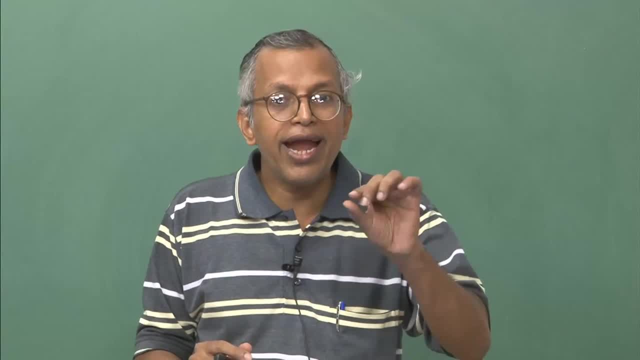 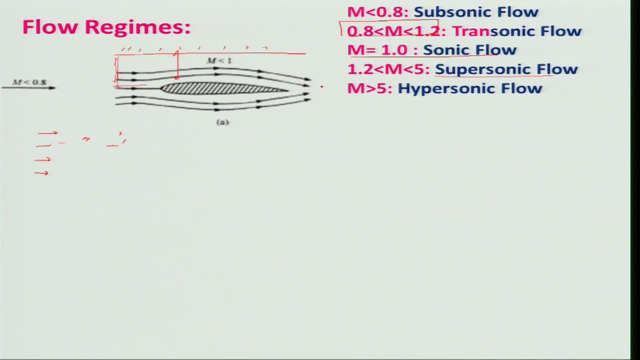 with our propulsive devices, right, and this mass, because mass has to be same, mass has to move into. So whatever the mass is flowing in this region- I have taken half of that- same mass has to be move into right, in the same smaller area. Therefore, there will be decrease. 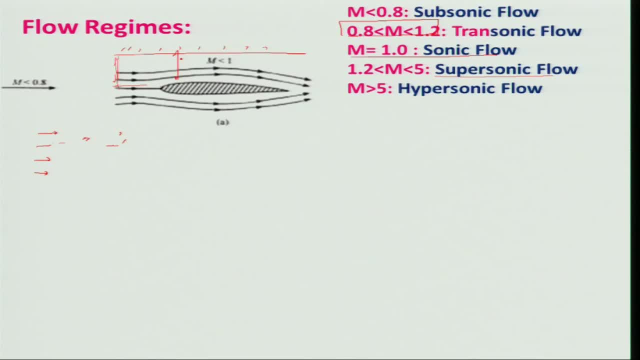 in velocity and the stream line will be coming closer to each other. But however, it is not drawn here, and if it is drawn, then- or it is- that means the fluid velocity will be here more than the what is the free stream velocity at this point. are 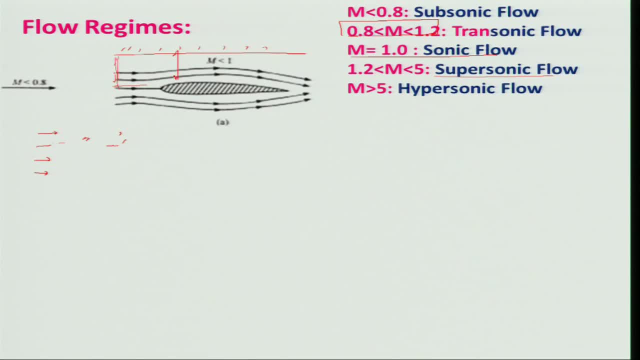 you getting my point. So therefore it is very important. then there will be increase in the fluid flow here and, as I told you, that there will be also deceleration here in this region, there will be change in the Mach number. That means local Mach number in this region will be changing. am I right if this is 0.8? 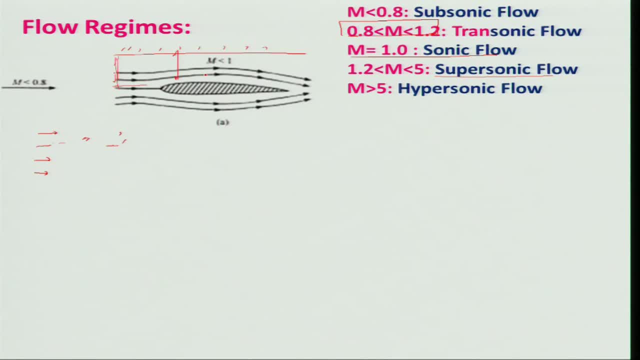 will it be 0.8 throughout. it will be somewhere higher, somewhere lower than the 0.8 if I take, or if it is 0.5, then it will be different. right, That means this region, local Mach number of the fluid which is moving around. it will be different. 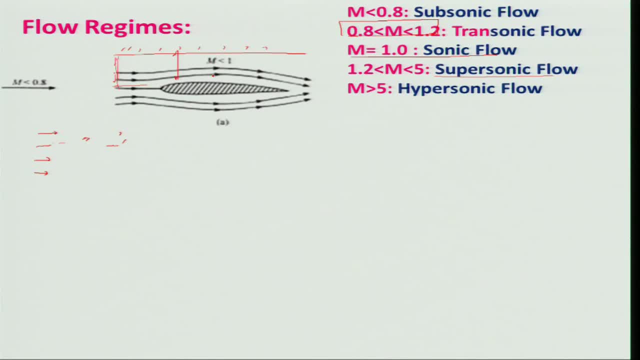 Now, if I increase my free stream Mach number to in the range of 0.8 to 1.2, what happens? for example, let us say my Mach number is around 0.9.. That means here it is 0.9. this, 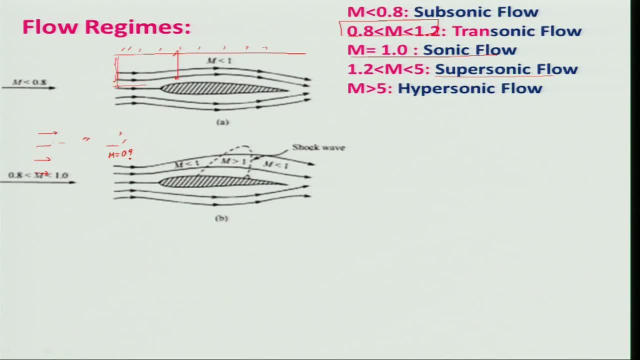 is the free stream. I can write down: this is 0.9, let us say, and fluid will be moving. there will be, You know, acceleration of the flow also, but it will be less than 1, and there is a regime where it is greater than 1.. And if it is greater than 1, there will be a shock wave which will 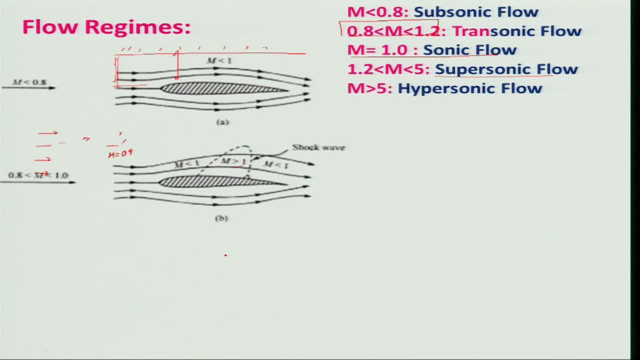 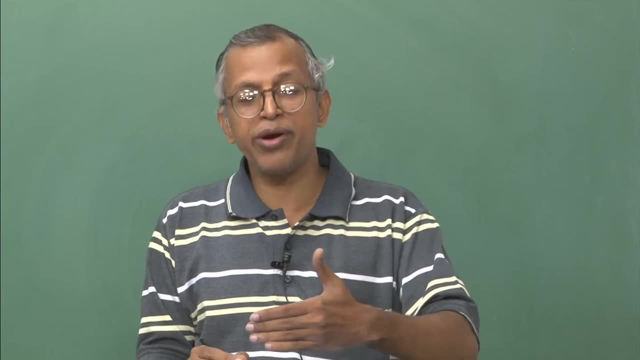 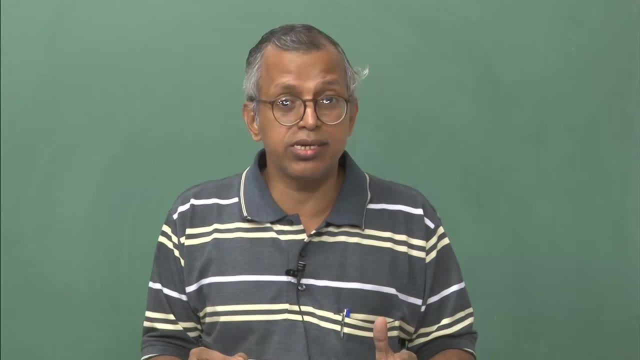 be discussing about this. basically, there will be discontinuities in the flow properties, and discontinuities means what it would not be. the stream line would not be that smooth. if you microscopically look at A staged shock is being formed that we will see. when are you are discussing right and 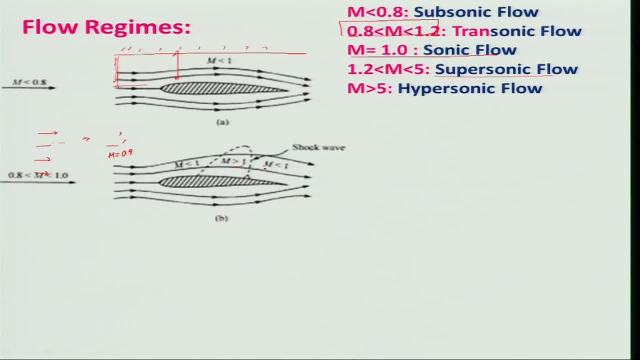 therefore, at the downstream of this, There will be Mach number will be less than 1. keep in mind that, sad as shown, only one shock wave on the upper portion of the stream, what you call aου foil. What happens to the lower one? will it not be a in this figure? it is not. 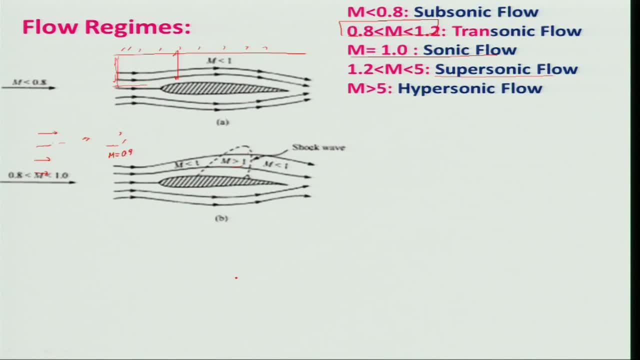 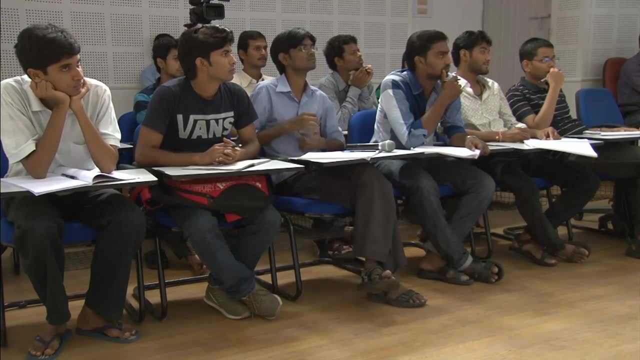 Will it be there or not Not there? in this figure it is not there. Will it there or not? That region of the stream, actually, none of you had problem? not, there would not be, is not it? am I right? But non symmetric, it would not be there. 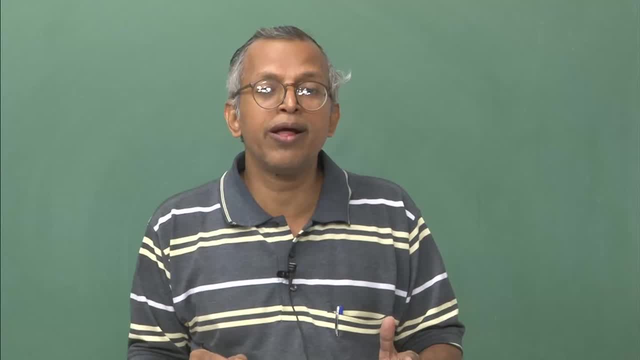 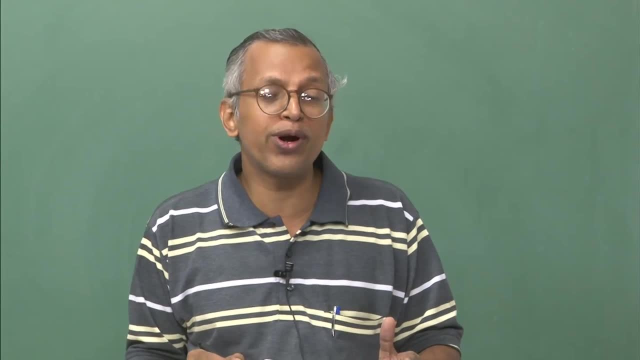 Angle of attack. that will be dependent on- and here we are assuming- the flow is not separated. If flow is separated, then this stream lines, whatever I have shown here, would hold good, depending on whether, where it is separated, all stream lines has to be changing right. 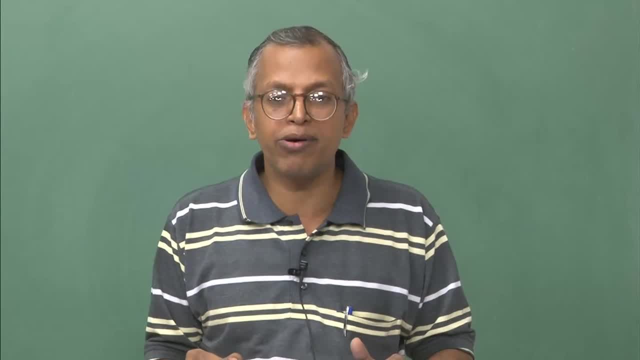 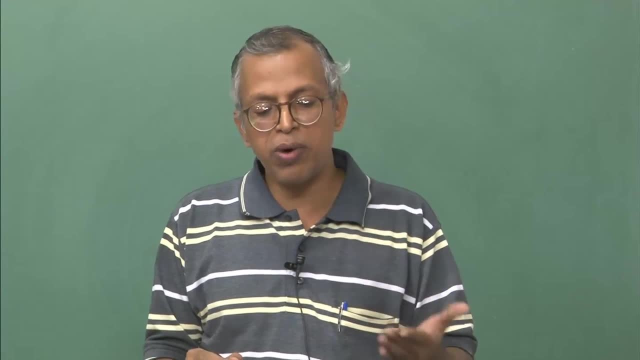 So therefore, we are not considering what you are talking about. we are considering whether, in this case, flow is not separated. That means angle of attack is not small and there is no angle of attack here. you can look at it. this figure does not show that it is a angle. 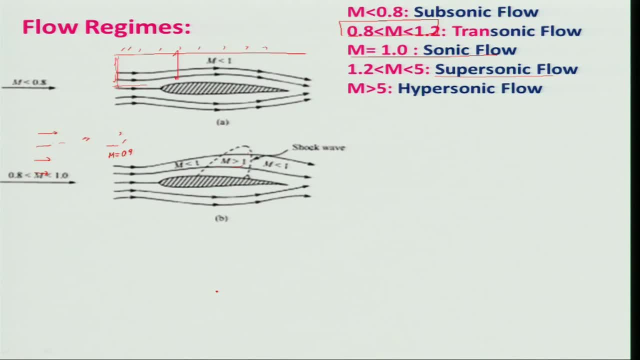 of attack. it is a just. angle of attack is 0 in this case. So, therefore, what will be? whether the shock wave will be there, this region, or not. If it is there, there will be. if it is there, then where it will be located? will it be located exactly, symmetric, in this? 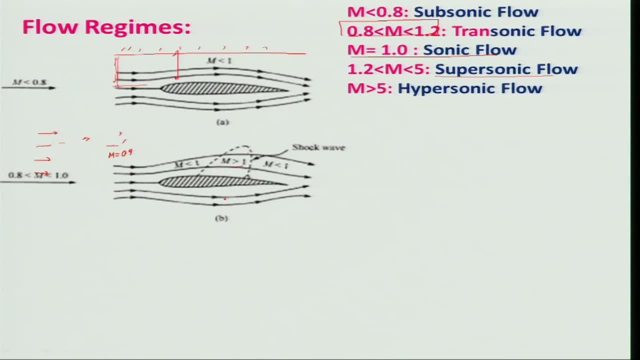 region. or it will be here or it will be there. It is quite difficult to say, but however, one can guess that it will be little downstream because of this region- you can look at this surface right- There will be the. when the Mach number will be greater than 1 will be. 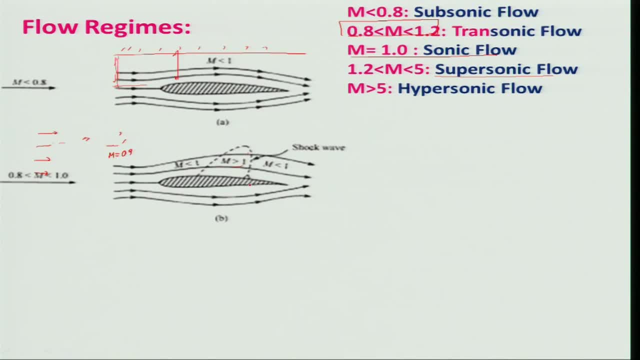 attaining little bit down right, Because if you look at the surface, you can see that. So therefore, you please think about it and then, you know, have a feel, for it is very important. And now let us look at a flow. you know, here we have considered 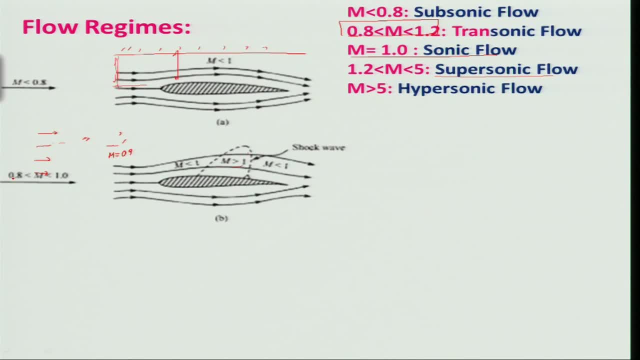 the Mach number range of the flow between the 0.8 to the 1 right, However, the trans sonic flow. it is one reason That means we are considering something 0.8 to sonic condition. you can ask me a question why you are So particular about 0.8, is it? 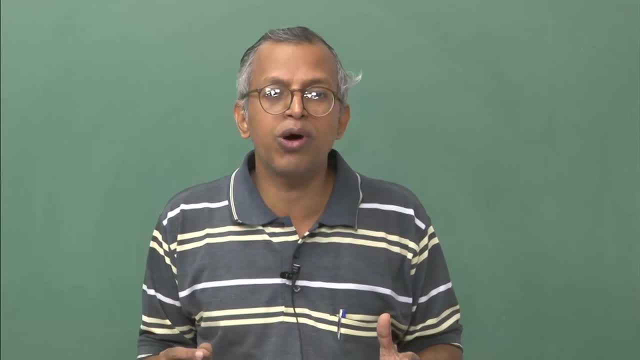 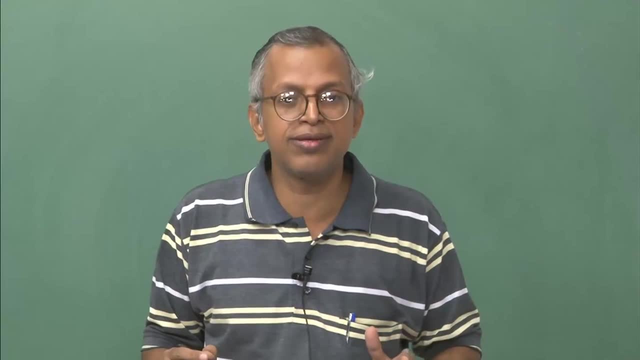 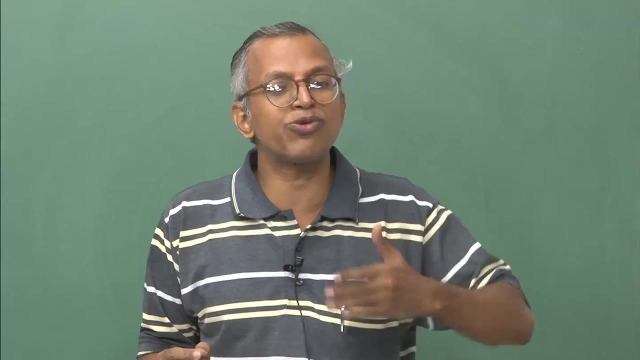 something you know So sacrosanct or magical number that it will be the same for all the time, or is there any basis? is it that question coming to your mind or not, because it is written in book? that is why we will have to take, am I right? 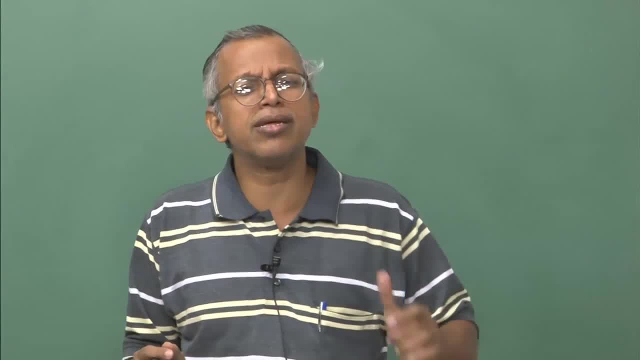 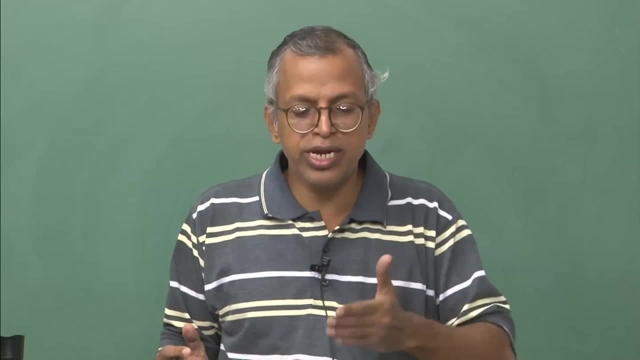 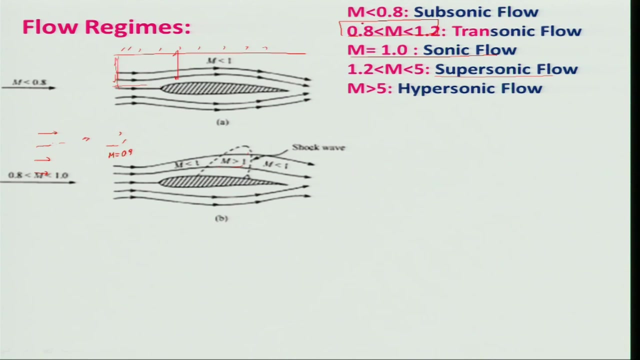 There is nothing sacrosanct about it, is just a mere thumb rule which is being done. it may be different when you conduct experiment, suppose in case of what you call streamline body. if I take a body, naturally this, you know numbers. what is given here, like 0.8,, 1.2,, 5, need not. 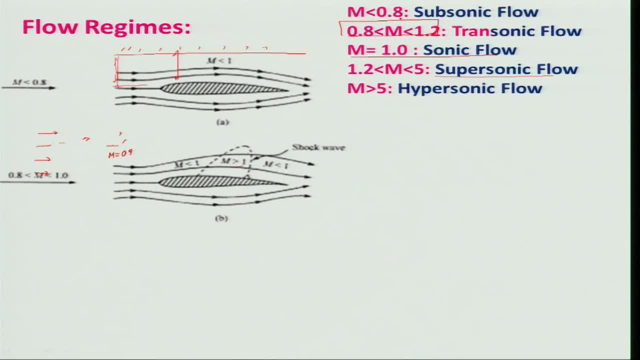 to be the same. it will be generally. For example, when you go for this subsonic flow regime in, it will be much lower than 0.8 when you talk about a flow over blob body, or some people call it as a blend body. So please, you should develop a feel for it, do not just remember. 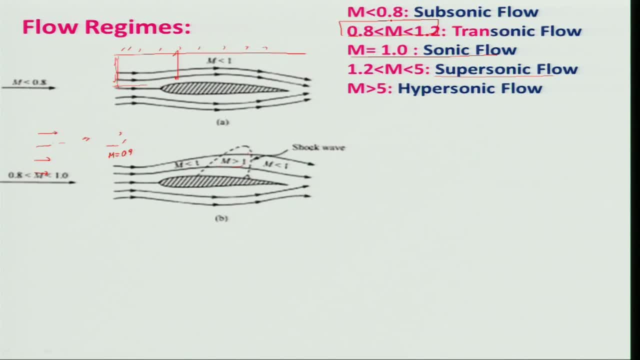 the number, but you need to remember the number, but you should know what is the limitation. So, coming back to this, that then we need to understand what happens when the flow is between the 1. 1 to 1.2. that is, the transonic region. What will happen if the free stream here you know. 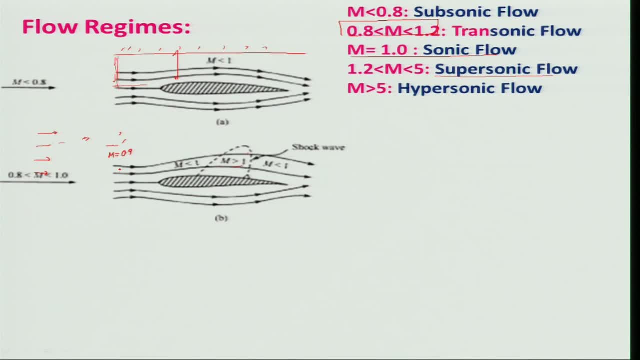 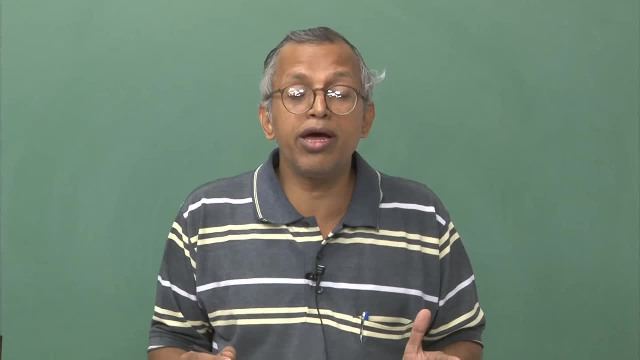 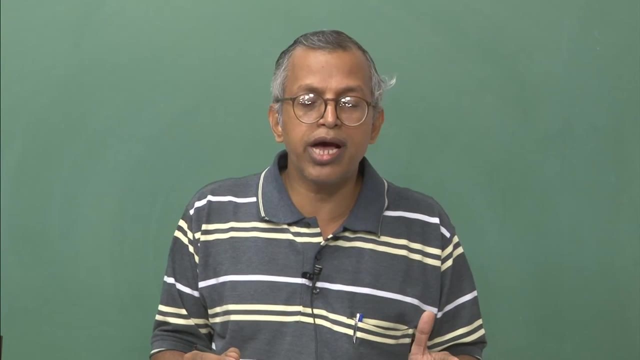 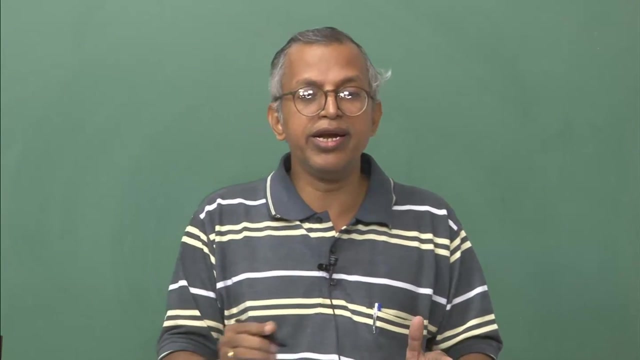 is not really, it is greater than 1,. what will happen? There will be, there will be shock. where there will be shock, it will be leading edge, nearby leading edge, or it is away from the leading edge, or it is somewhere downstream, you know, of the leading edge where it will. 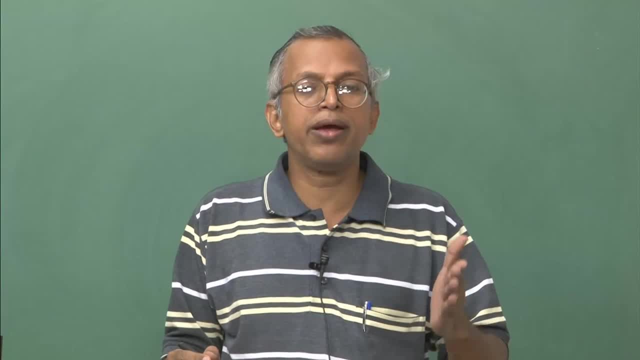 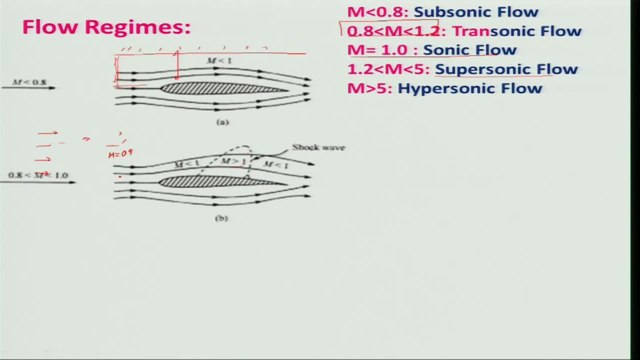 be. it will be, you know, before the leading edge, away from the leading edge, towards the you know flow or the main stream, upstream. rather, That means my shock will be like this, and this is considered as a bow shock because it is like a bow, The shape of the bow. and then when the flow is, let us say, Mach number, which is greater, 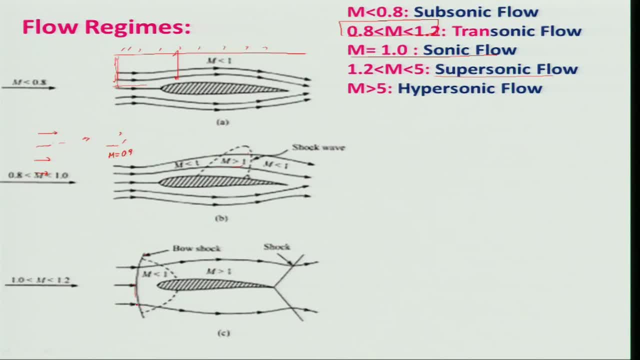 than 1, then the downstream of this bow shock Mach number will be less than 1.. Why it is so we will see. may be when we will discuss about the shock, and then after that it became accelerated and in this region The flow will be what you call supersonic M is greater than 1, Mach number is greater. 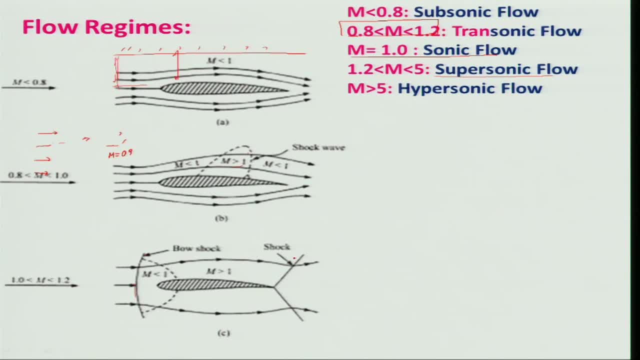 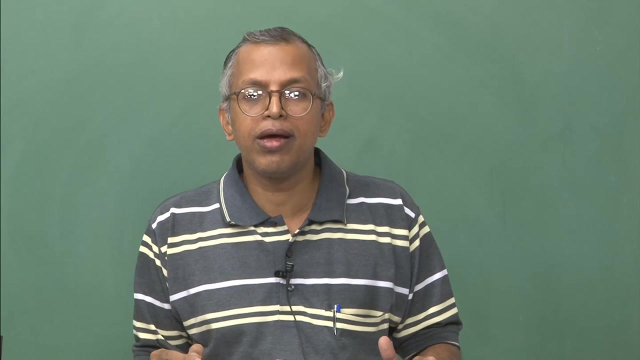 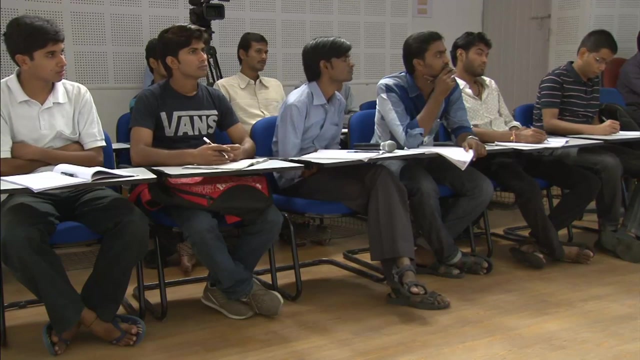 than 1.. And then there will be also a shock which will be here at the trailing edge, both the upper portion and the lower portion, and it looks like what. can anybody tell me this? two shocks. Have you never observe what? no, this is shock, it is not expansion wave. but I am asking. 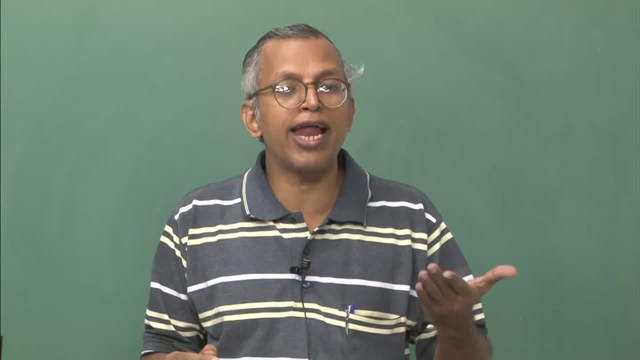 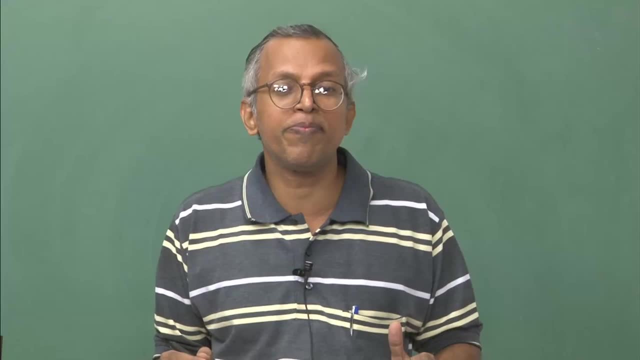 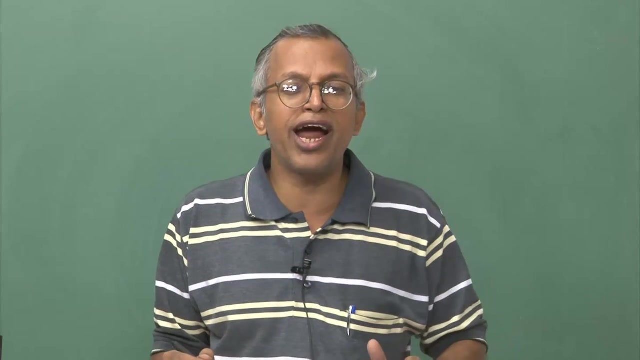 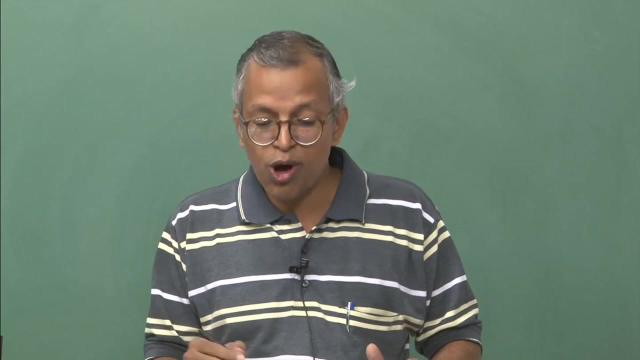 you? what is the shape you can have? have you never seen a fish? did you look at the fish shape? is it not like an aerodynamic body or aerofoil? I mean similar to that? it is having a tail. So this sock, we call it as a sex. See when. 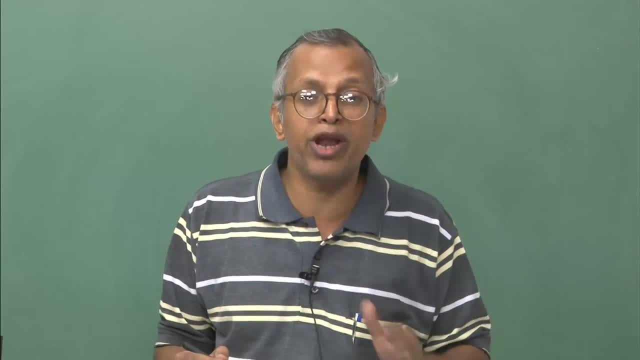 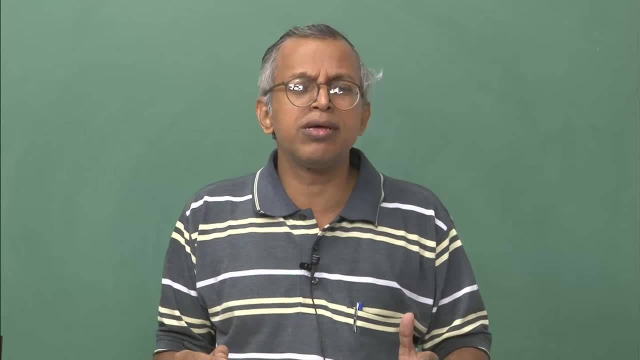 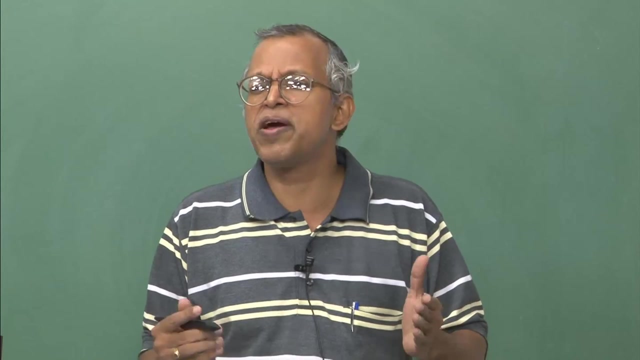 you look at nature, you should have a good observation power and try to relate what you learn and what they are having. If you look at, most of the science, whatever we are using, has come from the nature, So nature is a great teacher to us. we must observe the nature. 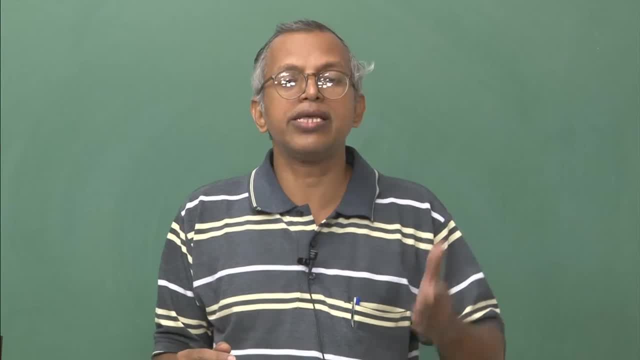 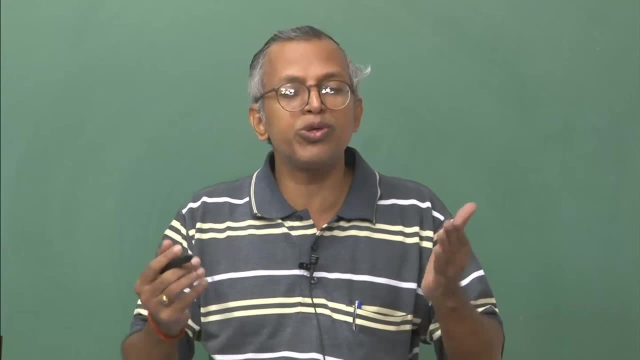 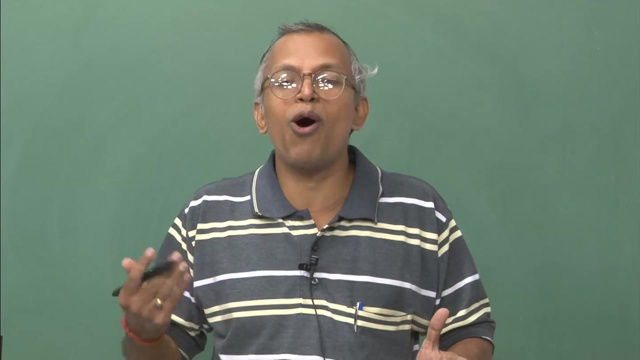 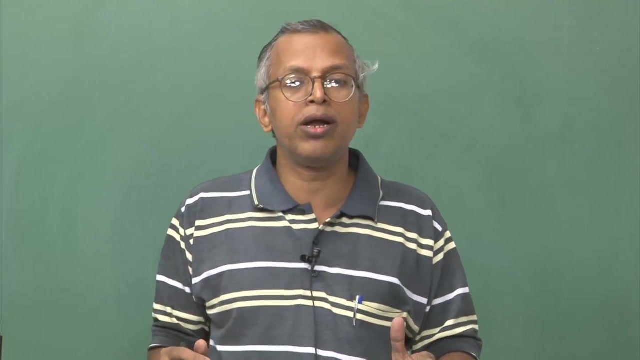 as closely as possible, As I always say that we need to learn how to live with the nature, not live against the nature, because he is the. you know, our mother sustains our all activities without any garage in mind. This feeling is very important to when you are doing the science, technology or life any 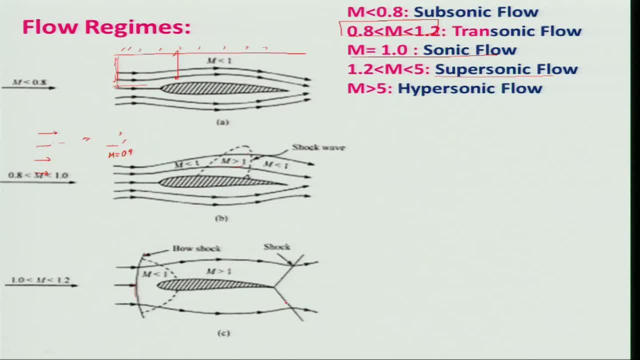 other thing. So therefore we need to learn this is known as feast tail sock. Of course there is a little complex. it is here involved. we would not discuss at this moment, But however, some of you are interested, you can look at it and keep in mind that in transonic 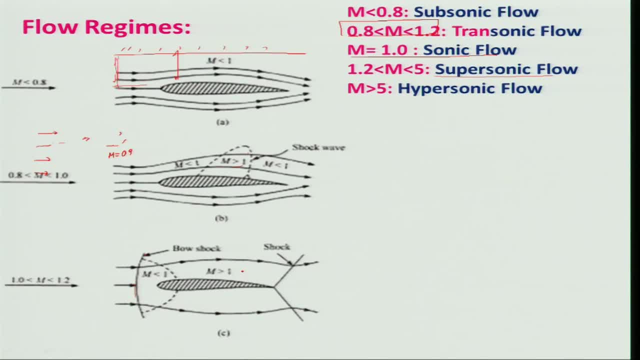 flow, we get the flow subsonic, supersonic and combination, which is quite difficult to solve mathematically. as such, And you will see that here also in this regime, the Mach number less than 1, Mach number greater than 1, we says that it is basically supersonic flow. 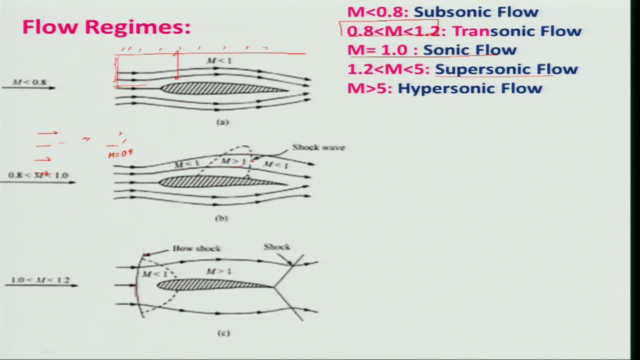 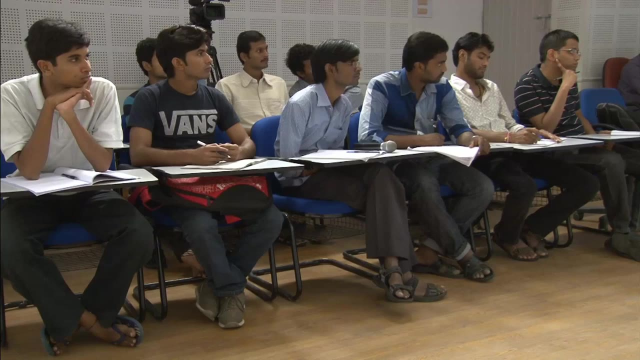 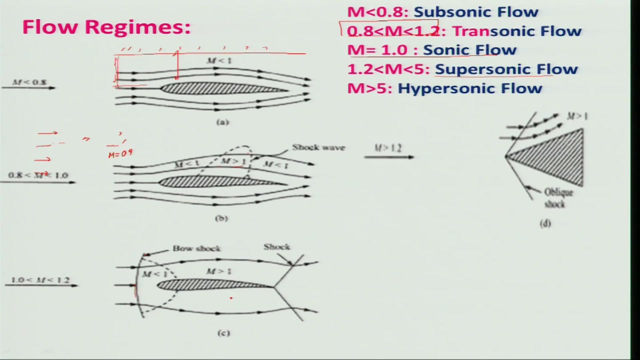 subsonic flow and therefore we call supersonic. subsonic combination is known as the transonic flow. So if I will increase this Mach number beyond 1.2, what will happen? So if I use this here in this, what you call a, an aerofoil or a slender body, then the sock. 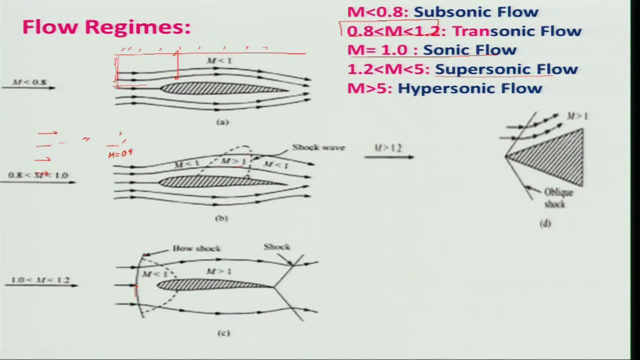 will be similar to your bow sock. And what will happen to the sock strength? it will be much higher. as the Mach number goes, it increases. What do you mean by sock strength? we look at it little later on. So generally people use a wedge. in this case it is wedge or a sharp nose, you know where. 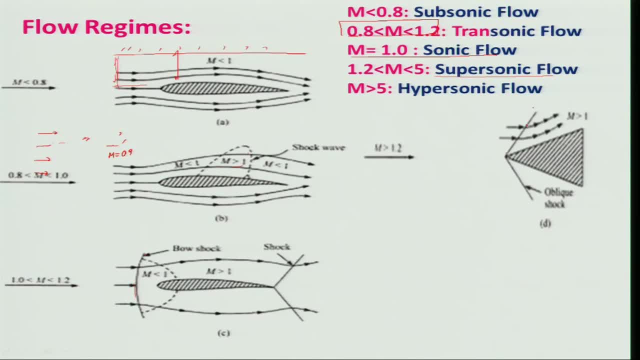 it which the socks are being attach and this socks is attach and makes an angle. therefore we call it as an oblique sock. We, which will be discussing little later on how to handle the oblique sock, how to analyze oblique sock and how we can use. later on we will see particularly- 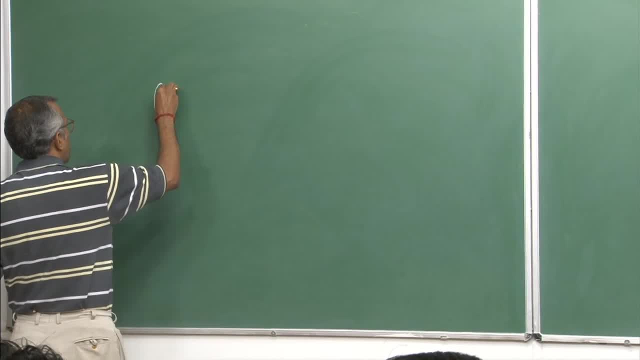 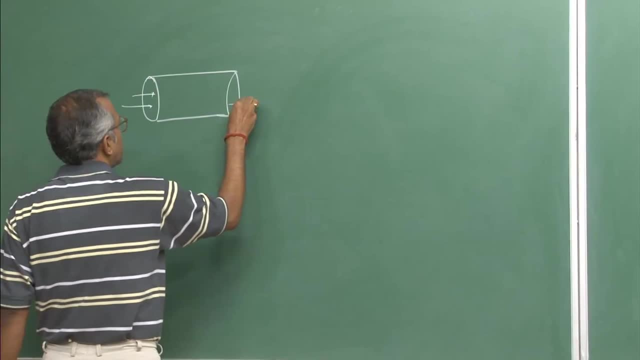 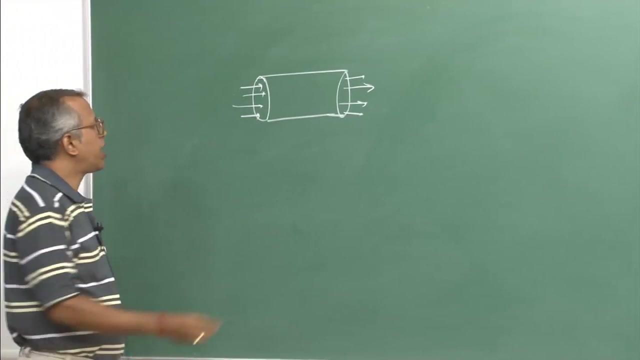 area P shit, more gas juice. and if you applyما to say I will, it will be, it will be 2 dimensional, is it so? in the in the into flow is taking place here, right, and I can say: this is my z direction and this is my 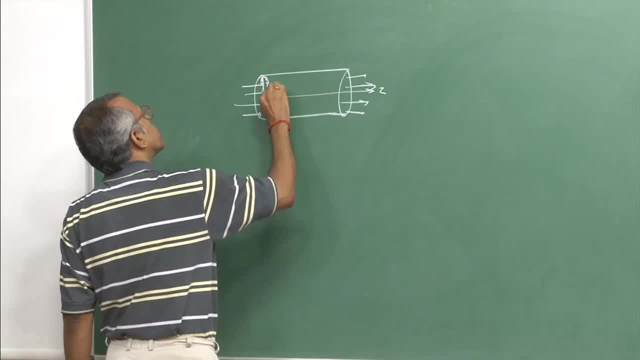 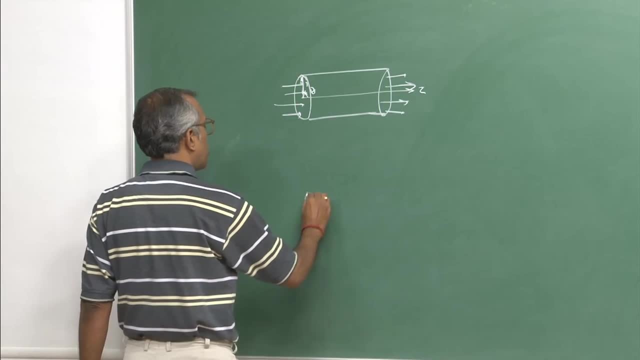 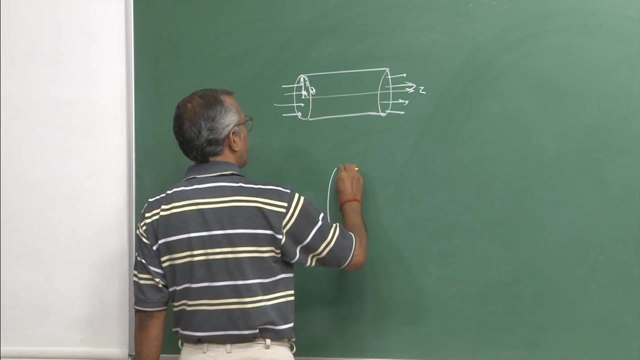 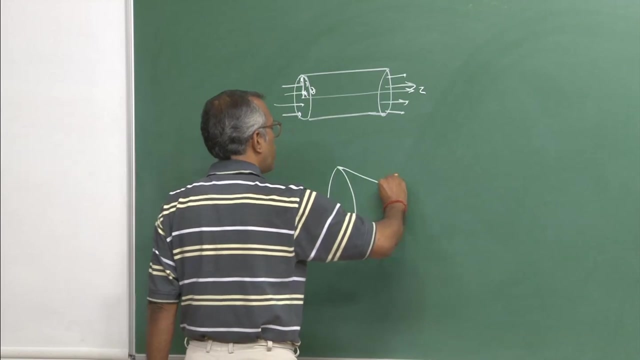 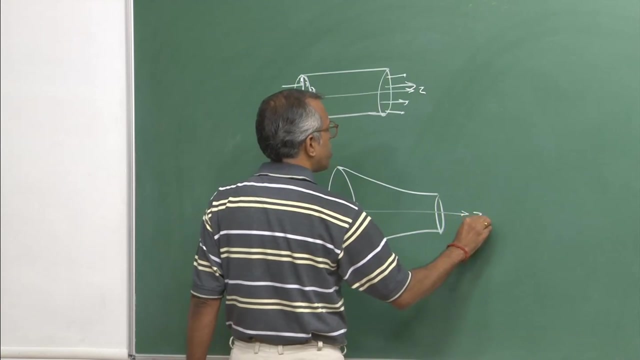 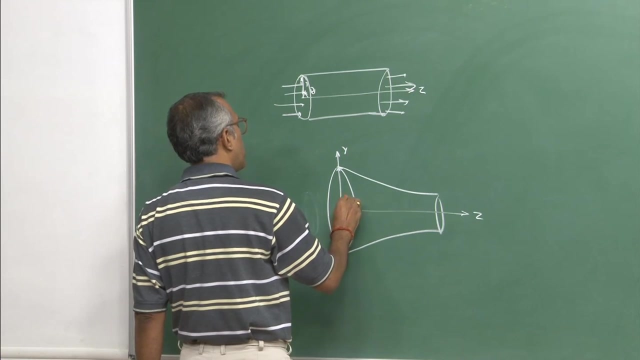 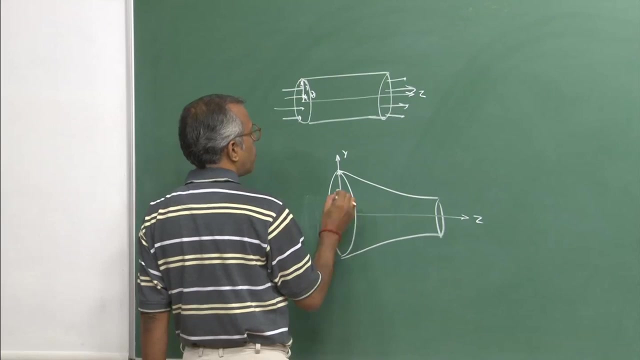 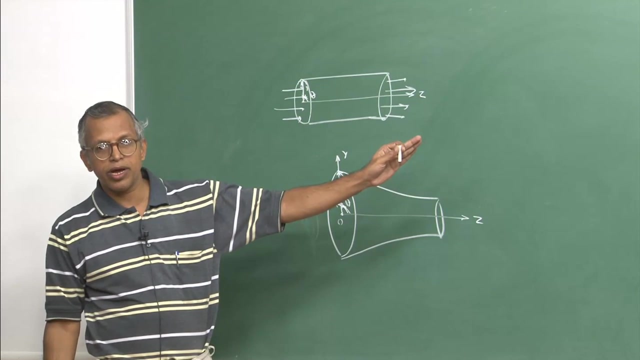 r direction. of course, this will be my theta direction right, And similarly I will take another one, let us say my z direction, r direction, and this is my o and theta direction. In this case, if I look at flow properties, and I will assume there is no boundary layer on the surface, that is also important one. 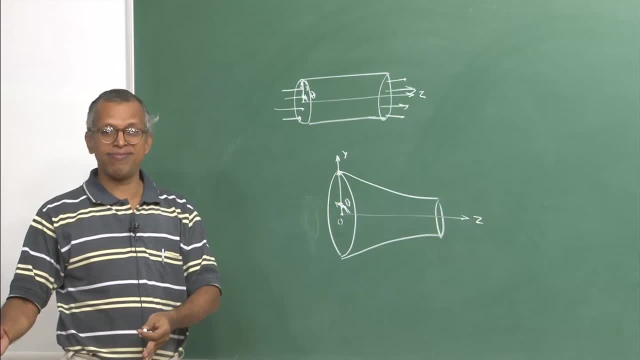 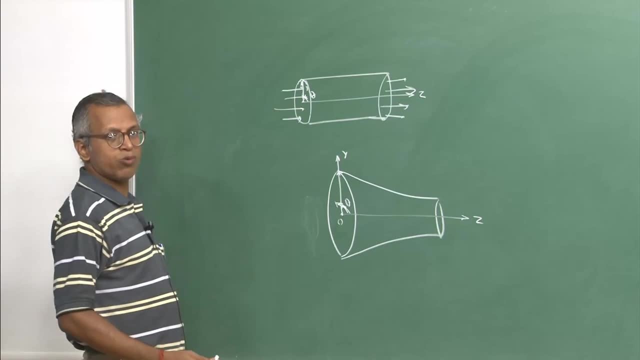 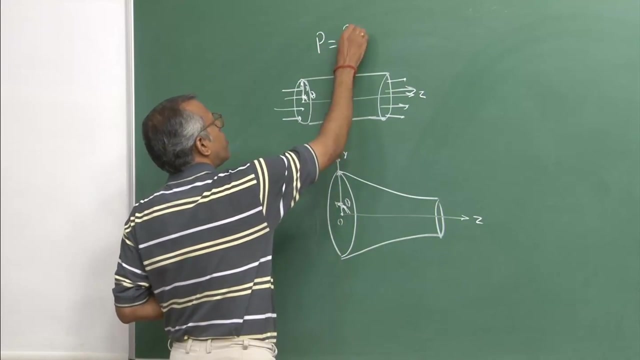 or I will assume it is. a fully developed flow means flow is already developed. here there is no change. that means there is another portion which I have not drawn. Then what will be the properties? let us say pressure at each point will be function of: 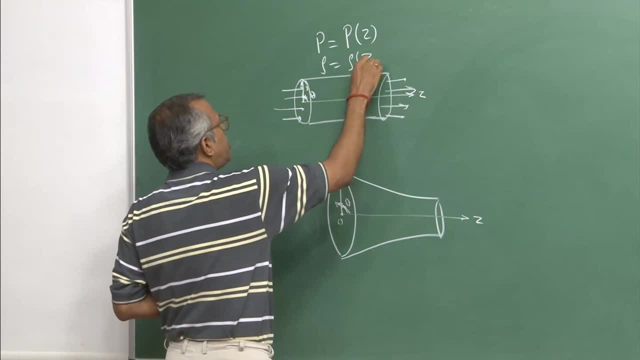 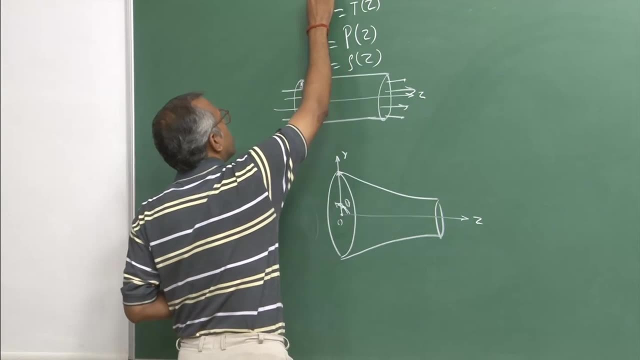 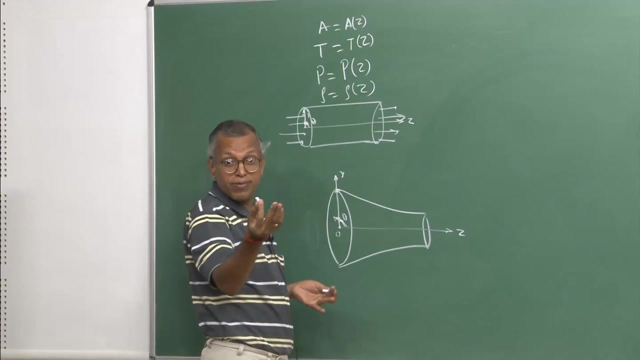 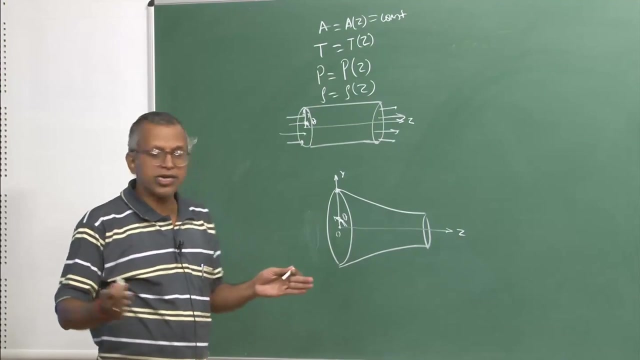 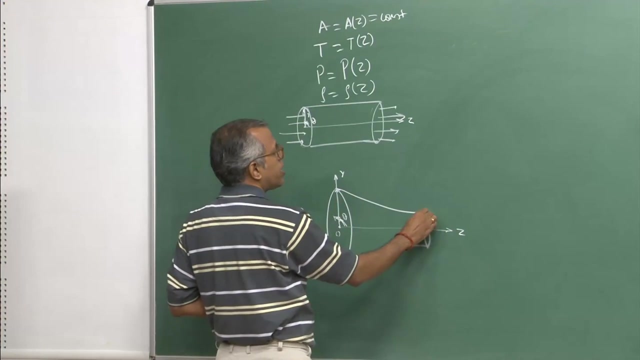 z. rho is a function of z. similarly, temperature is a function of z. and what about area? in this case, area is a function of z or not? it is not a function of z, it is constant. Area is constant, cross sectional area is constant. but in this case, what I will be in reality, 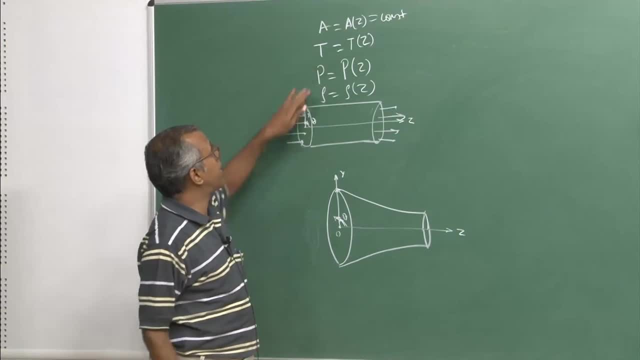 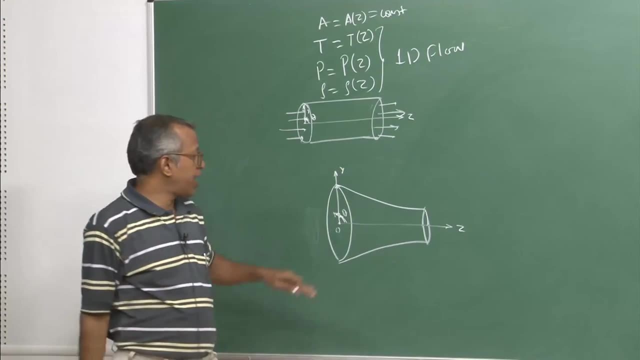 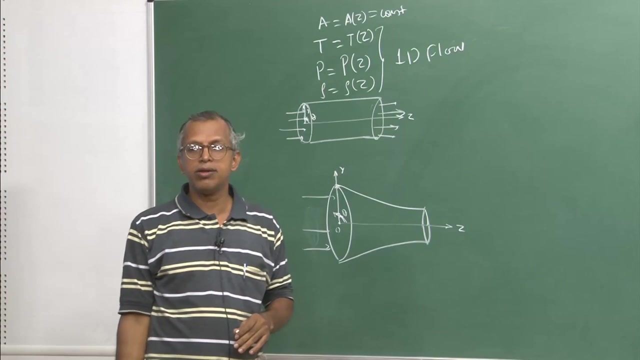 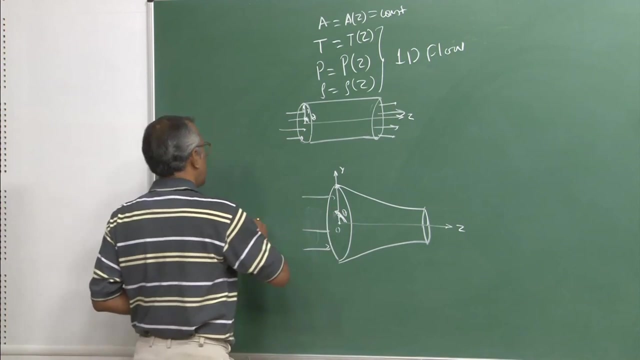 this flow will be not one dimensional. this I can call it as a one dimensional flow. Can I call this flow as a one dimensional? if flow is taking place this way, Can I call? I cannot. in principle it will be three dimensional. but if I say that, theta. 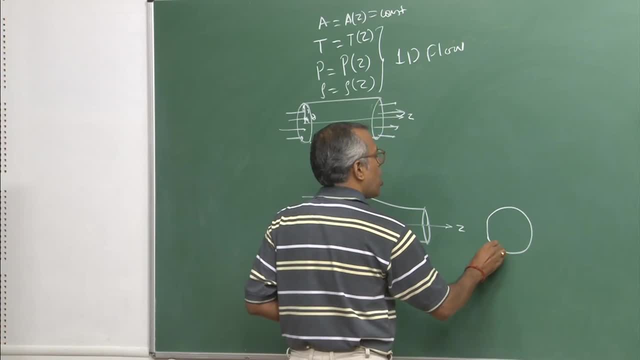 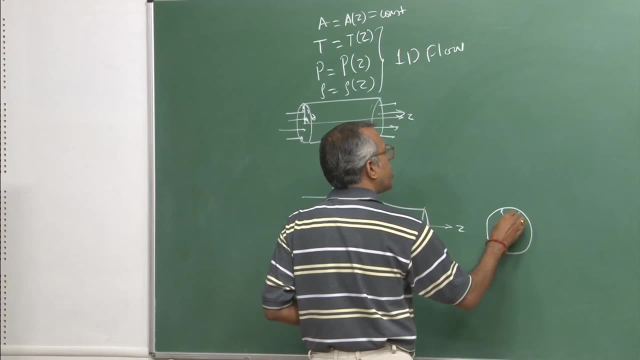 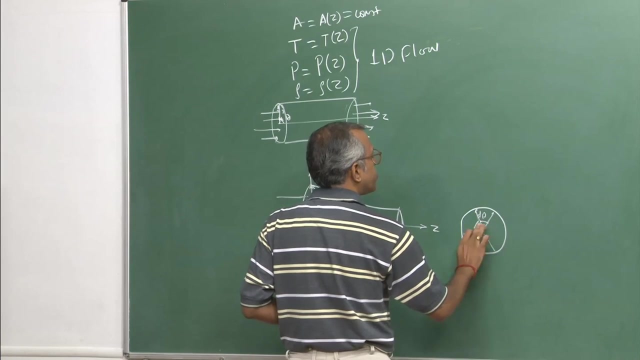 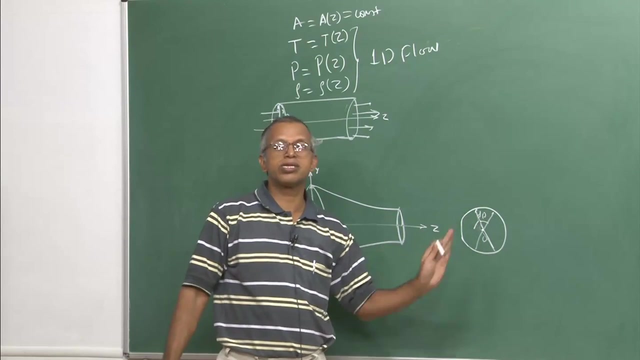 if I draw this and if I take this as a o, like any theta direction, any cross section theta, If I take d theta- you know kind of things, it will be same. So therefore this symmetric is there and everywhere flow is same, then I can say it is two dimensional. now, But if 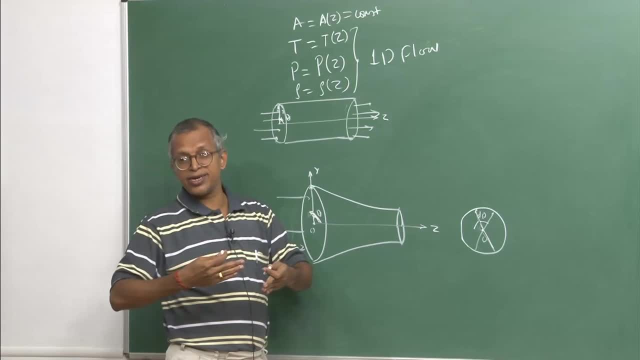 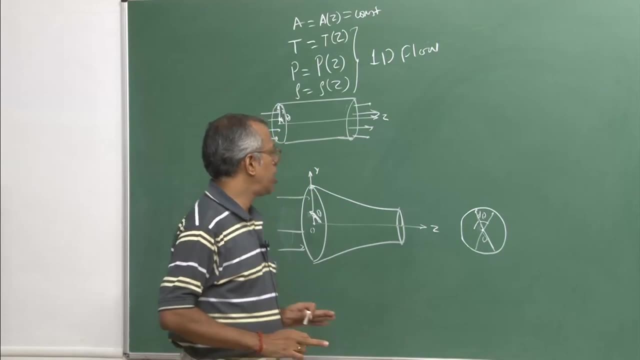 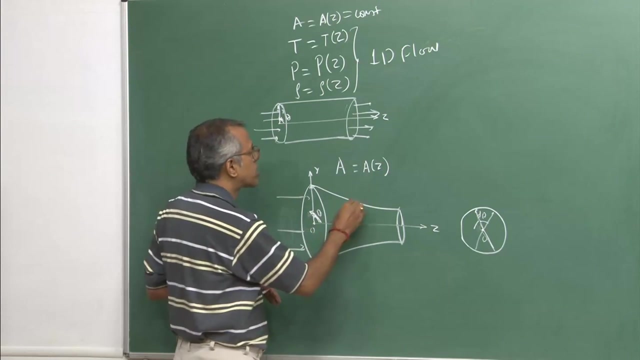 I will assume this is symmetric in the theta direction. therefore I can call it as a two dimensional: one is your z direction, other is your r direction. But if I will say this is area which is changing, because cross sectional area is changing along with the z, but if the 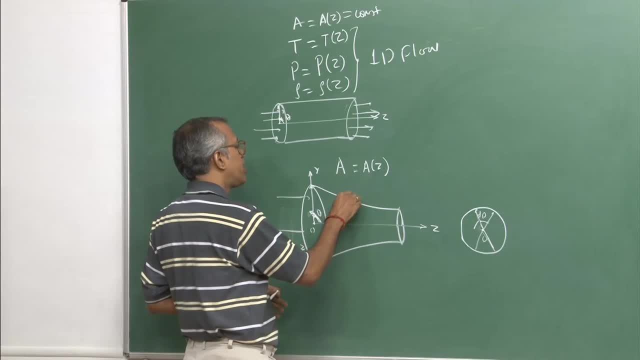 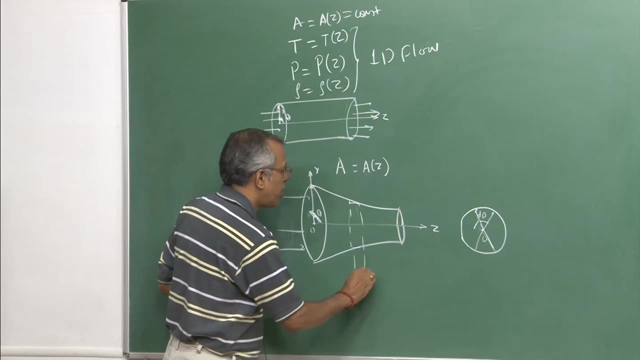 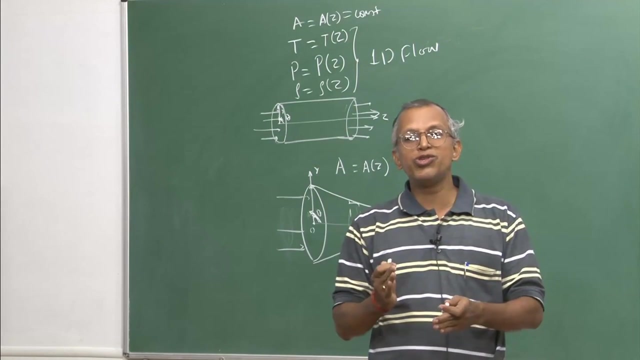 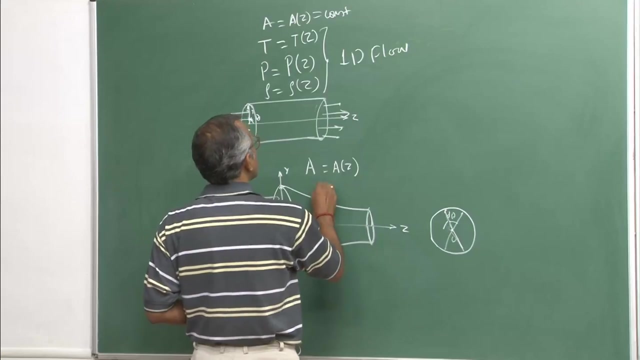 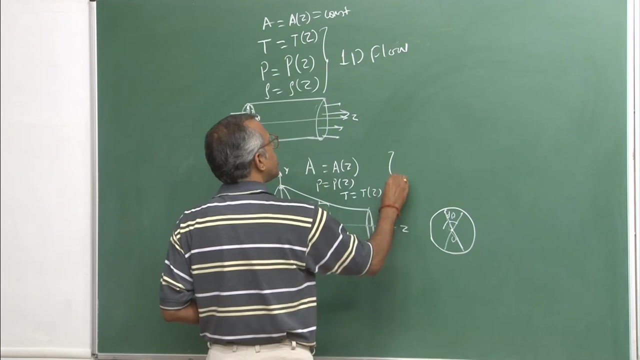 change is very small. If I take an element over here- you know, keep in mind, this is a circular and this is rate at which it is change is taking place- is very small, then I can assume to be quasi one dimensional. That is, p is function of z, similarly t is function of z and all other properties then. 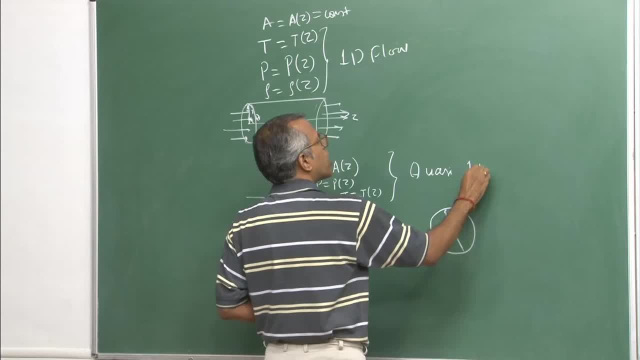 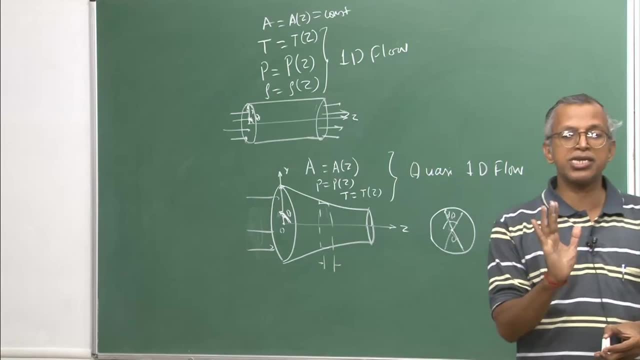 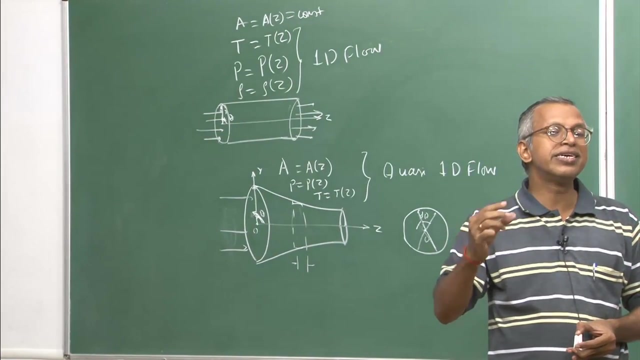 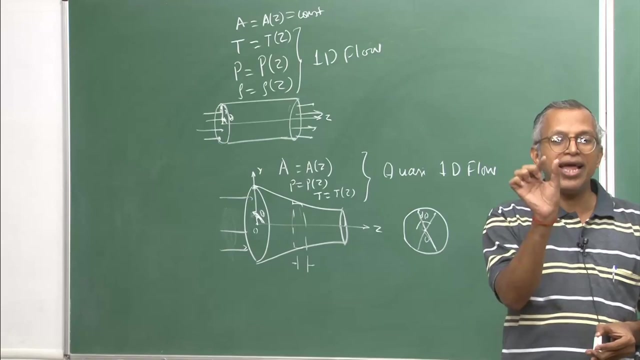 we call it as a quasi one dimensional flow. Please, this is the very important concept you must understand here. the rate at which along the z direction area is decreasing is very, very small, small, such that the property is not changing. if you take a small element like this, This: 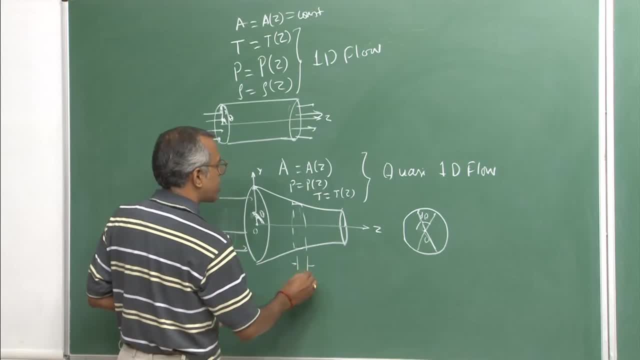 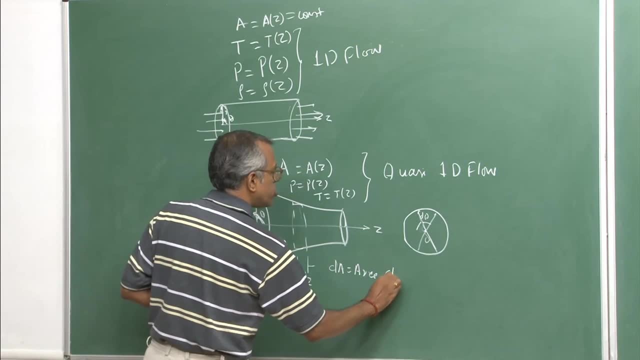 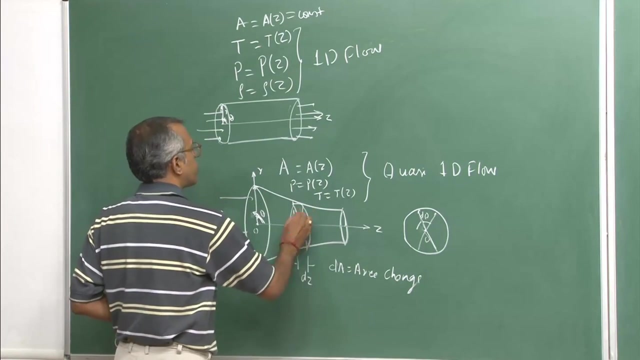 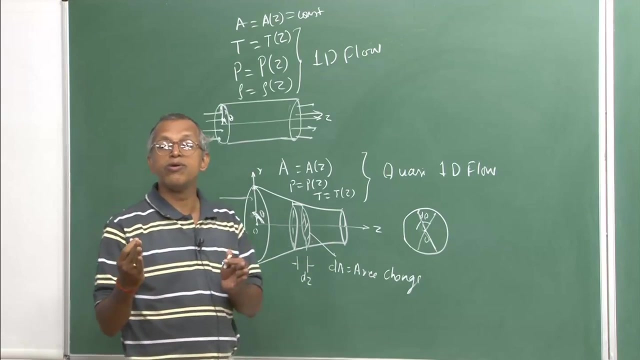 is my element. you can say d z in z direction. however, you can say in area wise, it will be d, a area change. If I take this, this will be basically like this kind of things, cross section, So this change in area. in comparison to this, it will be very, very small. So this: 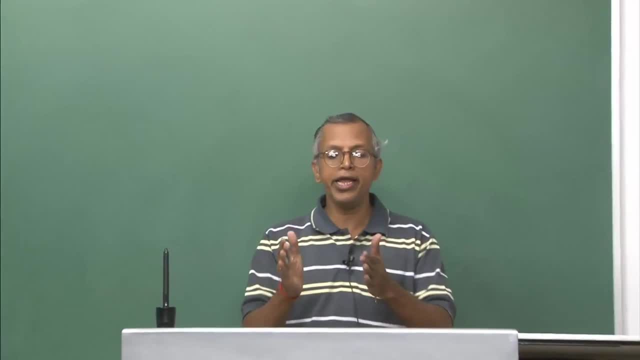 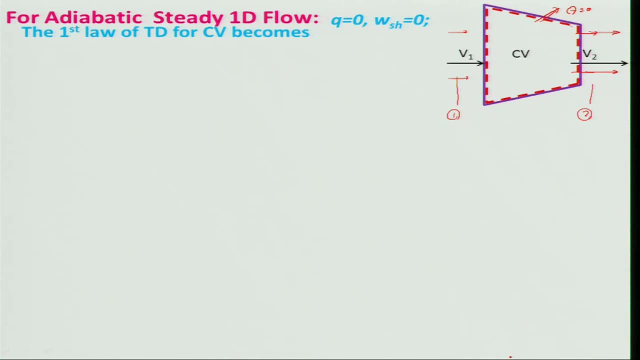 is a very important concept. you must appreciate this, and here we are doing the similar thing as well. However, it is not very obvious from the equation we will be looking at in little detail later on Here. I am considering this as a equations of first law of thermodynamics. 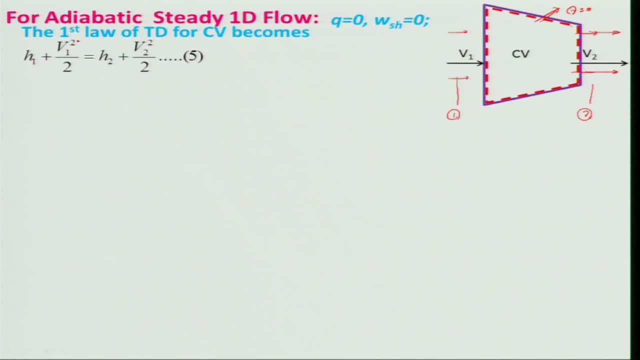 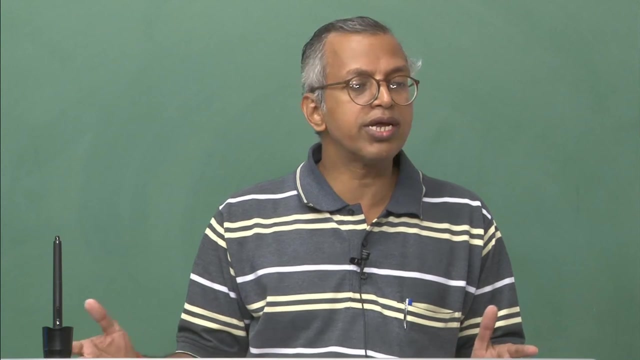 for control volume. We state that h 1 plus v 1 square divided by 2 is equal to s 2 plus v 2 square divided by 2.. Now this equation I have just written. do you agree with this? how it has come from? 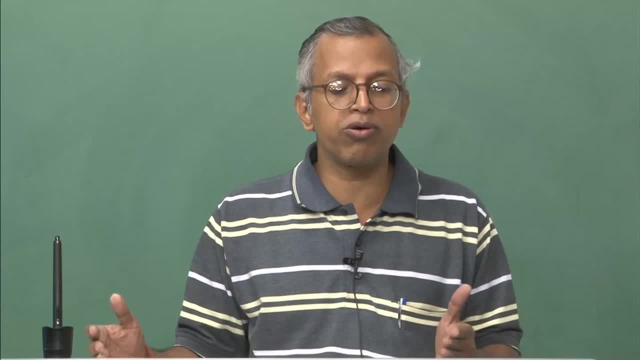 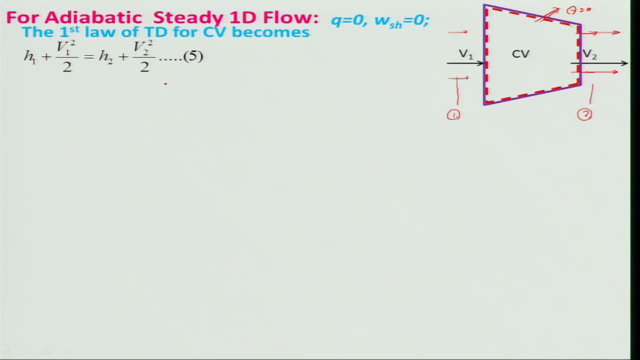 where it has come: h 1 plus v 1 square divided by 2 is equal to s 2 plus v 2 square divided by 2. from where it has come: energy equation. So if I want to write down energy equation what it would be, I must know that then I will. 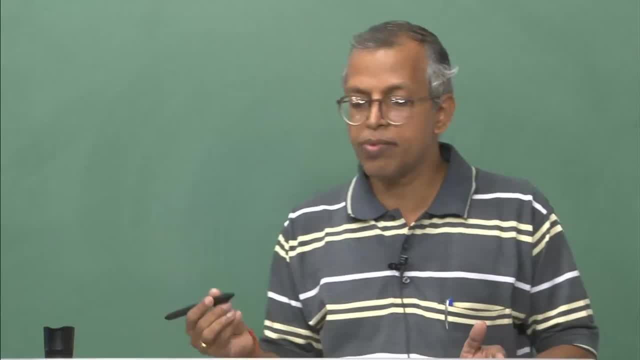 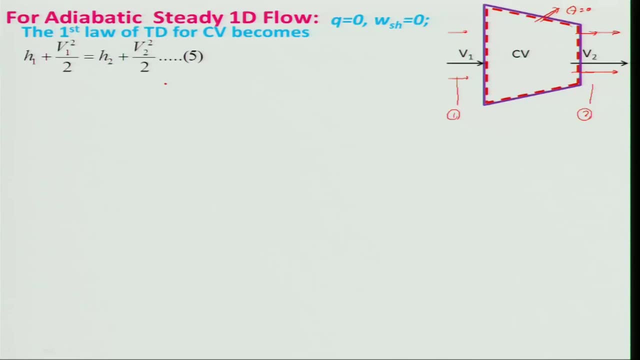 have to make this, what you call, make the assumptions whatever. that q is equal to 0, sap to work is 0, then I will have to do that and there is no gravitational, you know, or the potential energy change. I want to write down for you. let me do that. 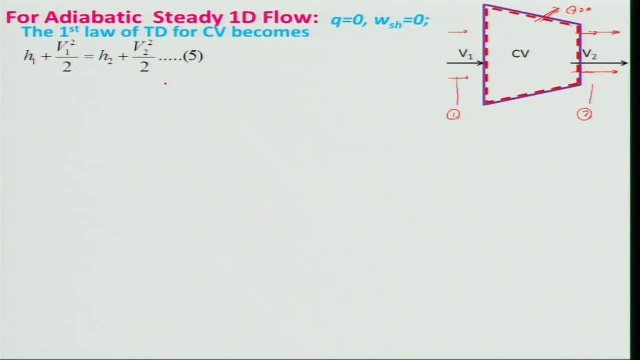 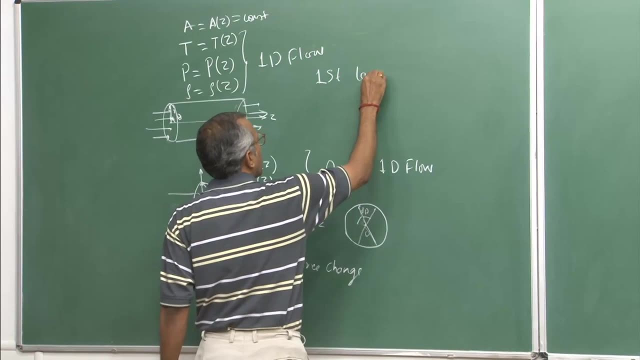 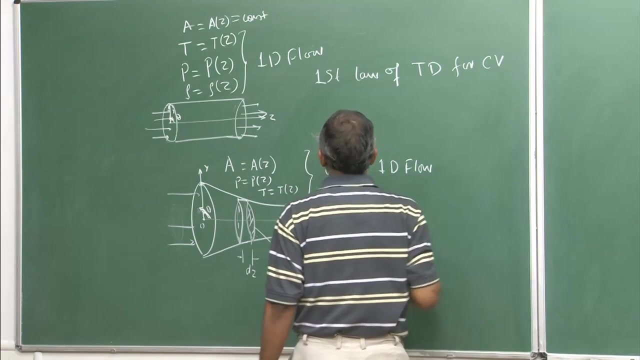 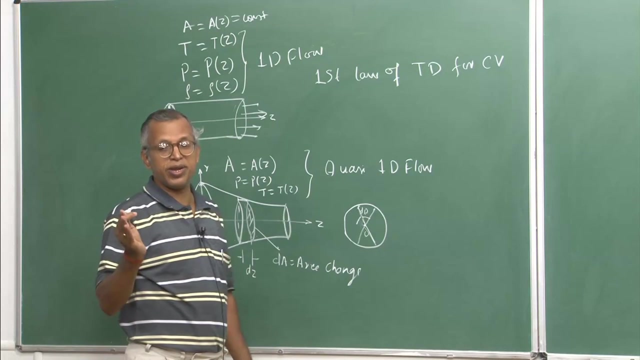 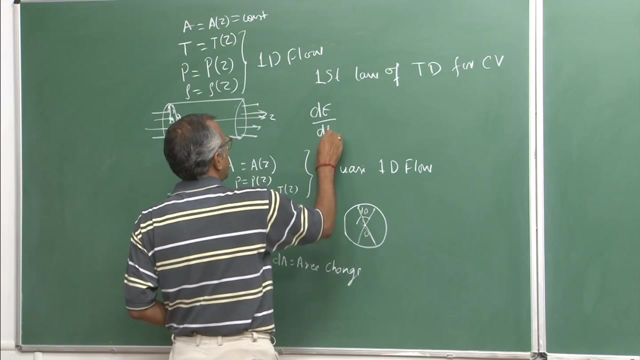 So if you look at this equation- thermodynamics for a control volume- and keep in mind that we are considering what you call one dimensional flow, that is very important. generally, you know flow is uniform. I will write down Across this, across section, what we are considering. So I can write down: d e by d. t is equal to: 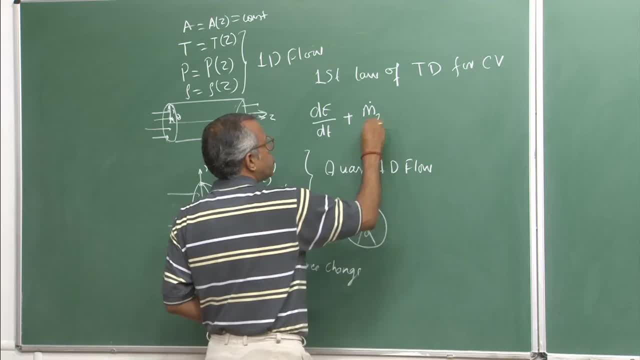 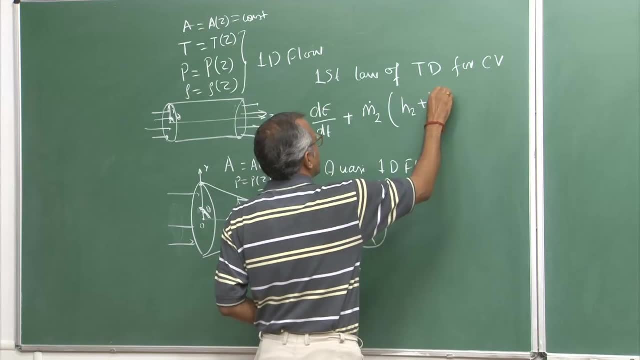 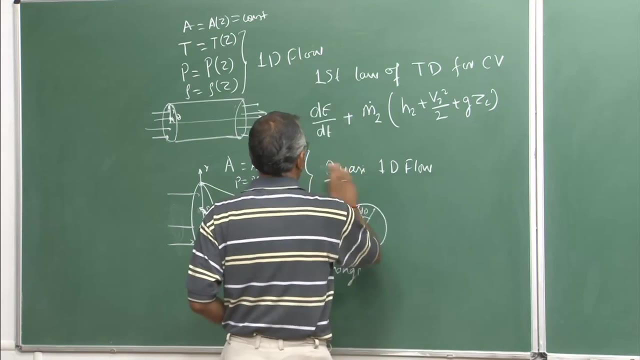 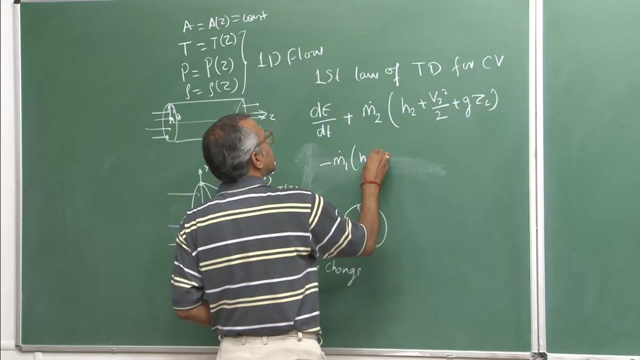 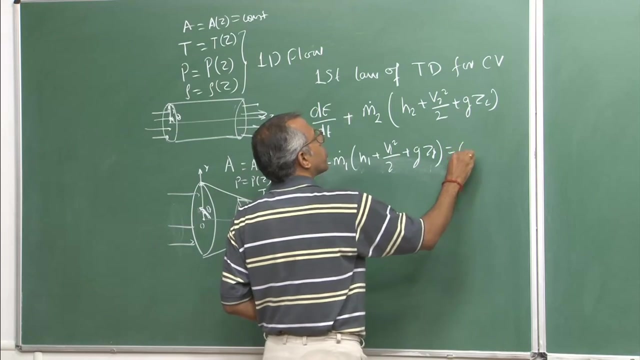 is plus m dot 2. if I take a station 1, 2 and it will be h 2 plus v 2, square, 2 plus g z 2. So this is equal to minus m 1, h 1 plus v 1. square by 2 plus g z 1 is equal to that. 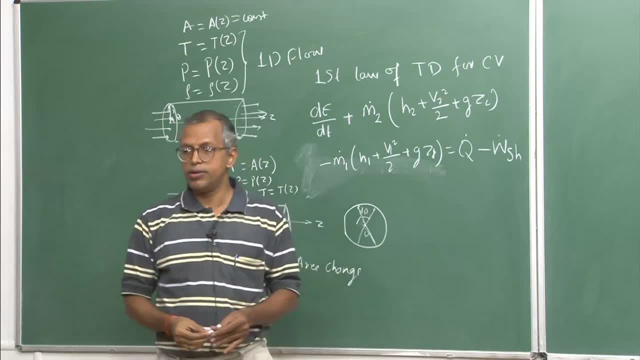 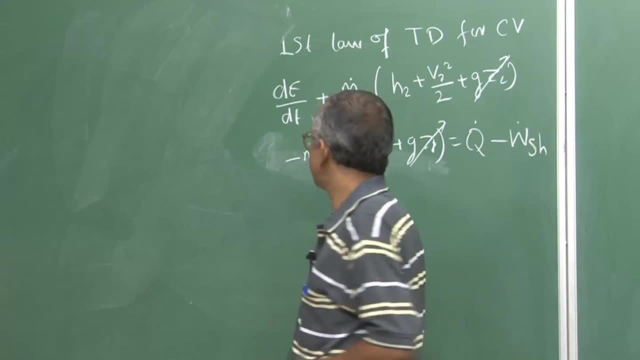 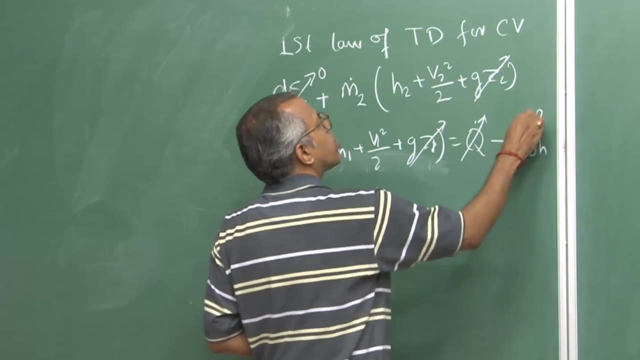 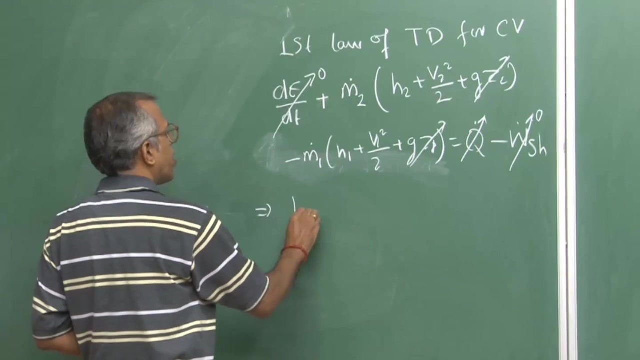 minus w sap. Now, in this case, what is happening? we are not considering this potential energy terms and this is a steady flow, Right, And there is adiabatic flow. this is sap. to work, then I will get: h 2 is plus v 2 square. 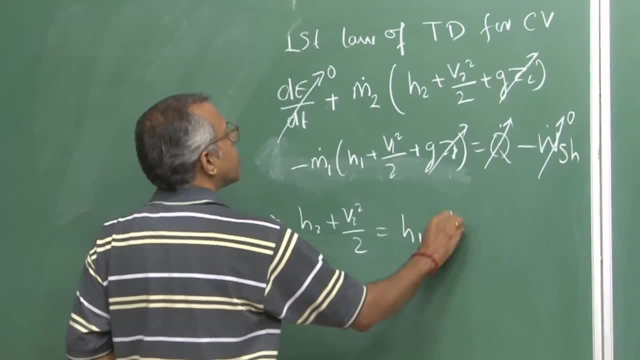 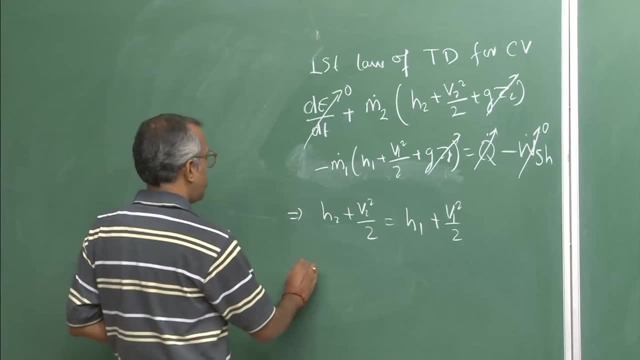 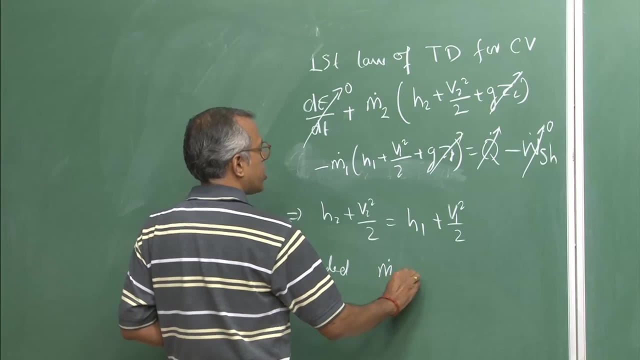 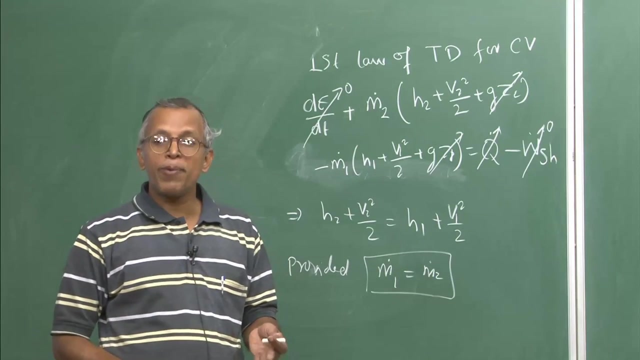 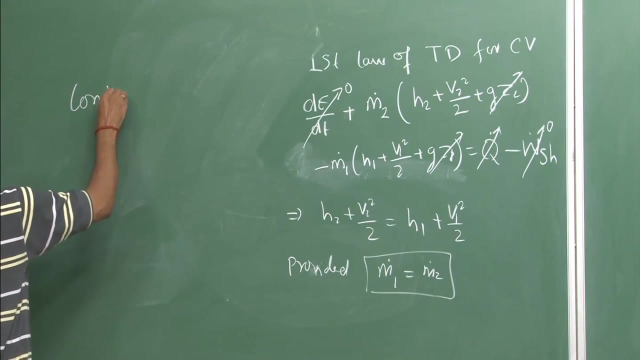 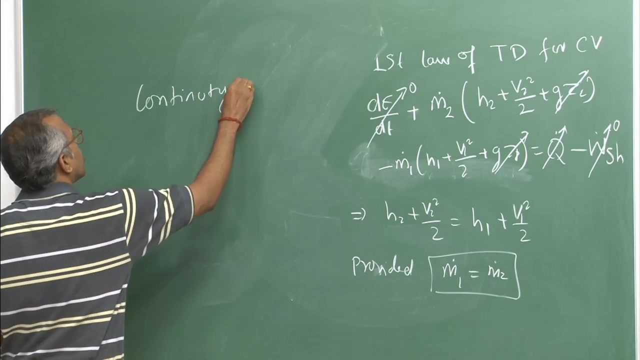 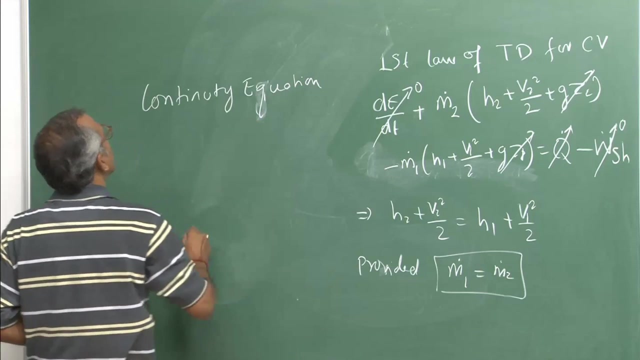 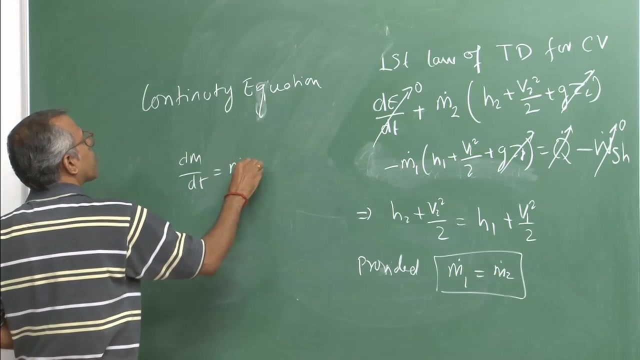 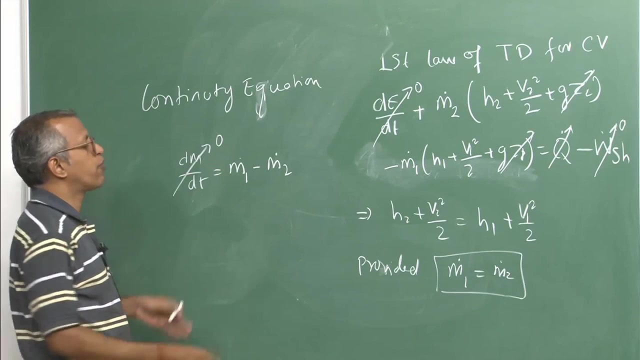 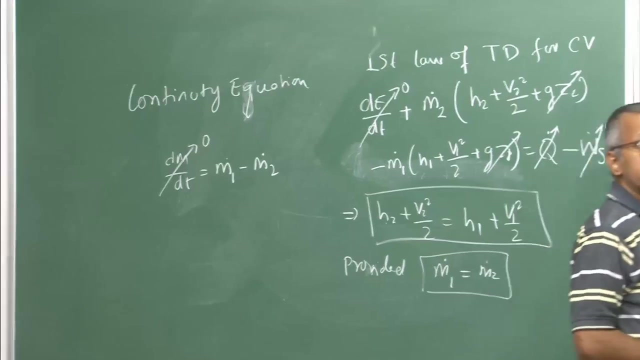 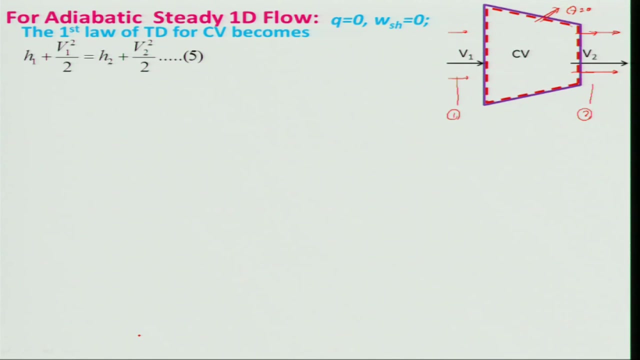 2 is equal to h 1 plus v 1 square by 2. provided what? provided you know, provided I will write down the flow under steady state condition, with, of course, no sap to work and adiabatic in nature. So if I convert this equation in terms of what you call temperature, 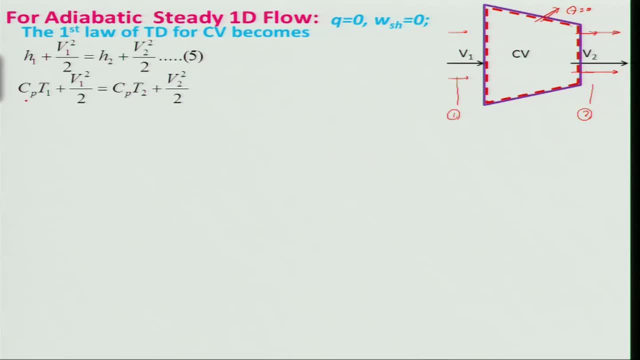 what I will do. I can write down in place of enthalpy. I can write down: c, p, t 1 plus v. 1 square divided by 2, is equal to c. p, t 2 plus v. 1, square divided by 2, is equal to c. 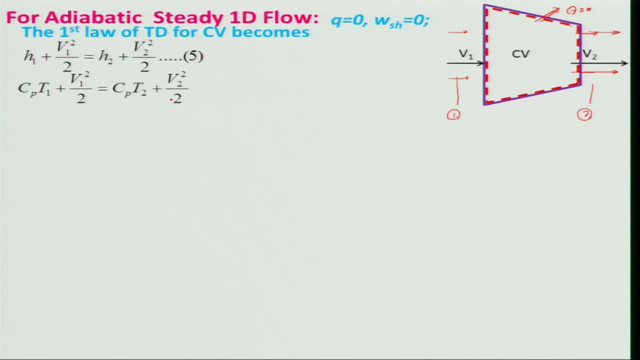 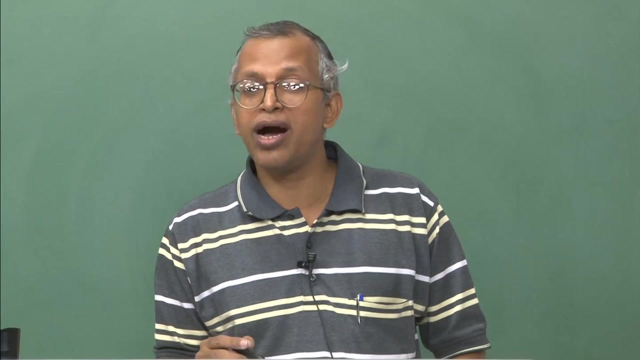 p, t 2 plus v 2, square divided by 2.. How could I write this? under what condition I can do this? can anybody tell me? we are assuming as an ideal gas right- What kind of ideal gas it is? it will be calorically perfect gas because the c? p is a function of temperature. c p is 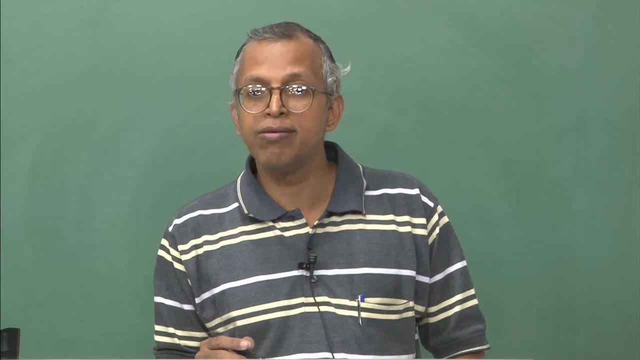 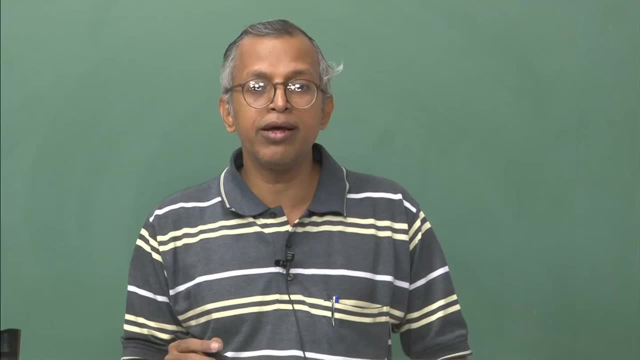 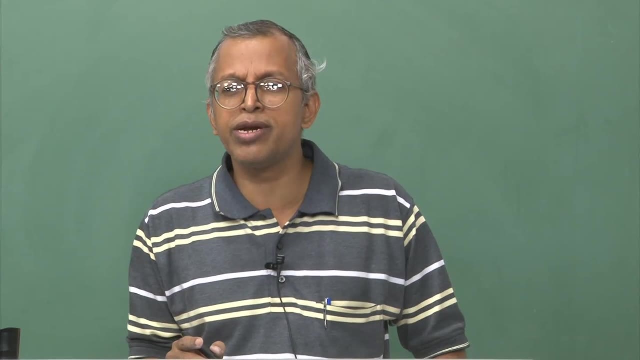 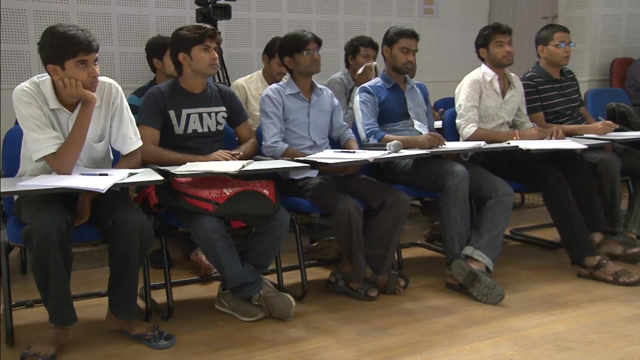 also a function of kind of fluid. If it is oxygen, it will be different. if it is helium it will be depend different, right? If it is carbon dioxide it is different. what are the difference between three examples I have given? one is monomolecule, dimolecule and trimolecular. 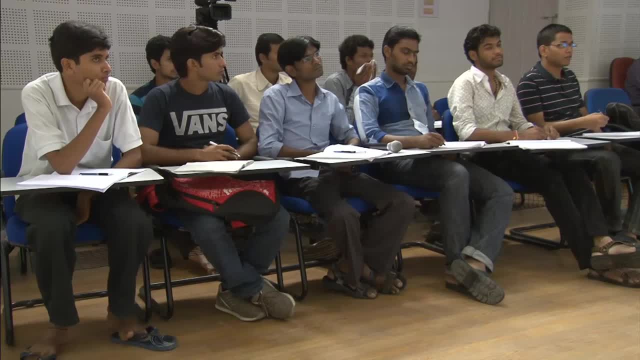 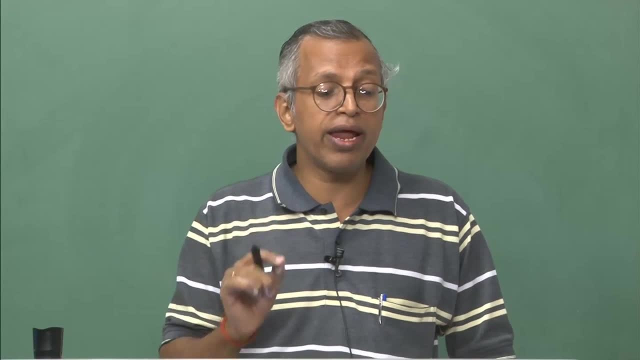 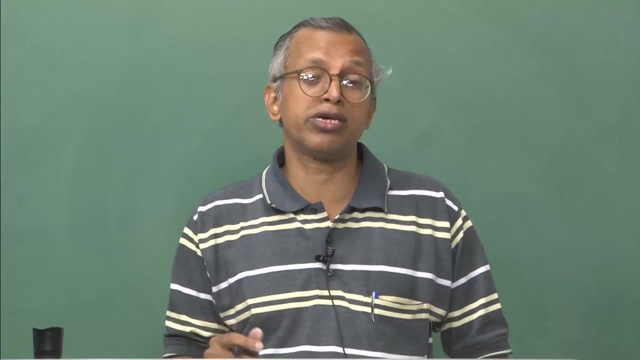 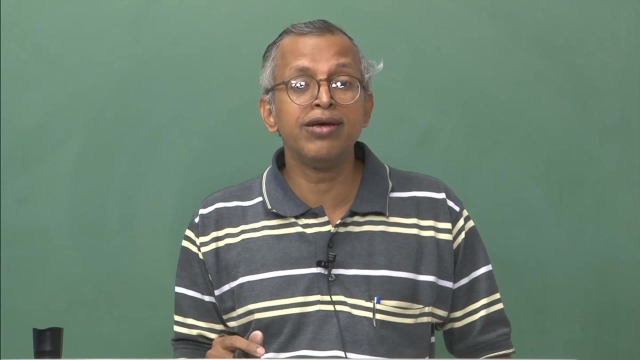 structures right, atomic Right. So therefore it c p will be different. and here we are assuming that specific heat, or the c? p, is also a function of temperature. in this case we are assuming that c? p is not changing with temperature. When it will be valid if the change in temperature is not? 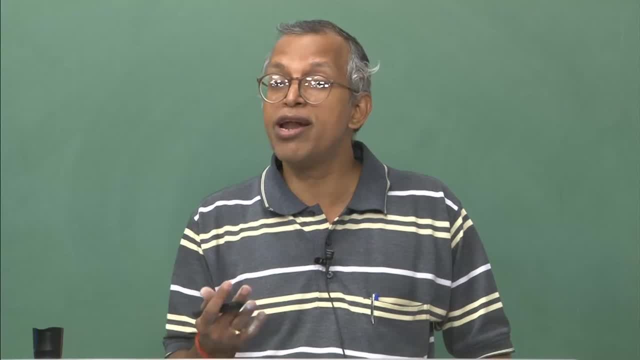 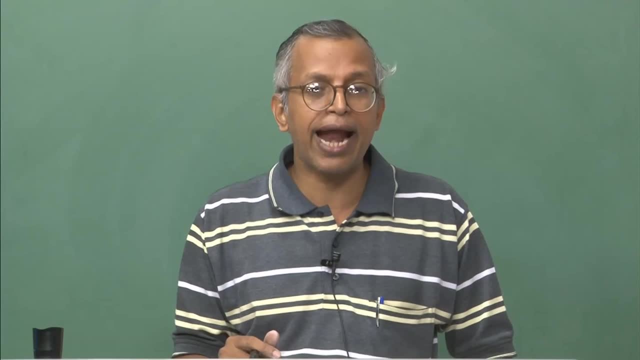 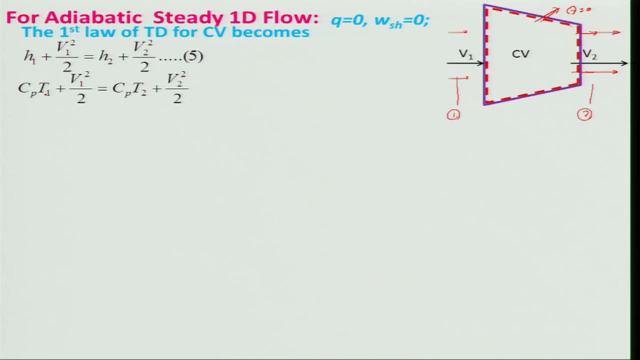 much, but in case of combustion we cannot really do effort to do that. of course we will be doing, but we are making lot of error in that right. So therefore you keep in mind that we could do this conversion for the calorifically perfect gas right Now. what we will do, we 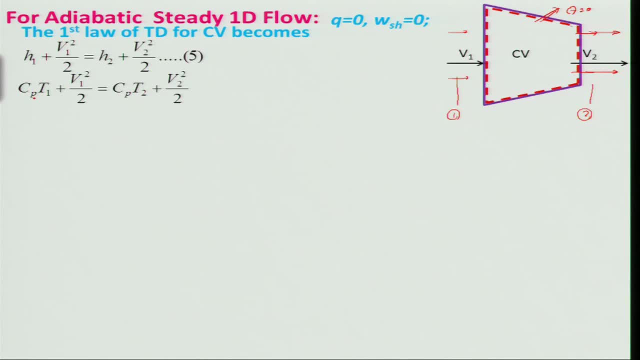 will put this in place of c p. we will express in terms of the gas constant, that is specific gas constant, that is r, what we are saying And what we will be doing in the in place of c p. you know I will be using c. p is equal. 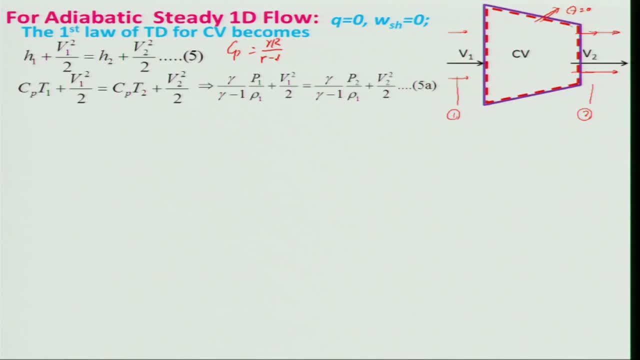 to gamma r divided by gamma minus 1, and keep in mind that ideal gas equation is equal to p, rho r t. So if I write down in place of c, p has c, gamma r, gamma minus 1. it is here And in place of r and t, And if u raise to, 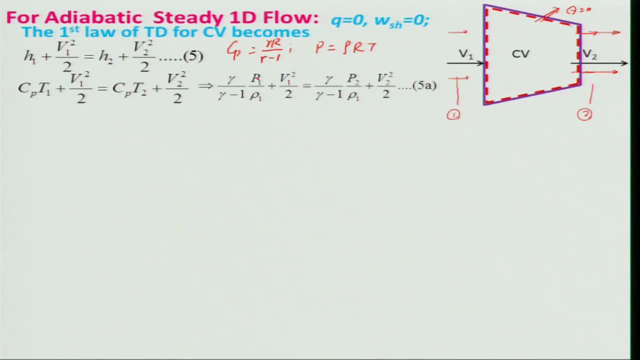 if you look at this, T 1, R, T 1, it will be P 1 divided by R 1. from this equation of, from this equation of state for an ideal gas, you can write down P 1 divided by R 1, of course. 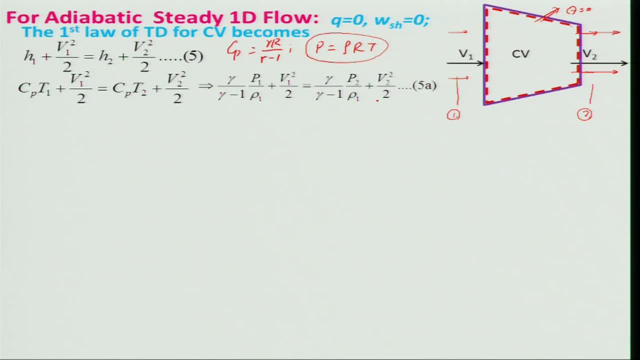 V, 1 square divided by 2 remains same and similar thing for the right hand side. Can we recognize this equation, what kind of equation it is? all of you are exposed to the fluid mechanics earlier and even what kind of equation this is. can anybody tell me what it says? it says: 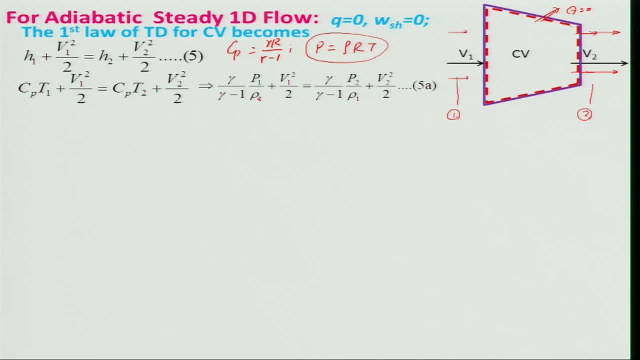 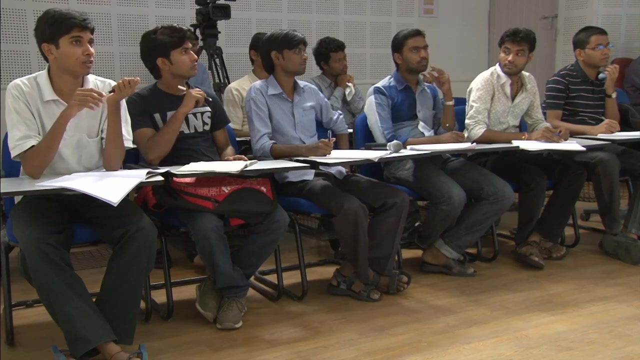 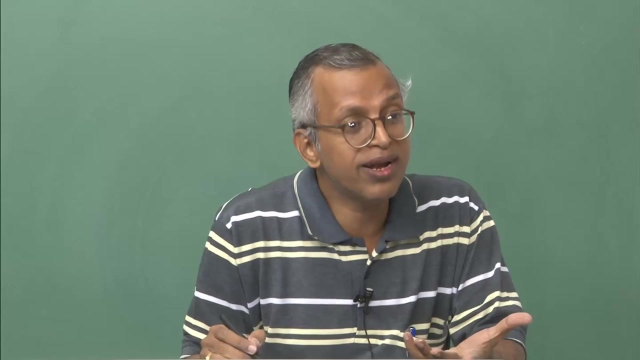 basically ratio of pressure and density. This says is the velocity particularly you can think of in terms of kinetic energy, and what is this? can you say anything about this term? I mean, I am expecting an answer: P by rho 1, P 1 by divided by rho 1. what it indicates physically, what do you mean? speed? 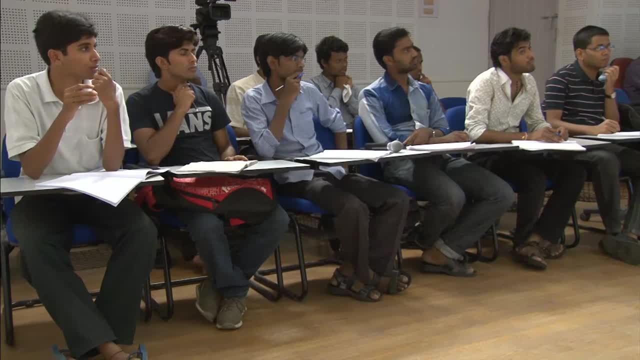 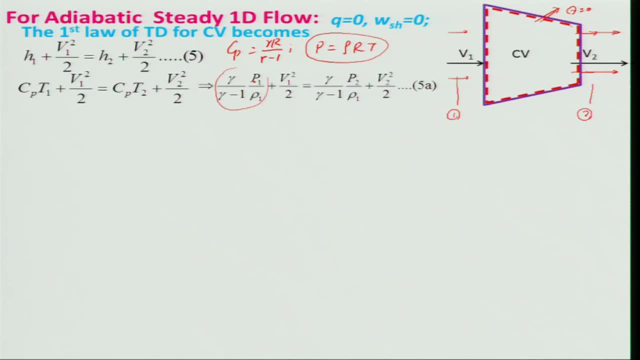 of what speed of sound, where speed of sound comes into picture here. So, if you look at, this is, of course, what he has told. it is similar to that, but, however you know, it is different. physically, If you look at, it will be linear, And if you 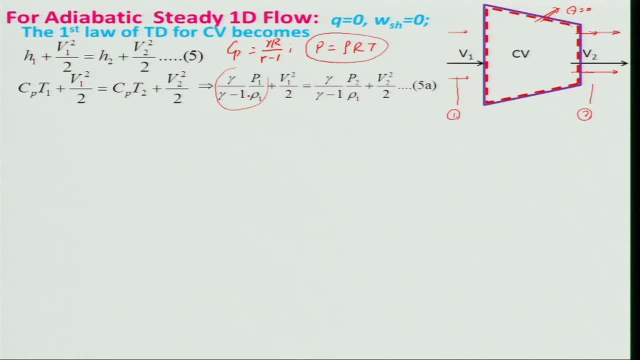 like making a flow. what will make the flow to happen? it is the pressure, if I look at in that terms. So, but this is applied basically and if you look at, can I call it as a Bernoulli's equation, and generally people call it as a Bernoulli's equation for compressible flow. 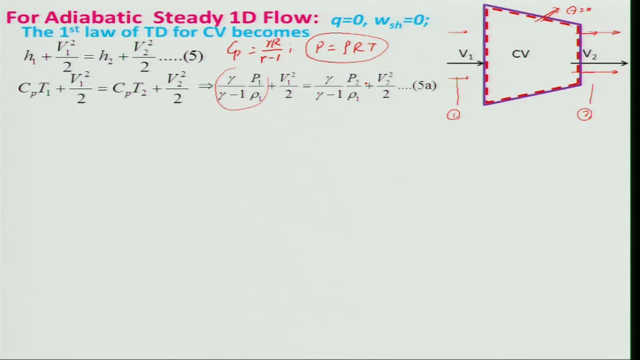 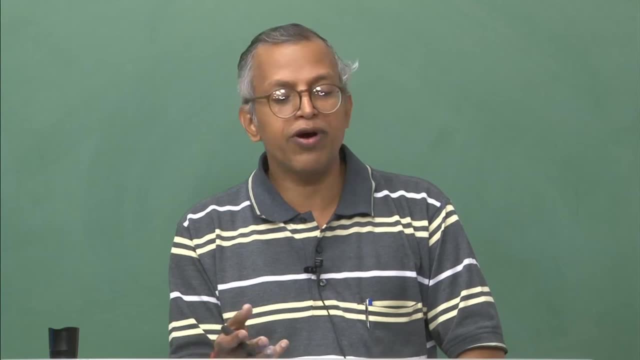 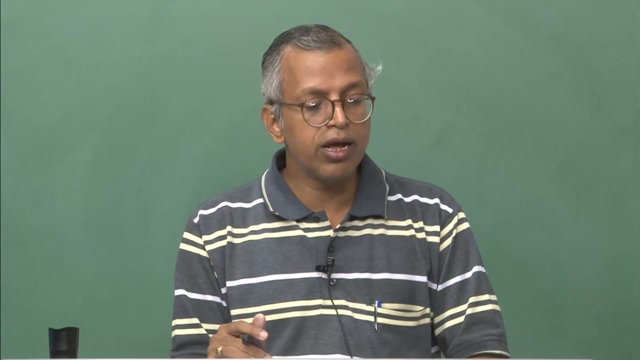 But, however, in some of people dispute they says that you know, like Bernoulli's equation would not be there for an cannot be applied for an for compressible flow. But however, it will be convenient because it is similar to that. let us see that, whether we can derive. 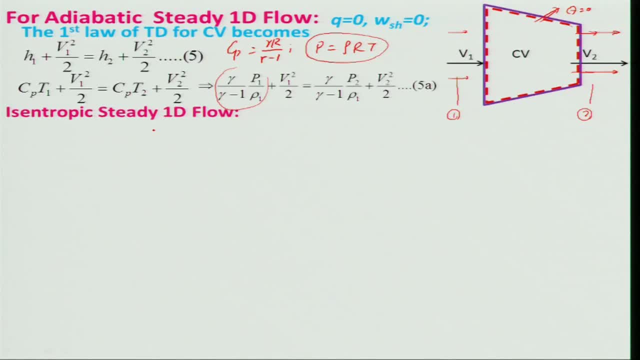 a Bernoulli's equation considering the flow to be isentropic and steady, one dimensional. When I say that isentropic, it is basically change in entropy is equal to 0.. If change in entropy is equal to 0, then what will happen to this? first Gibbs law or expression. sometimes people call it as a Gibbs expression. 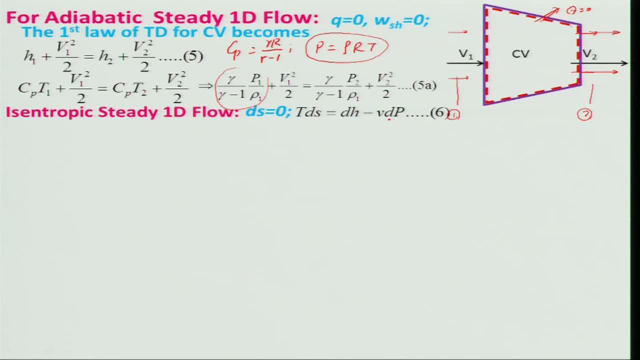 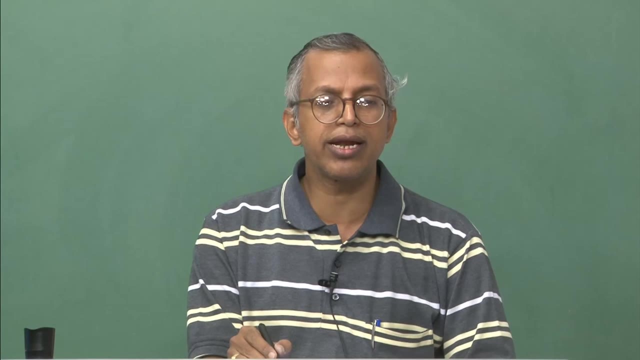 that is, T d s is equal to d h minus v d p. I think I had discussed in the last lecture this is a combination of first law of thermodynamics and second law of thermodynamics. together We will get this expression some of you might have looked at and see that how it is derive. 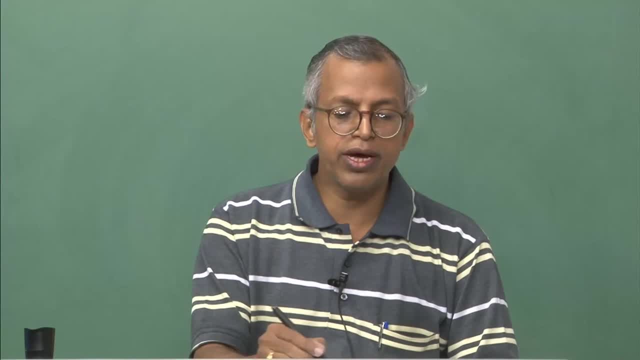 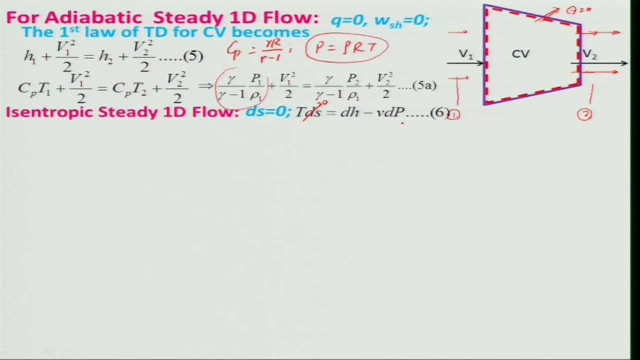 and what it is implication. So if the it is an isentropic flow, then I can make you know it is 0.. So what it indicates this expression? equation 6: it indicates that d h is equal to v d, p. 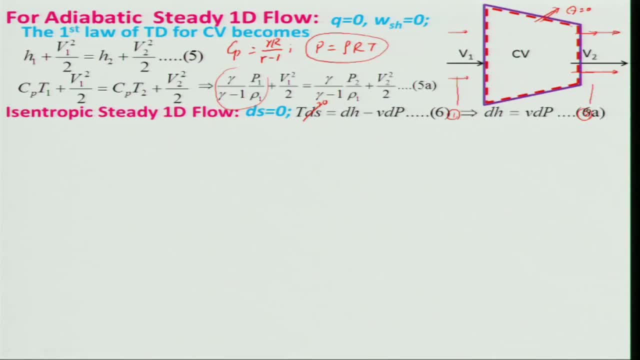 what will be done on the fluid so that it can flow? as a result, 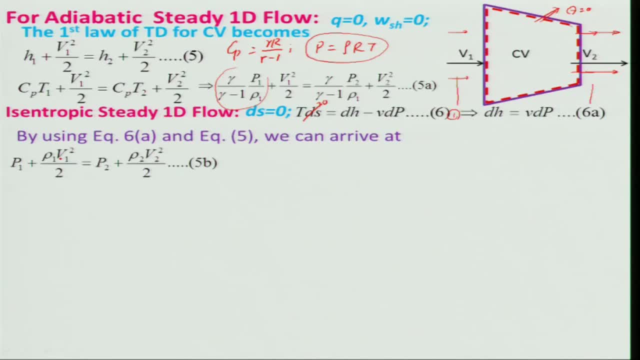 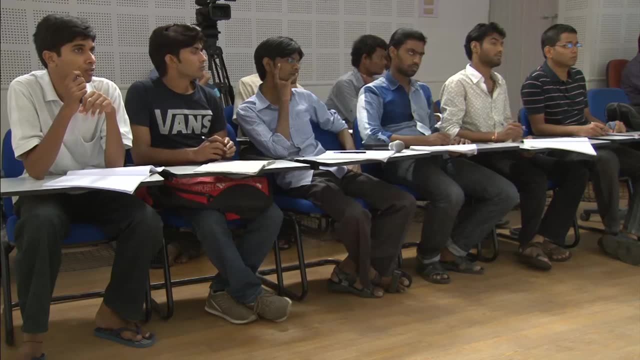 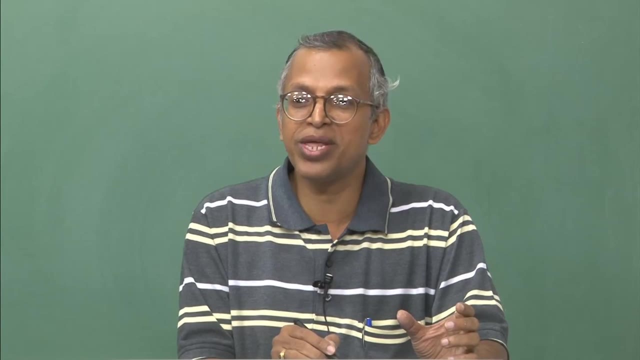 there will be kinetic energy, change in energy. that means what is saying: if pressure increases, what happens to the velocity decreases? but we know that in the pressure gradient is more, then velocity will be more. there is something contradictory, am I right? Then how will interpret? 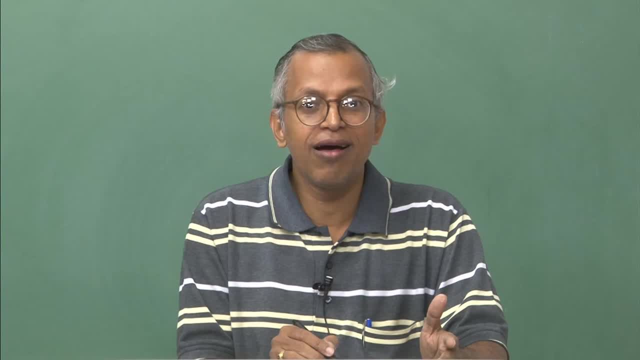 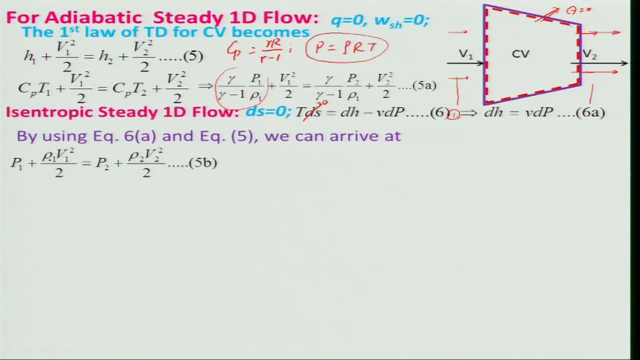 this. but from this it says: if I take station 1, p 1 I mean, and the pressure p 1, and then at the station, same place, at 1 it will be, velocity is v 1. if pressure is decreases here at the station 2, here you know what happens to velocity. velocity will be higher because 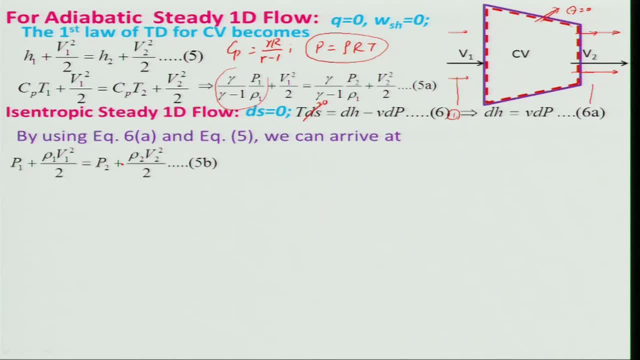 the total is remaining constant. that means total energy is remaining constant at between the station 1, between the station 1 and station 2, am I right? Of course there is another term which is there due to the elevation kind of things, which we have not consider what we call it as a potential energy. that means what it indicates. 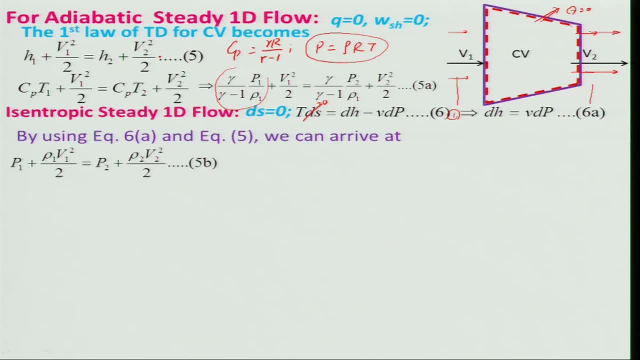 that the energy equation, that is, the equation 5, is same as that of the equation 5 b, which comes from what momentum equation, right You can derive that, and this is valid for what? steady, incompressible equation 5 b, and then isentropic flow, and whether in rotational 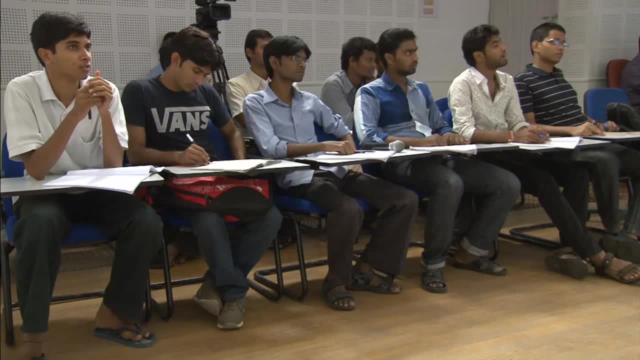 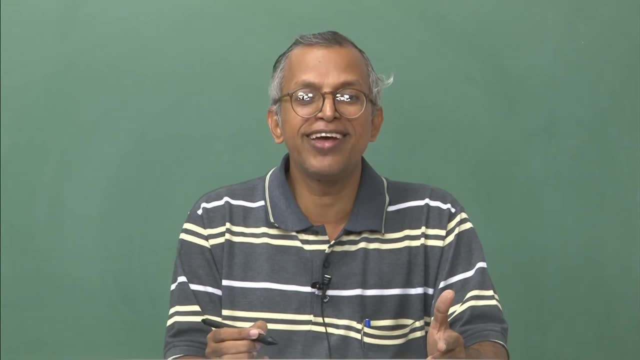 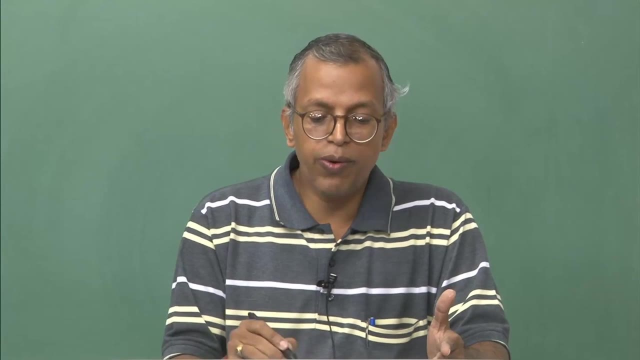 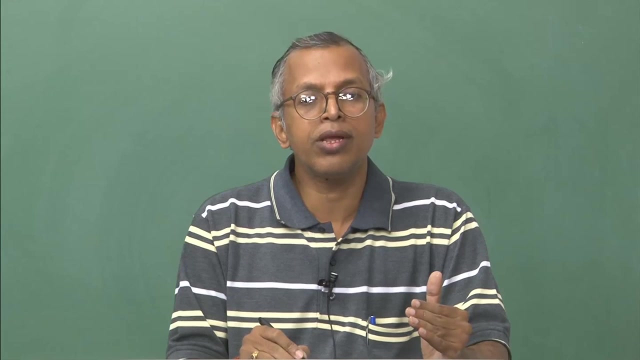 why I did not talk about it? because if it is rotational, then entropy, you know, has to be changing, particularly when near the boundary layer, you know So, and also it will be dissipated, kind of things. So therefore it is valid for one dimensional, steady, irrotational flow. 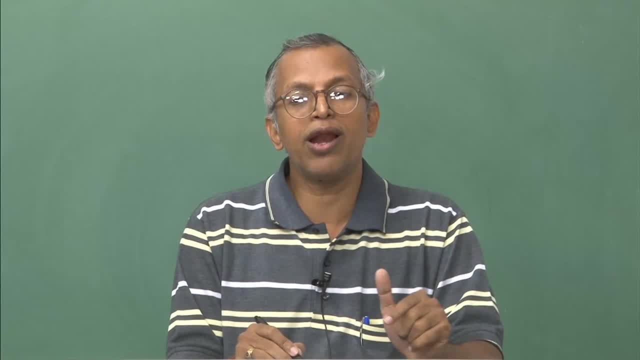 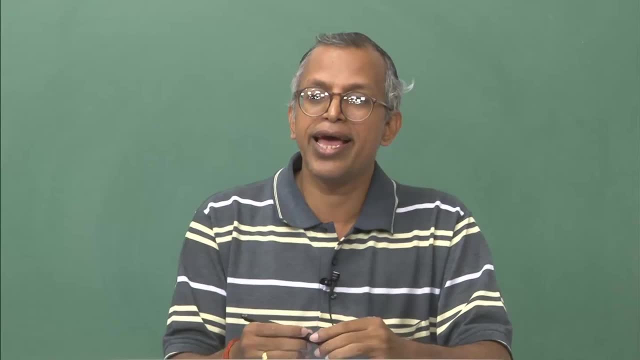 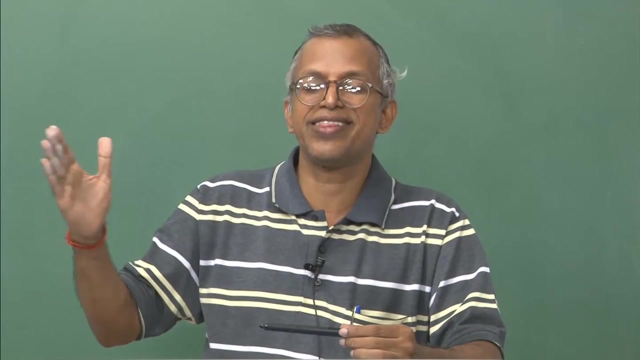 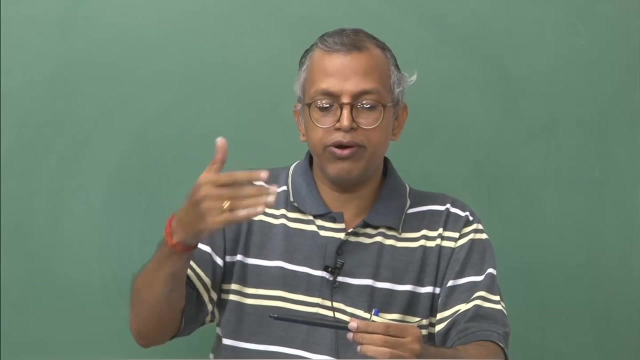 and therefore we call it, you know, flow along a streamline right where mass will be remaining constant. that means you will take a stream tube that mass at any section is remaining constant. therefore continuity is valid. So therefore, you know like one has to consider. 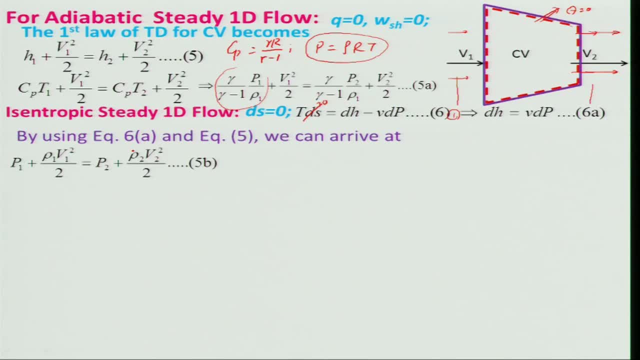 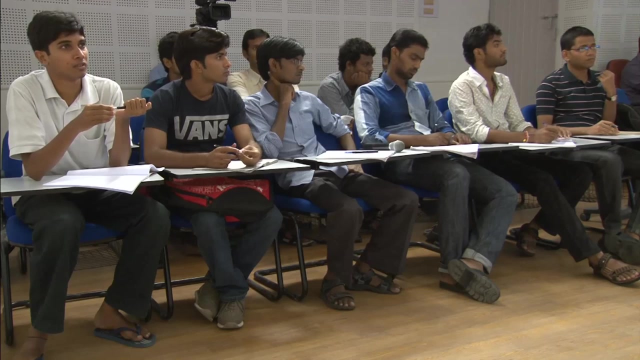 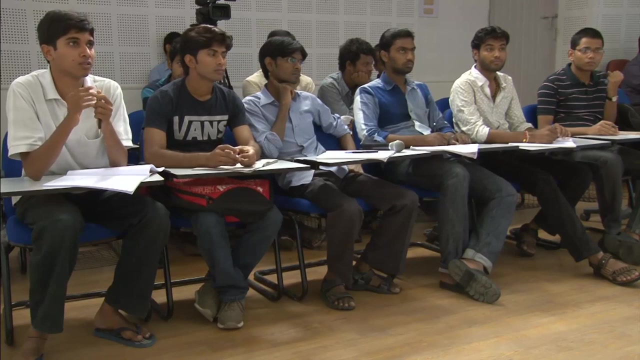 that along a streamline, it will be valid. So, and I have already told you that rho v square is a dynamic pressure and p is a static pressure, right? what do you mean by static pressure? can anybody tell me what do you mean by static pressure? is there? in fine, go ahead, Brought to the rest. right, how I will get it. 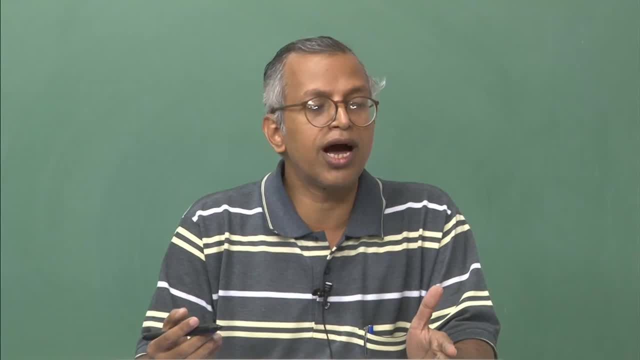 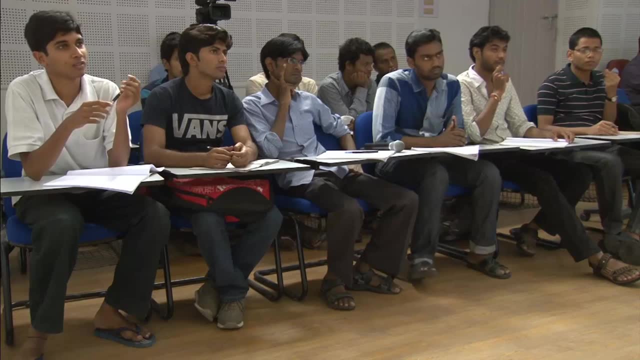 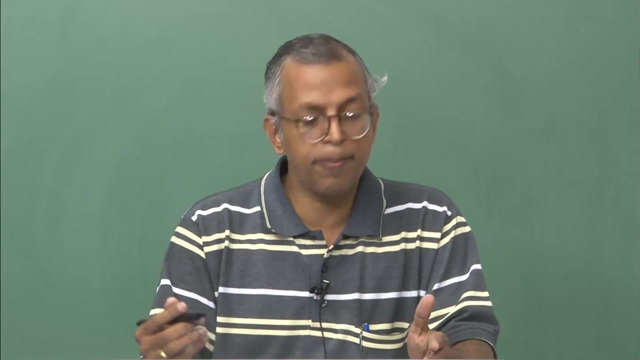 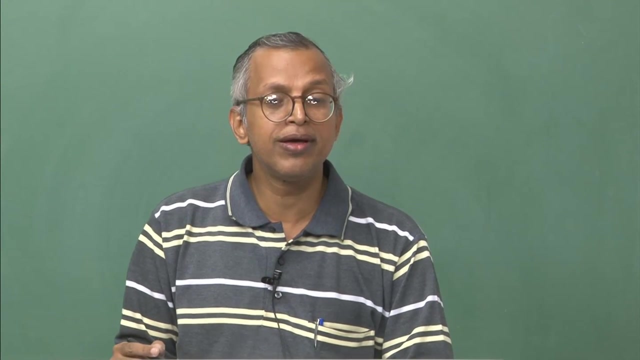 if I say that I want to measure, how can I measure it? is it I will make the fluid to come to the rest isentropically? is it possible? I can do that? that means what it is. can you people think about you? imagine that you are hoping over a fluid. So you are hoping over. 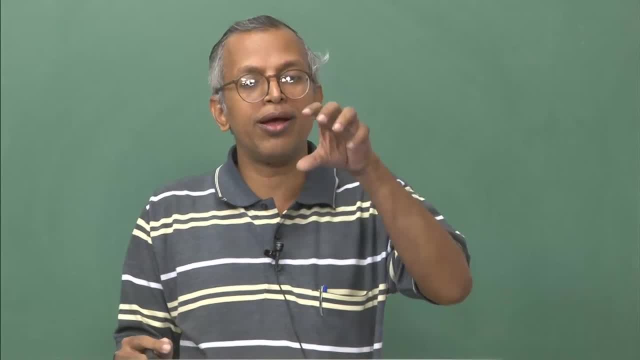 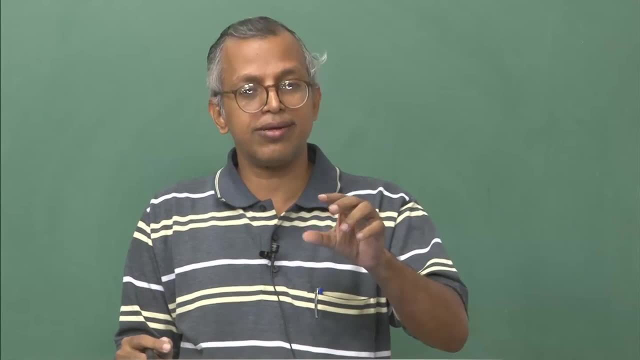 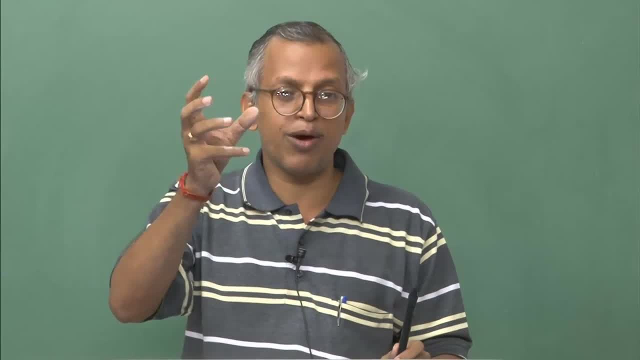 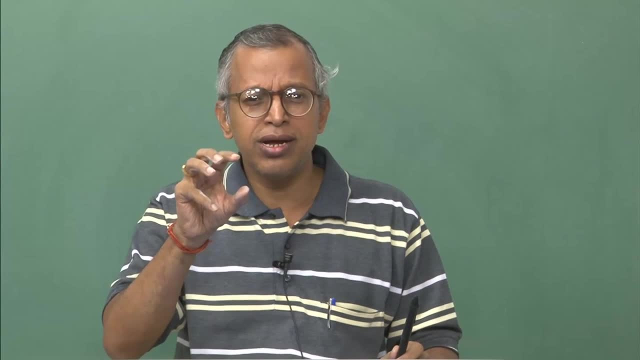 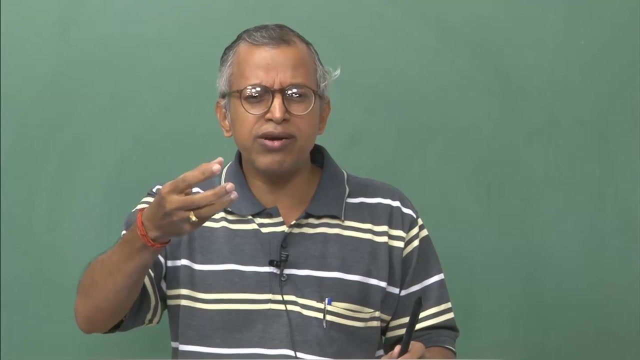 if there is a fluid element- and I am having a tiny center, Of course it is quite difficult imagine that- and then it will be experiencing certain pressure due to what, as it is moving right, A element will be having certain velocity, velocity as it moves different places, it may be experiencing different velocity, that is. 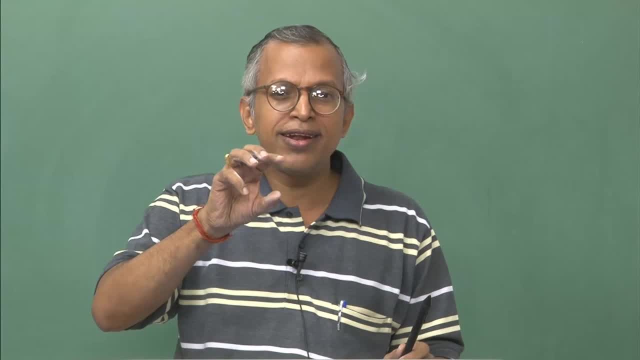 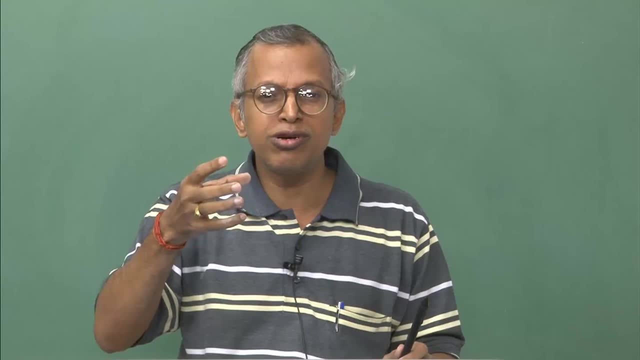 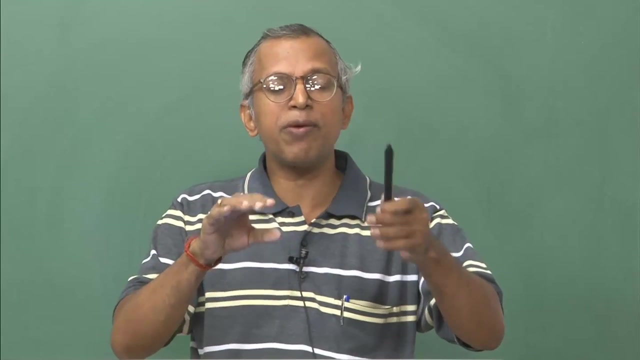 a different thing. but then what it will be experiencing? it will be experiencing a pressure or a force. The force is due to the molecular interaction. that means molecules will be coming and bombarding each other. that means that pressure which will be felt due to the change. 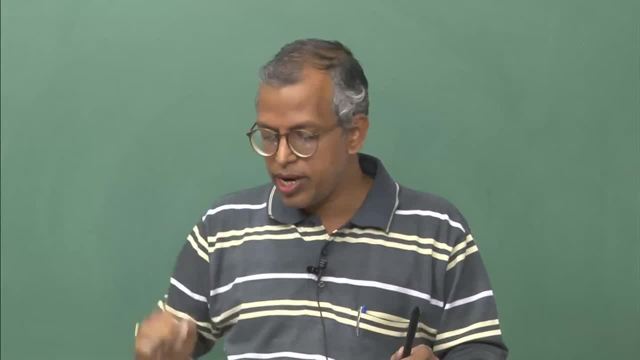 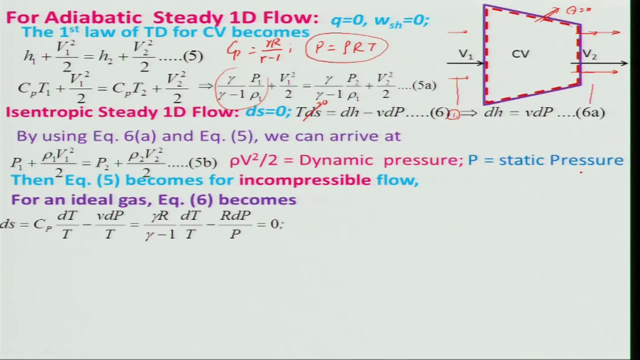 in the what you call momentum change that you will get the pressure. we call it a static pressure. So for an ideal gas equation 6 becomes. you know I can write down: d, s, will, c, p, d t by t minus v d. p by t is equal to gamma r divided by gamma minus 1 d t by t. 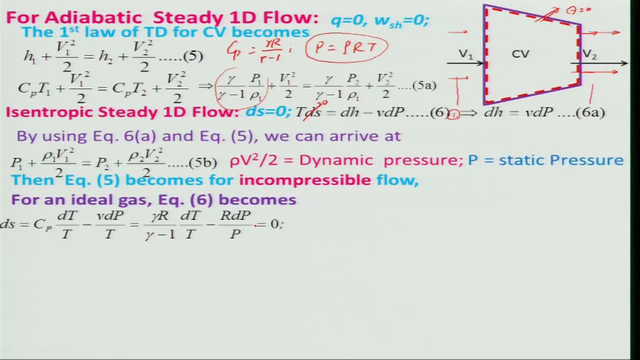 and minus r d p by p is equal to 0.. Are you getting this, this what we are getting? we are. So, basically, equation 6: I am taking and looking, applying this, you know, changing this c p values and putting this equation of state, and we are getting: p is equal to rho r t, if I apply. 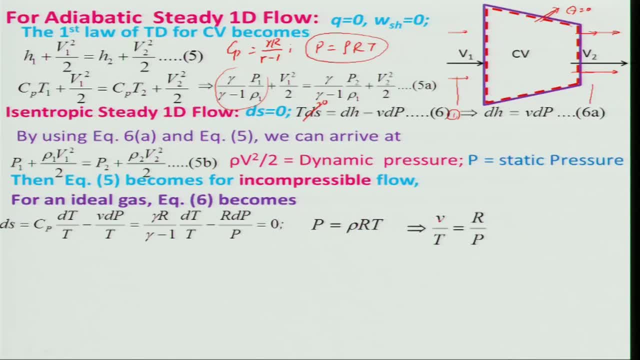 this ideal gas law, then I can get into v by t, r by p, And then if I say gamma is basically ratio of c p by c v, then I will get this expression p 2.. By p 1 is equal to by t 1 gamma, gamma minus 1. keep in mind that this is not visible, but